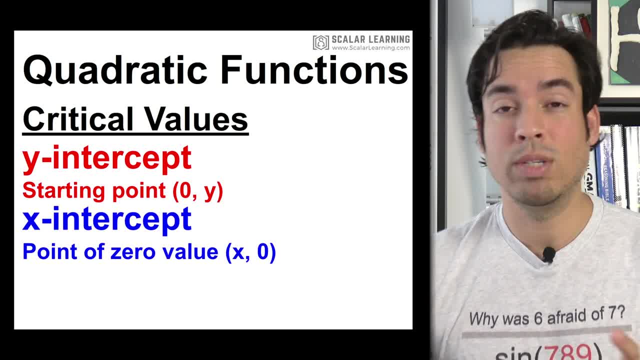 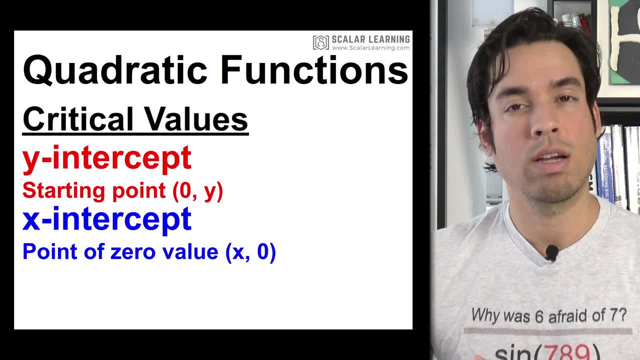 intercept. okay, and that's the point of zero value. again, if we take that analogy of the ball, it's: when does it hit the ground? when does it drop to a height of zero? alternatively, if we're talking about profit and maximizing that profit, there will be a point where the profit level will come down to zero and you'll 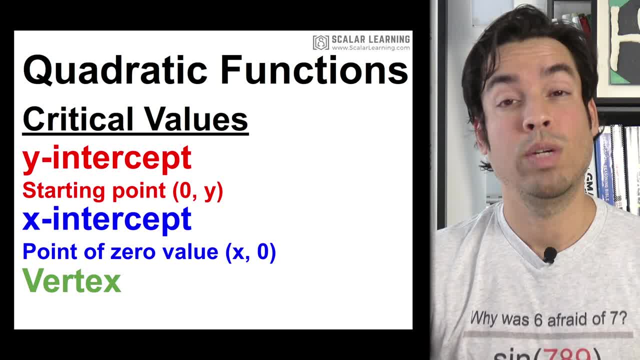 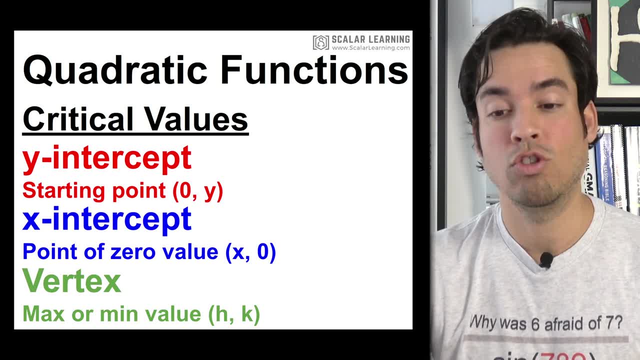 be making no money again. that's the X intercept. finally, we come to the value of the vertex, and for the vertex, this is either going to be the maximum or minimum value, and it's usually denoted by H comma K. now, when we saw that first example where it opens up, there's going to be a bottom point and this vertex 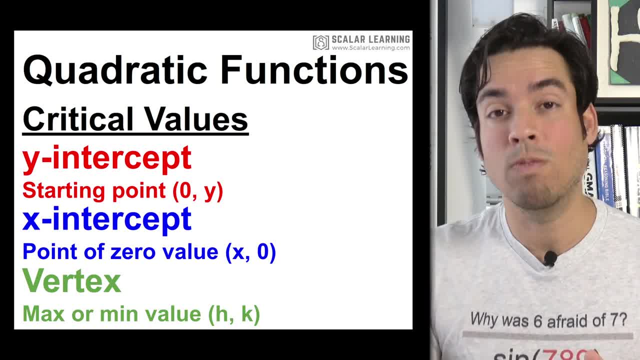 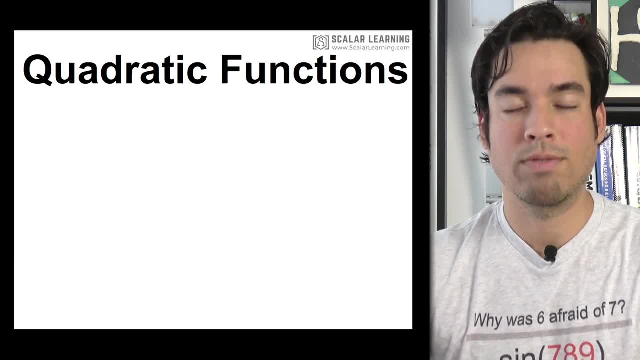 will be that minimum value and, conversely, when it opens down, you see it looks like the top of a mountain and then the vertex will be the max point. now we want to talk about the format of quadratic functions when they're written out and it's going to. 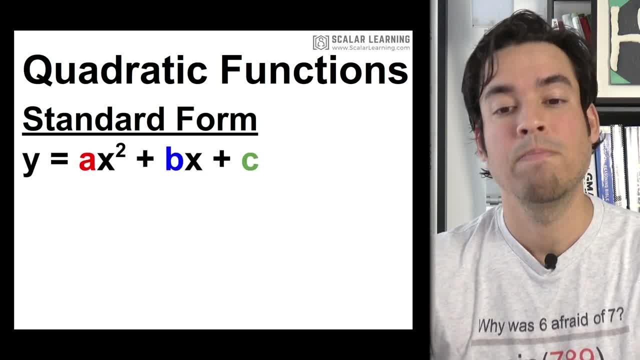 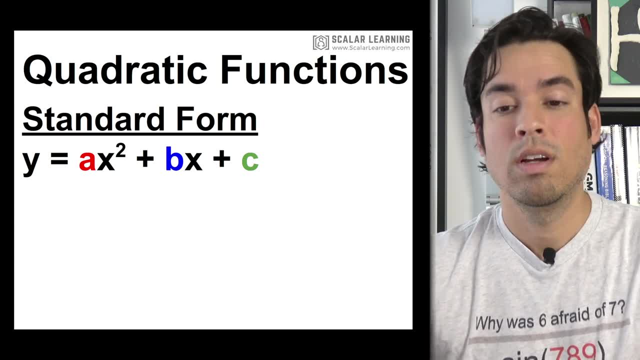 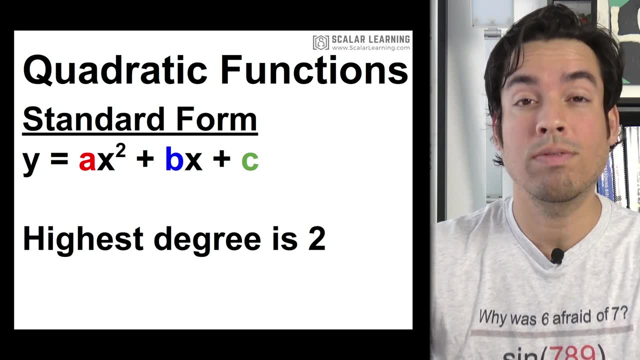 we're gonna start with standard form. so standard form looks like this: it's: y equals a, x squared plus B, X plus C. again, a, B and C are just constant coefficients. they can be positive or negative and they don't have to be whole numbers. the highest degree, meaning the highest exponent, is 2. that's what defines a. 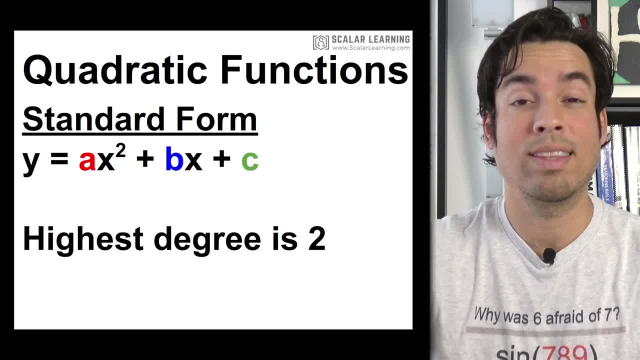 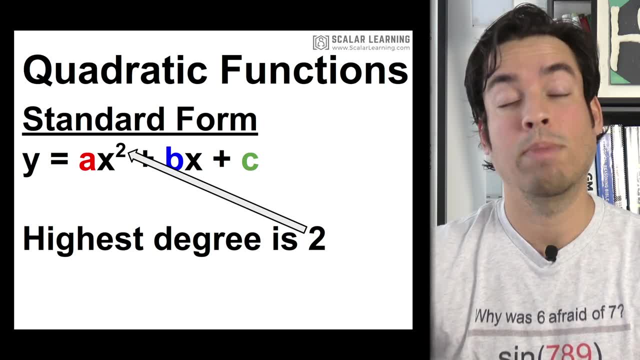 quadratic function. you can't have it to the third power, the fourth power or anything like that. the highest degree has to be 2 and you can see there's that 2 right up there on the, you know, connected with the a term. by the way, the a term is always. 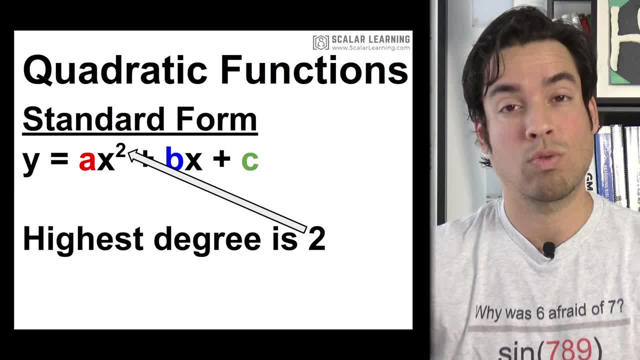 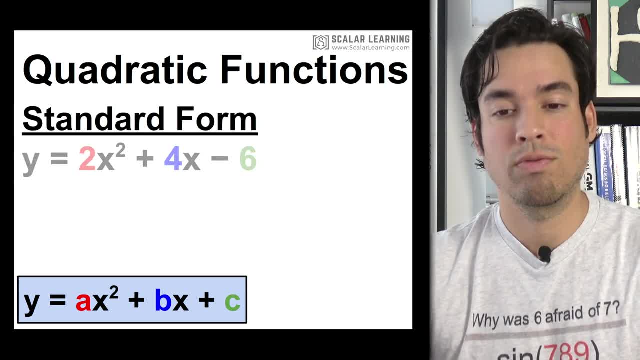 determined by whatever constant, is multiplying the x squared. now again, sticking with the fact that we recognize that there's our standard form at the bottom, I'm going to give you an example of one in standard form, and it's right here: 2x squared plus 4x minus 6, so this is a quadratic function with actual 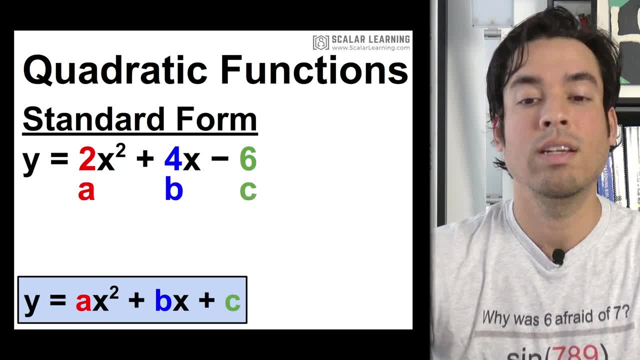 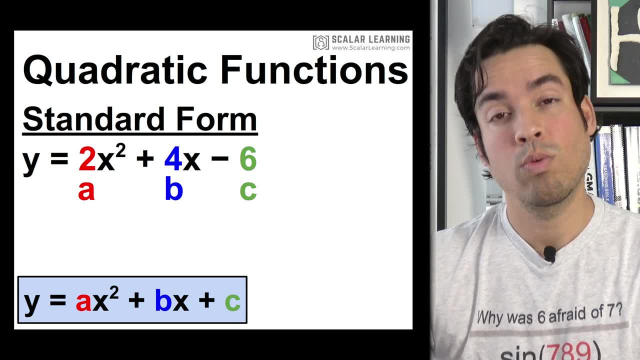 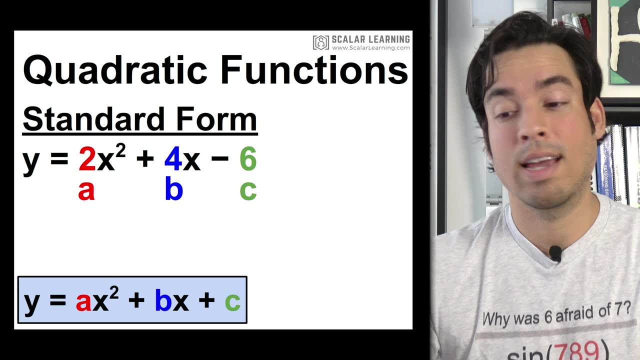 constant values in standard form. notice very interestingly: right the two values, the a, the four values, the B and the six. but it's not just six is actually a negative six. we always want to be conscious of the fact that a minus sign is sticky and it sticks to that number to the right and it actually tags it as: 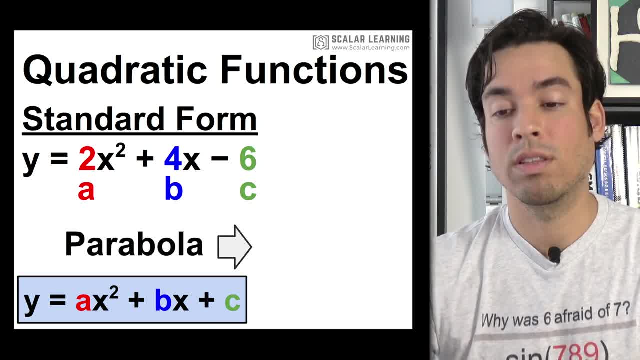 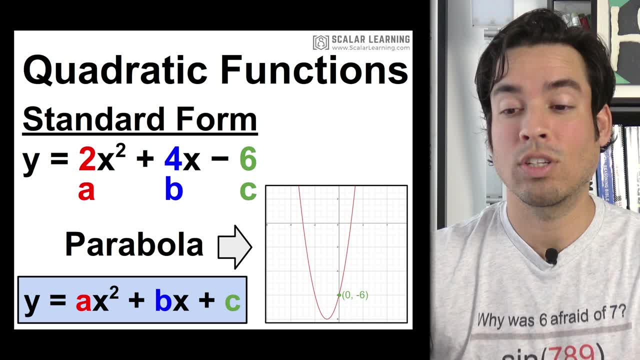 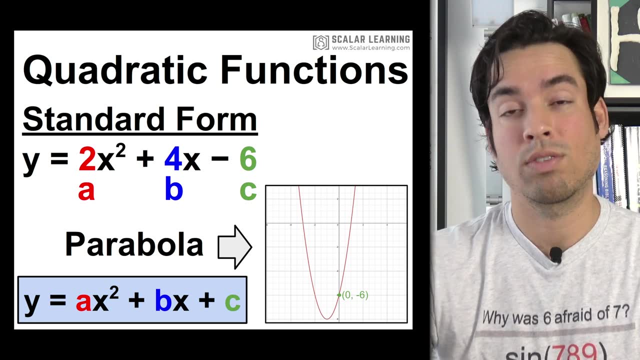 a negative number and if we now look at the parabola and the graph of this, we can see that. where is that negative six show up? it's very interesting because that negative six is actually the y-intercept. and it makes sense because if I zeroed out X, meaning if I plugged in zero for X, I would get negative six. 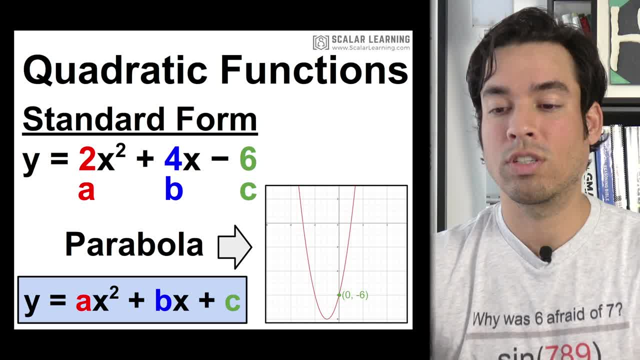 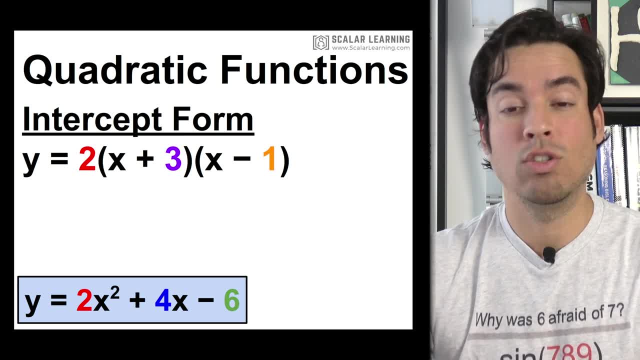 for the function value. so there you see it on the graph y-intercept, and then the of 0 negative 6.. Now again, moving forward with this same function. we're going to put this exact function into what's called intercept form. Intercept form is also where it's simply factored. 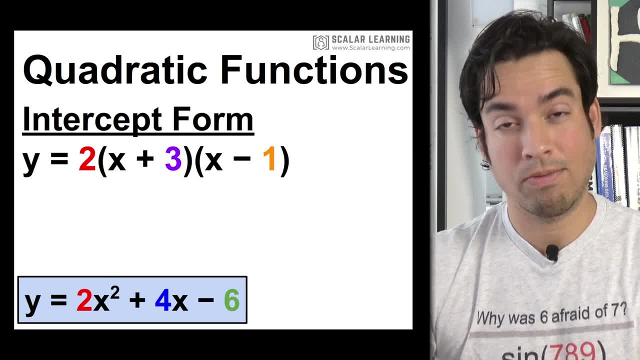 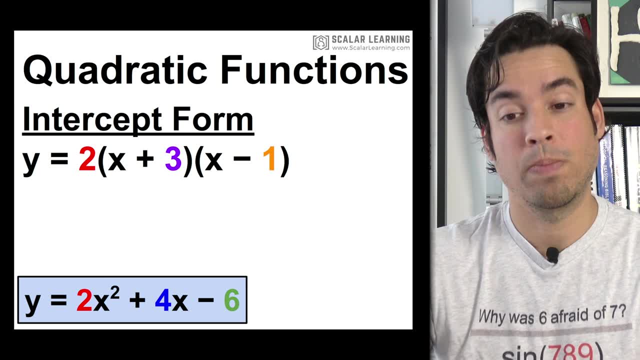 we're going to talk about factoring in a second, but what's interesting about intercept form is that the constants that are there show us what are the x intercepts and notice there's two. okay, there can be one and there can be none, but in this case there are two and it's that purple and that. 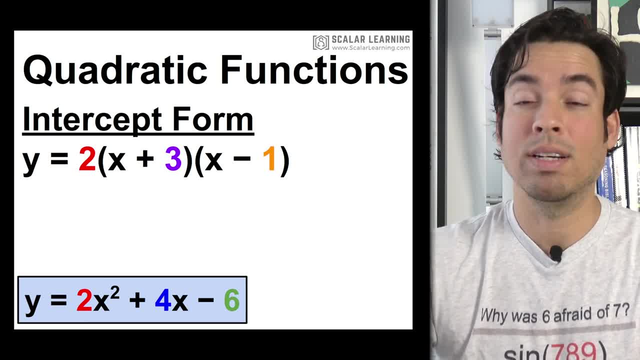 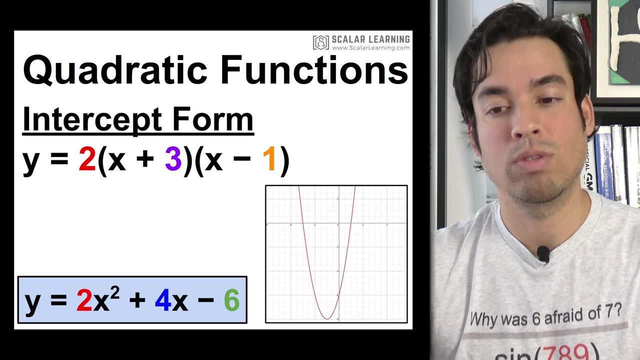 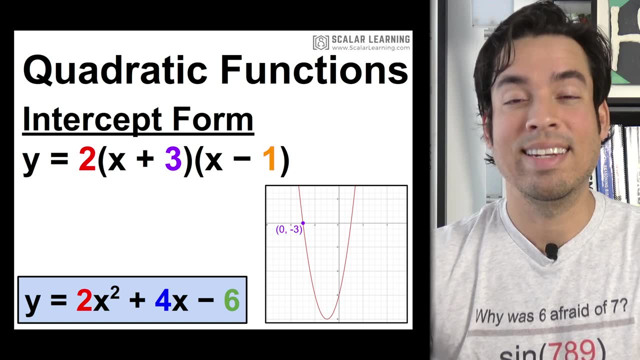 orange number, that 3 and that negative 1. but it's also important to note that when we have, when we see those values, it doesn't mean that there is an x intercept at x equals 3 and x equals negative 1. in fact it's flipped. so you'll see we have a x intercept at negative 3, and that's really. 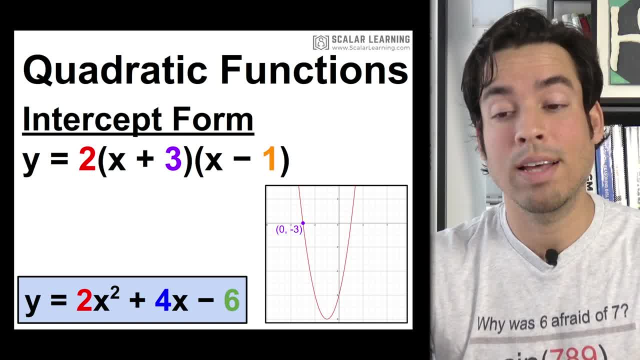 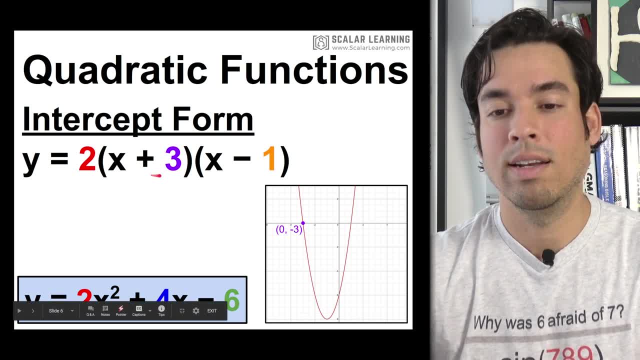 important too because, remember, the x intercepts are where the function value is 0, meaning we're trying to find a value of x that zeros out the whole function. So if I plug in a negative three into this binomial, it's gonna be negative three plus three, which is zero. 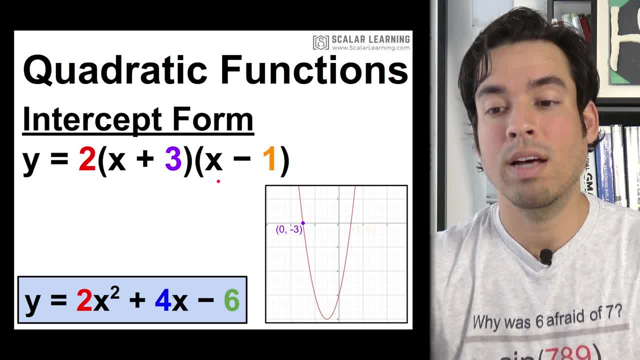 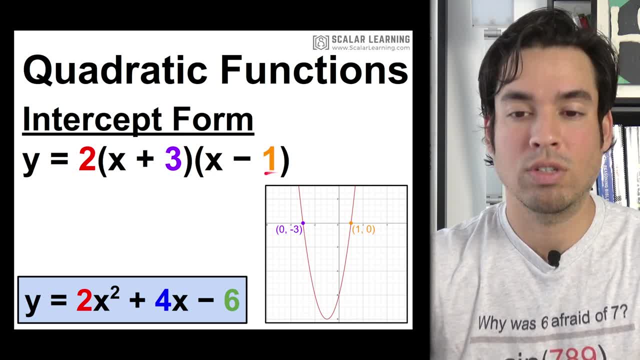 and it's gonna zero out the whole thing. likewise, if I plug in a positive one, right, you see that x intercept the positive one zero into here- it's gonna zero out this entire piece, which, zero times anything, is zero. so again we'll get a function value of zero. now we're gonna talk about something called 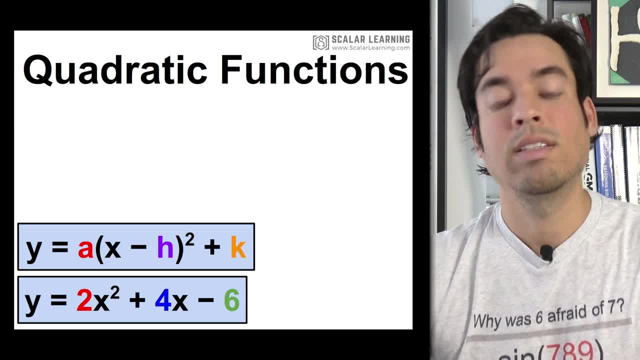 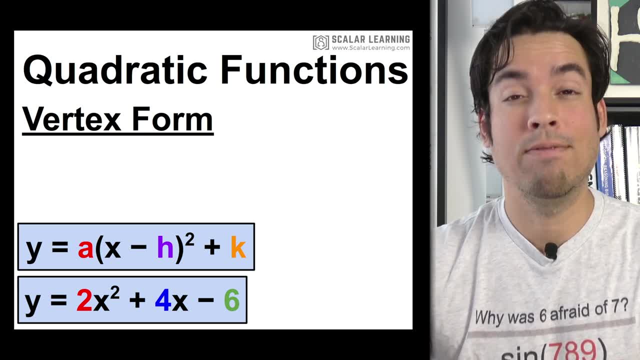 vertex form. so here's vertex form. it's: y equals a times x minus h, squared plus K, and in this case that H and K value actually show us the vertex, remember, which is again either that max or min point of the function. so now we see that. 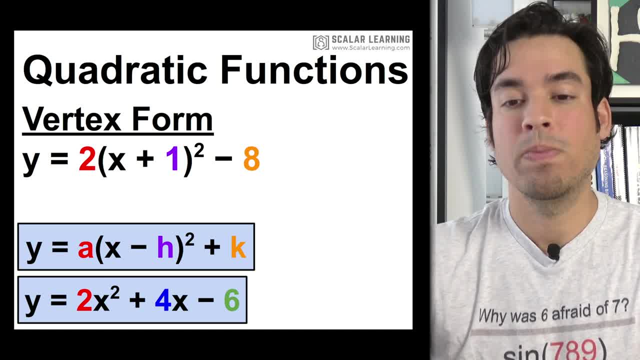 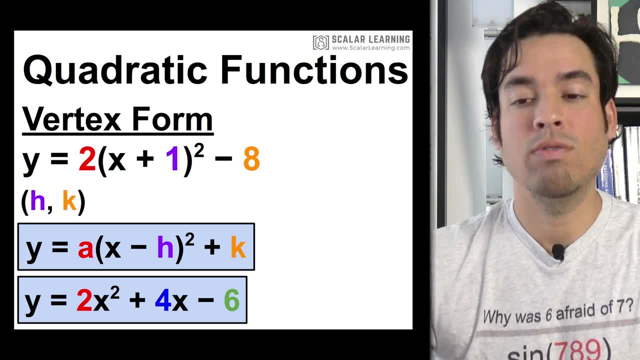 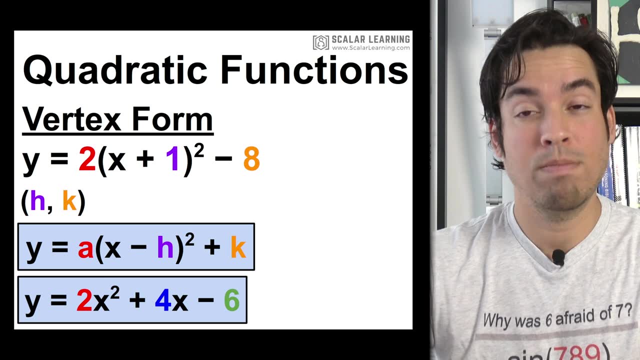 once it's reformatted in this form, are presented in this form: that value, that purple value, is the H, which is the X coordinate of the vertex, and that yellow value, that negative eight, is the K value. this one is a little trickier because you have to remember to negate the purple one. 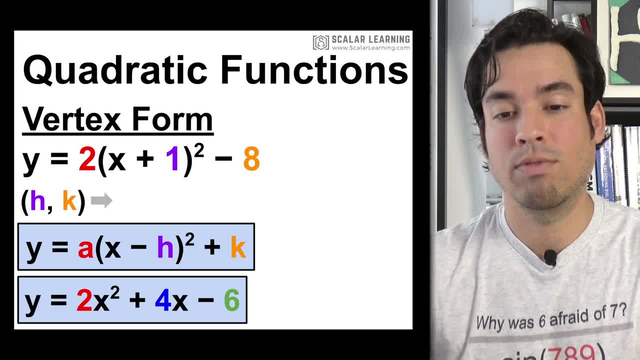 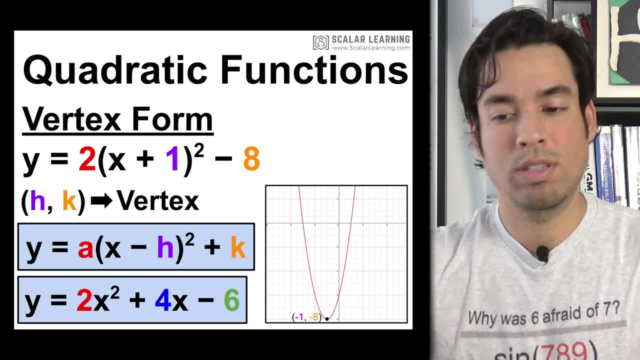 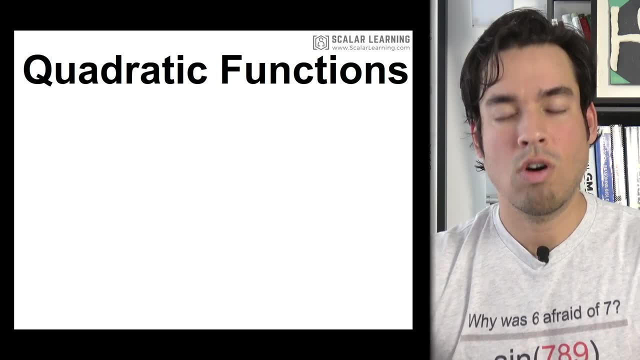 and keep the yellow one the same. so this is actually gonna have a vertex of negative one, negative eight. so you see that. so again, that one value is negated to its opposite, but that eight, which is a negative eight, actually is kept the same as negative eight. now let's talk about how do you find the vertex, if it's. 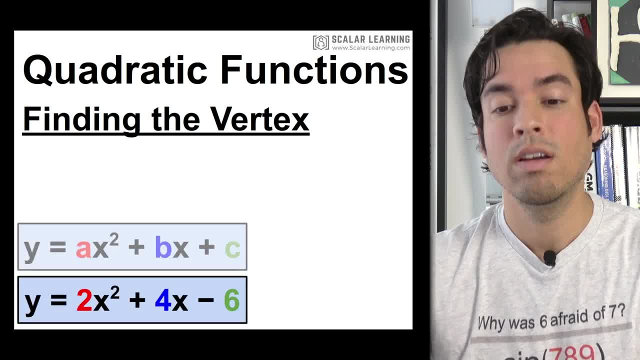 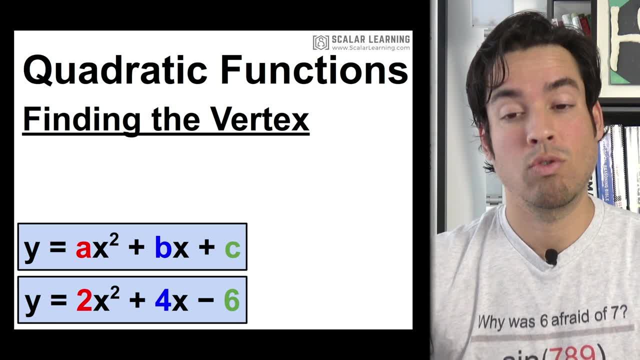 not in vertex form. so again, if it's in vertex form, it's pretty easy to see. but let's take that. take this example: when it's in standard form. now there's a really important formula that you've got to know in order to find the vertex. so it, when it's in standard form, you can find. 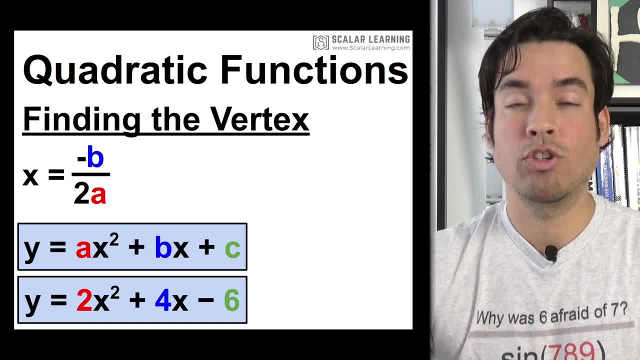 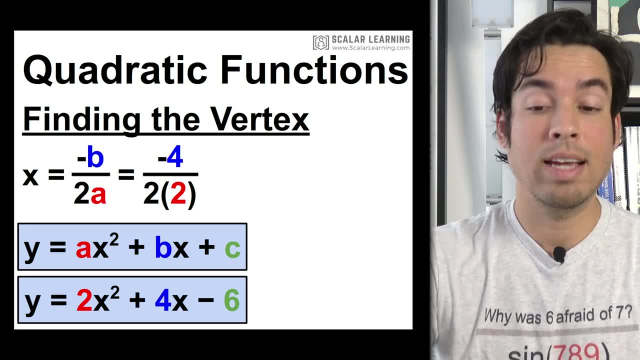 the vertex by putting negative B over 2a and then that will be the X value of the vertex. if we look in this example here, the four is the B value. so I say negative 4 over 2a. 2a is 2 times 2, so then we get negative 4 over 4, which of 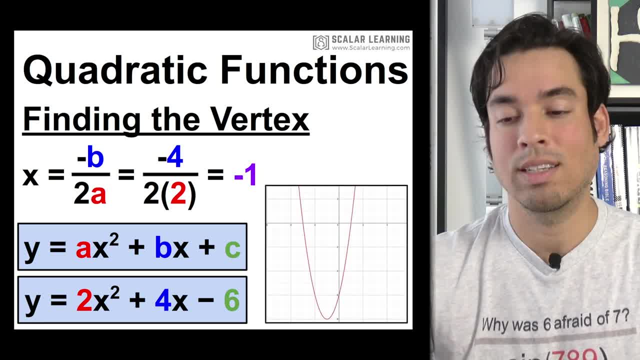 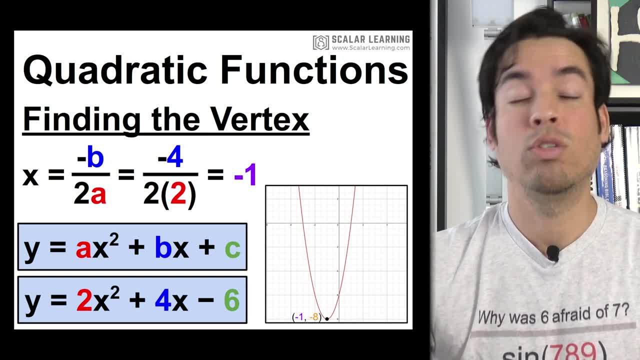 course, equals negative 1 and that is the X value of the vertex. and again, as we saw before, and there it is negative 1 comma, negative 8. now how do we find a vertex if we plug in that negative 8? you simply take the negative 1 value. 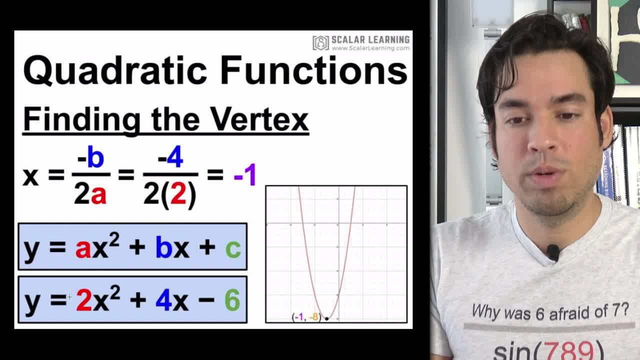 that X value and you plug it into the function. so just to show you what that would look like here, what we'd be doing is I'll take negative 1 and plug it in for all the X value. so first of all, it would be 2 times negative 1 squared plus. 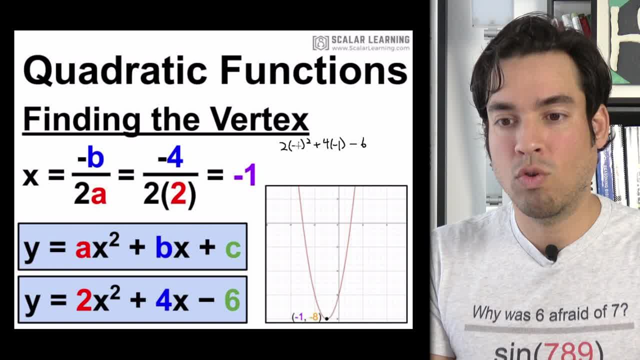 4 times negative: 1 minus 6. this of course negative 1 squared is of course 1 times 2 is 2, 4 times negative. 1 is negative 4. negative 6 just stays as is. 2 minus 4 is negative. 2 minus 6 is negative 8. so 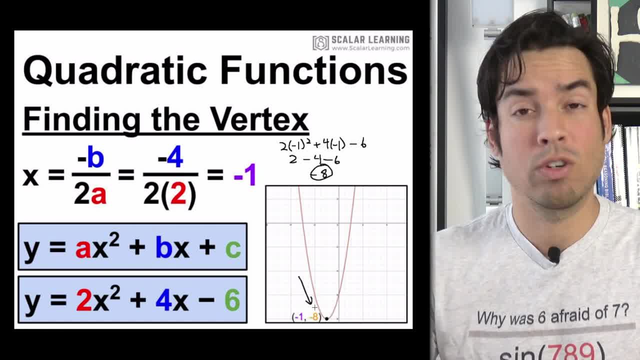 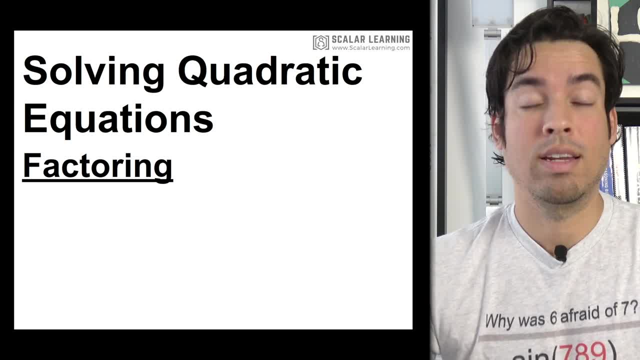 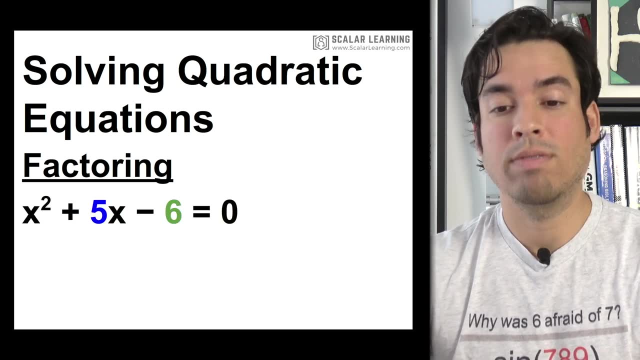 that gives us our corresponding Y value of the vertex. now let's talk about solving quadratic equations. so again, a quadratic equation is simply an equation where the highest degree is 2, so the first thing that we want to become aware of is factoring. so in order to factor this, we have to ask the question: what? 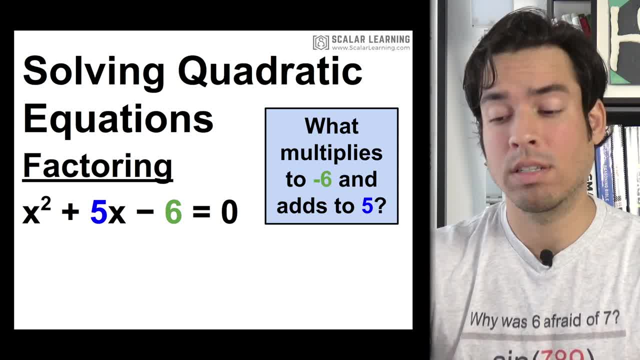 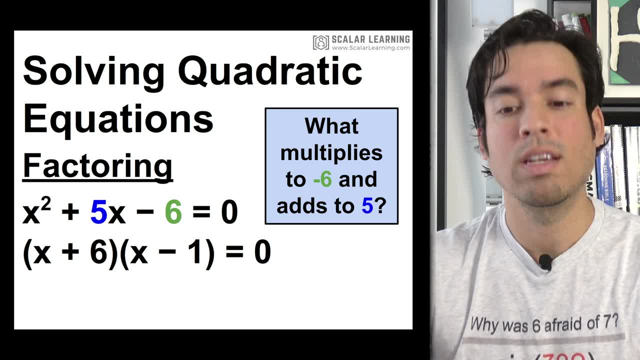 multiplies to negative 6 that green value and adds to positive 5. okay, so what would do that? well, that would be 6 and negative 1, and that makes sense, right. 6 times negative 1 is negative 6. 6 plus negative 1 is positive 5 and that's. 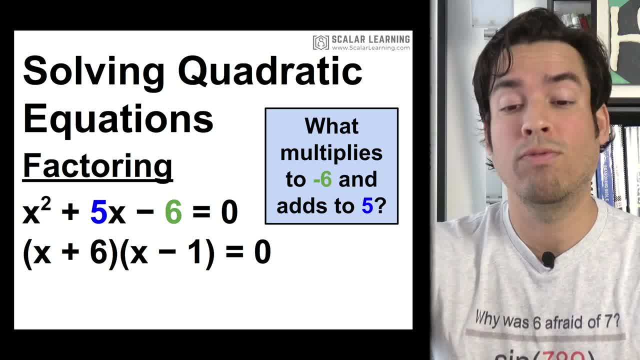 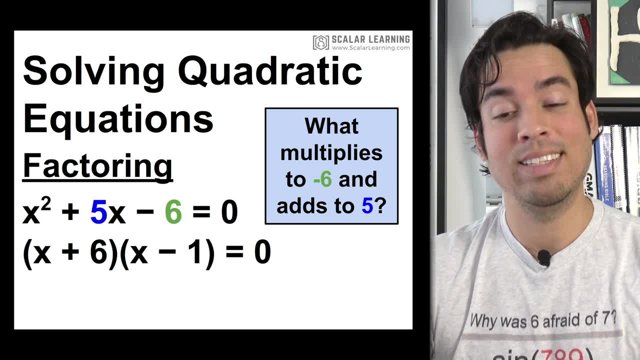 how we split it up. we split it up into those two binomials and if we were to FOIL we would come back to that original equation. and now the solving this equation gets really easy, because I can look at each individual binomial and I say, hey, what makes the one on the left go to 0? well, it's negative 6 because 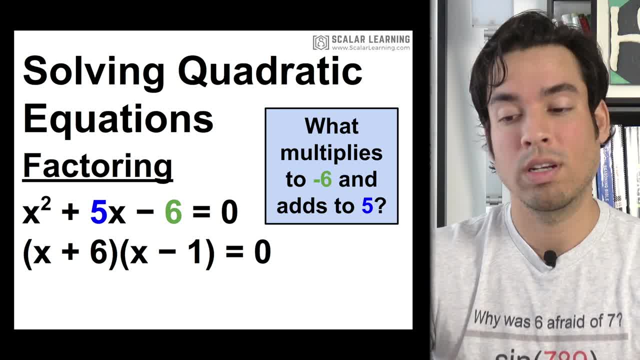 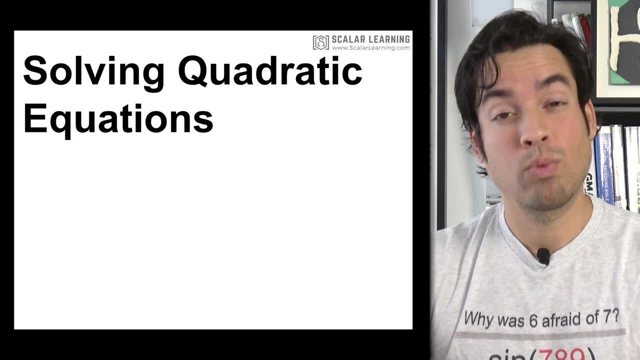 negative: 6 plus 6 is 0. what about on the right? 1 minus 1 equals 0, so my two solutions are negative 6 and positive 1. next we're going to talk about something really really powerful called the star method, and this has to. 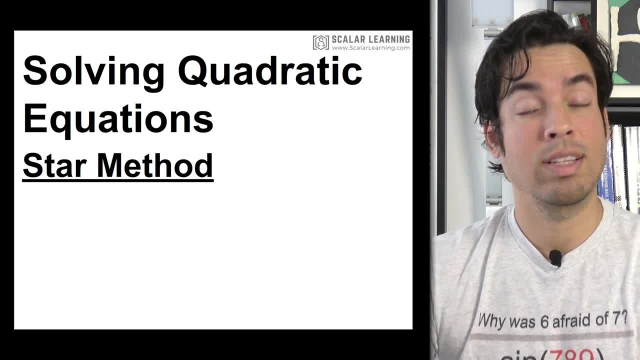 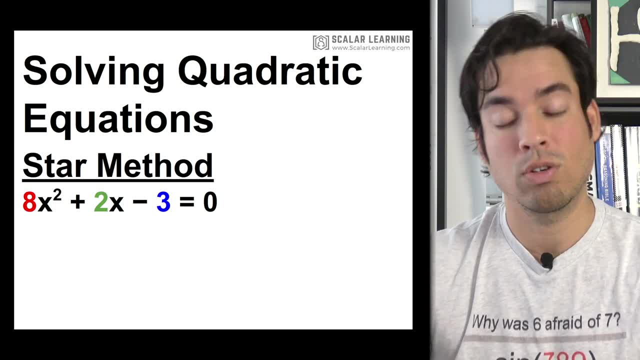 do with factoring quadratic equations when there is a leading coefficient. so let's take an example: here we've got 8x squared plus 2x minus 3, so this is a lot more difficult to factor. so here's the protocol and again the the chance that. 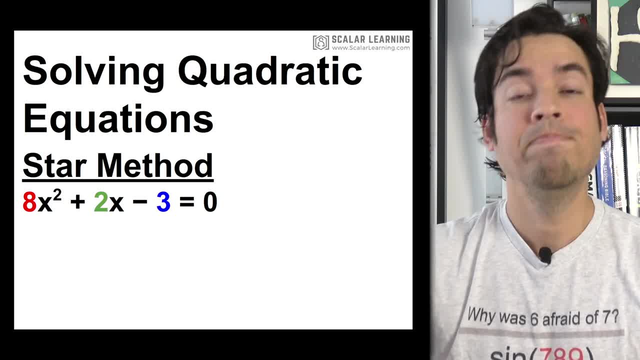 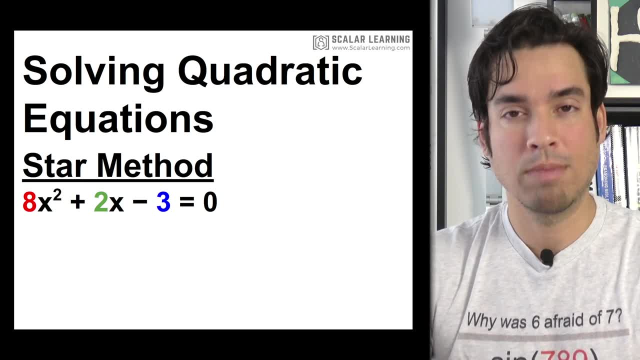 you're gonna get something like this on the SAT is low compared to quadratics with the leading coefficient of 1, but I just want you to be aware of this and put this in your back pocket if you have the time to understand this technique. so check it out. what I'm gonna do is I'm gonna 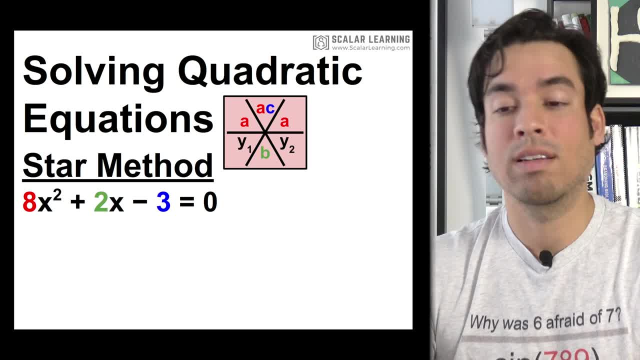 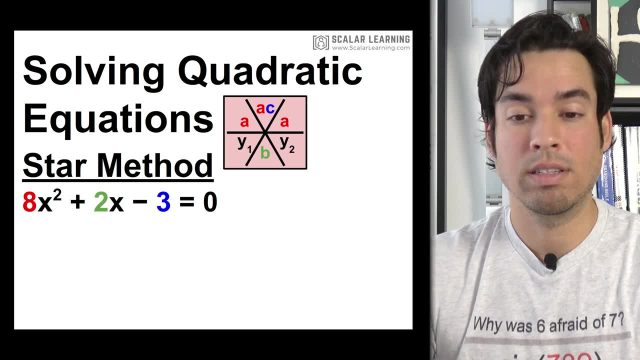 create this little star and the top left and top or right thoughts. I throw in a in the top slot, I throw in a times C and then the bottom slot is B. so let's check that out in practice. so I have 8 and 8 on the top left and top right again. 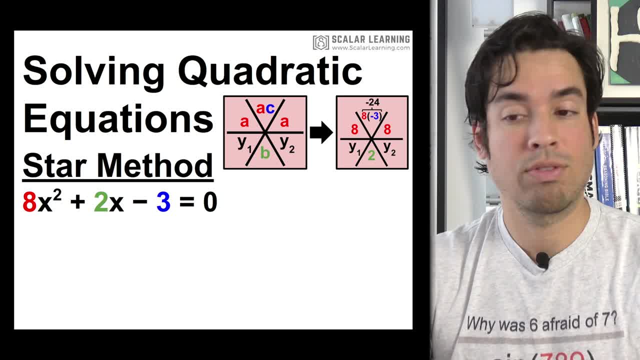 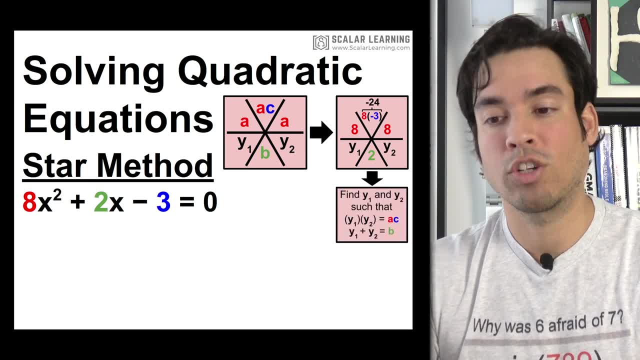 that corresponds to the a value. then I have 8 times negative 3 on top, which is negative 24, and I throw that 2 on the bottom. now, why do I do this? okay, because now I ask the question of what values of y1 and y2, meaning what two values can I find that multiply to? 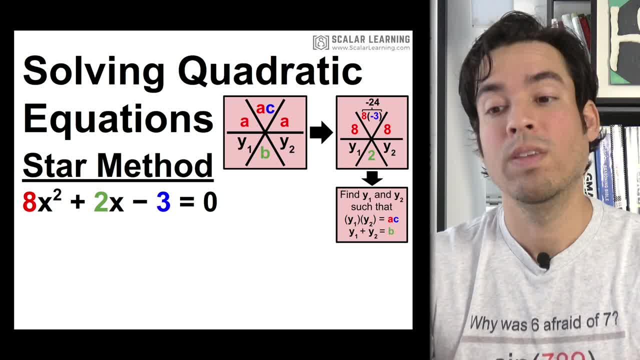 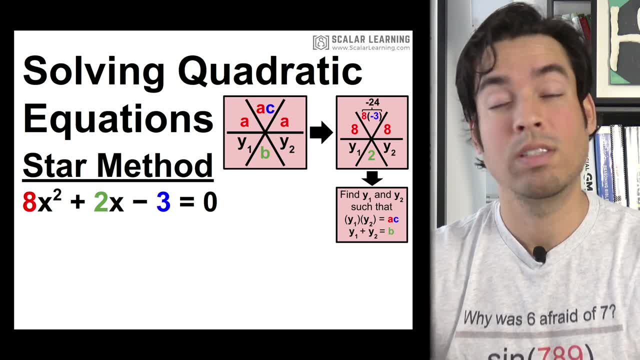 negative 24, but add to positive 2. so the answer, of course, would be 6 and negative 4. right, 6 and negative 4 multiplies to negative 24. 6 plus negative 4 is positive 2. so we know that it's going to be 6 and negative 4. so I throw those. 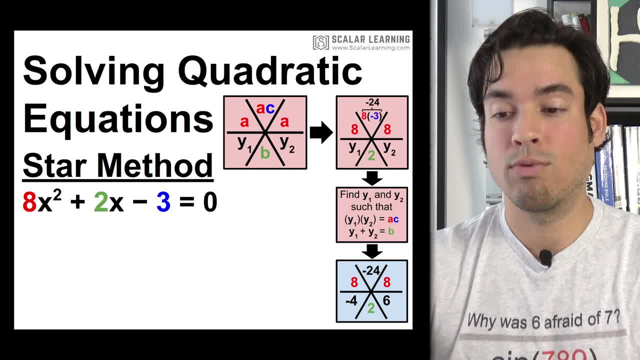 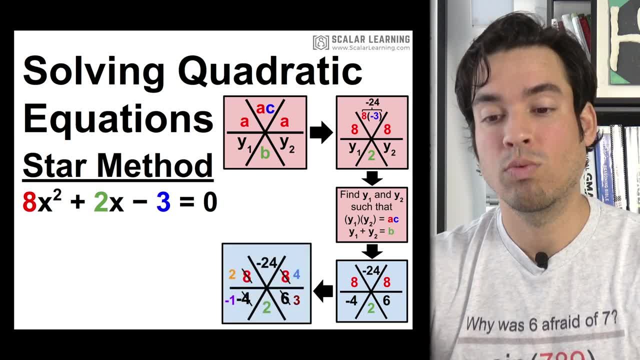 throw those down there now. look at that 8 over the negative 4. look at that 8 over the 6. now I want to. those are the key pieces right now. I want to treat those like fractions, and so what I'm gonna do is I'm gonna reduce both of those, right. 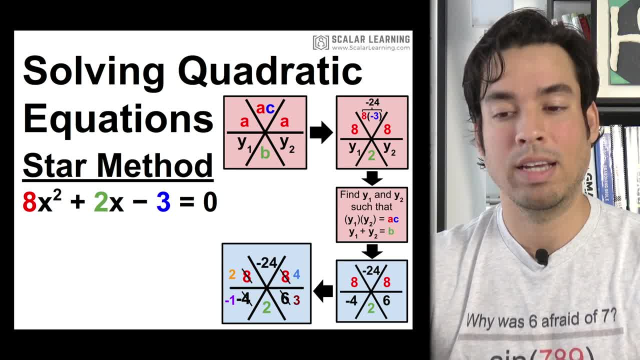 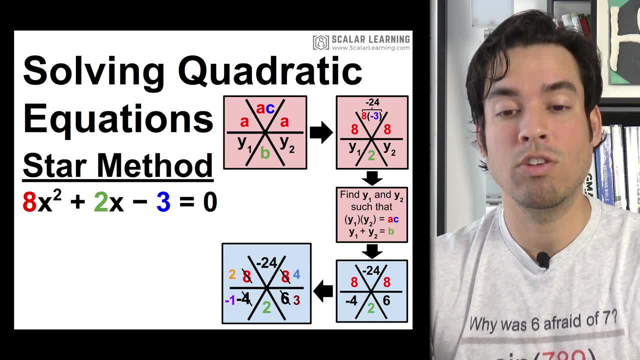 you notice that 8 over negative, 4 reduces to 2 over negative 1, 8 over 6 reduces to 4 over 3. now the most important part is we take that orange and purple value- that's gonna make one binomial. and we take that blue and brown. 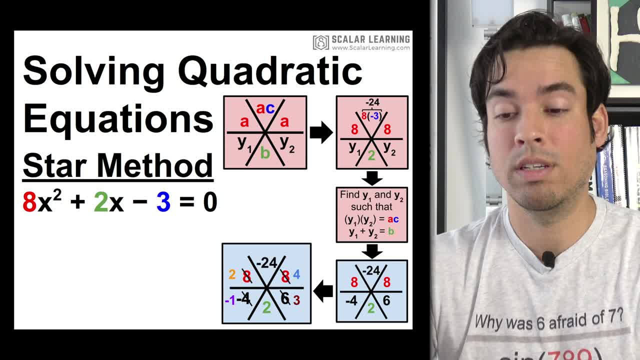 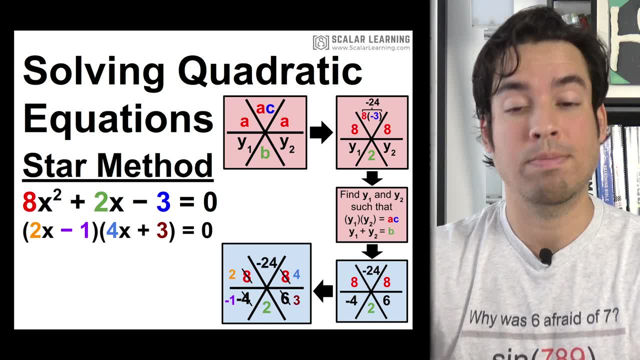 value and that's gonna make the second values of the second binomial. so this is how it looks. it's gonna be 2 and notice, the top value always goes with the X. so it's gonna be 2x minus 1 times 4x plus 3. and now we 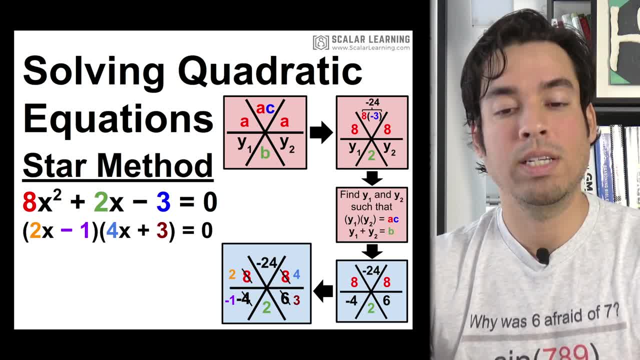 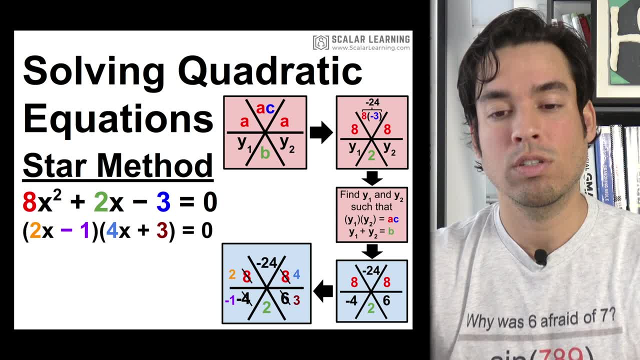 factored it, and what are the zeros in this case? well, what makes that first binomial go to 0 is going to be 1 half. what makes the second one go to 0 is negative 3 fourths. so again, our answers for this are 1 half and negative 3. 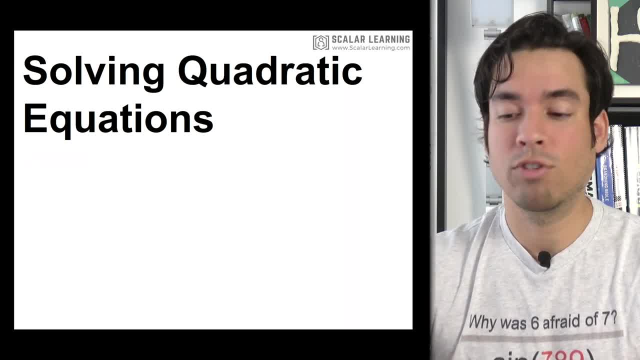 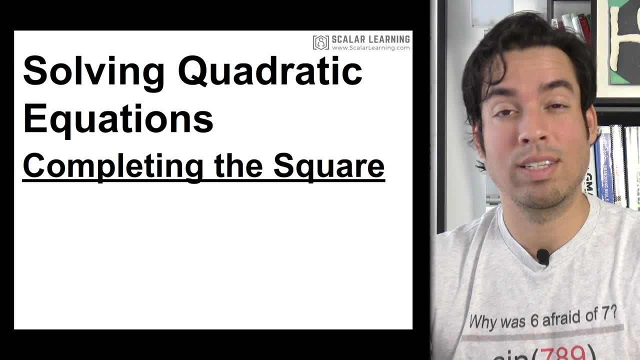 fourths. next, we're going to talk about another method, same thing, for solving a quadratic equation, and that's called completing the square. now, to me, completing the square is not really a necessary technique, because you can always solve using either factoring or something we're going to talk about. 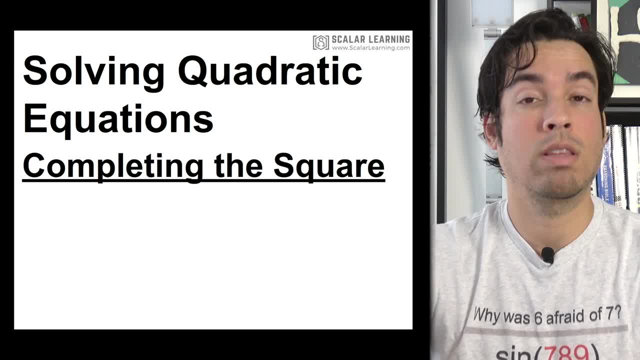 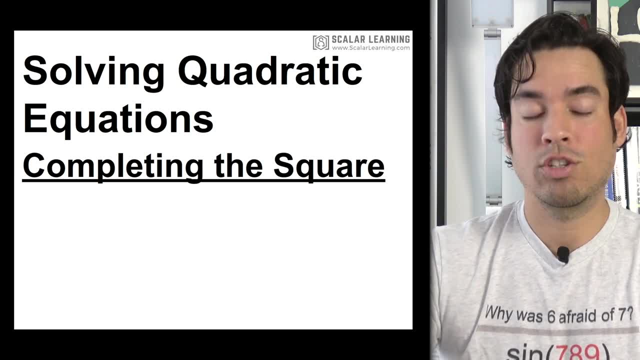 shortly, which is the quadratic formula. but the one good thing about the process of completing the square is it's helpful later on to show in another video when you're trying to get a circle equation, for example, into standard form. so we're going to take this example of x squared minus 6x plus 8 and we're going to use 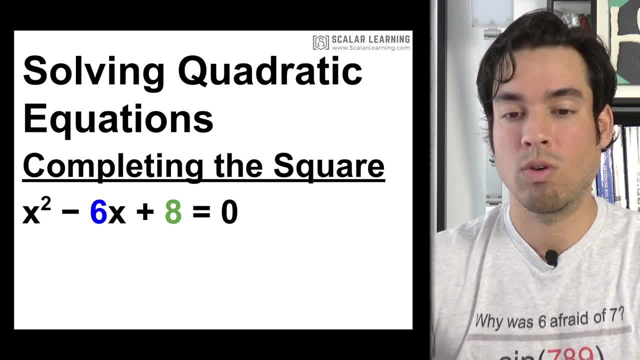 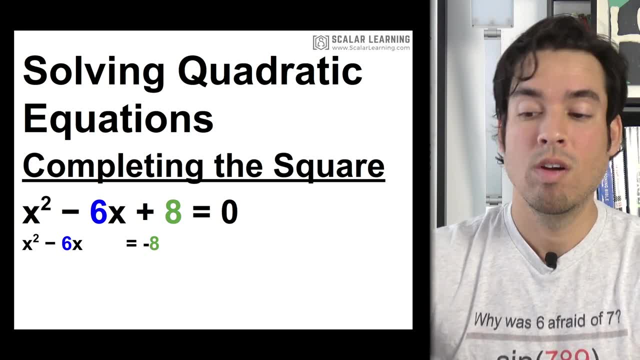 the completing the square process to actually solve for x. so first, what I'm going to do is I'm going to subtract both sides by negative 8. so you notice, I put the negative 8 on the other side. okay, then the next step is that blue value, that's 6. I'm going to take half of that, which. 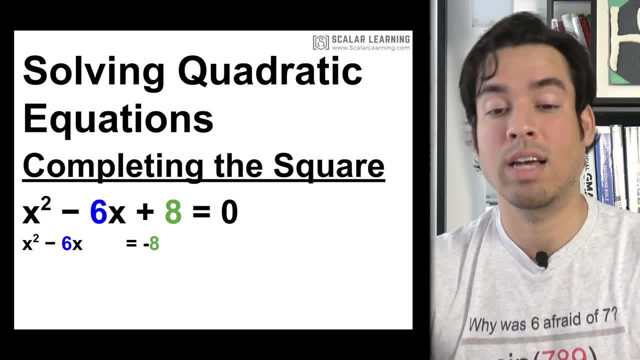 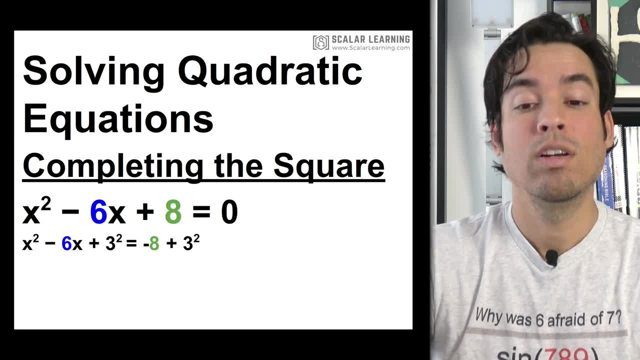 is 3, square it and add it to both sides. so we take half the blue value, which is 3, and square it and add it to both sides. so I'm adding 3 squared to both sides. remember, always must be a balance we got, whatever we do to the left side, we must. 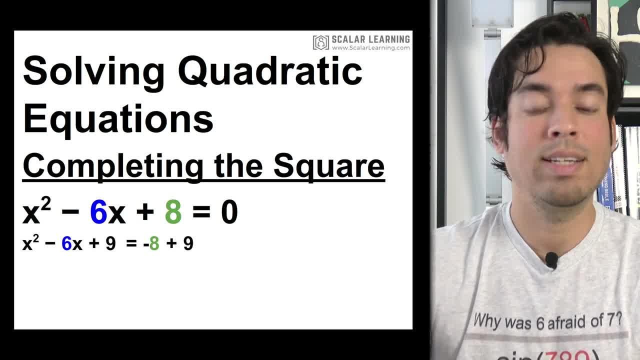 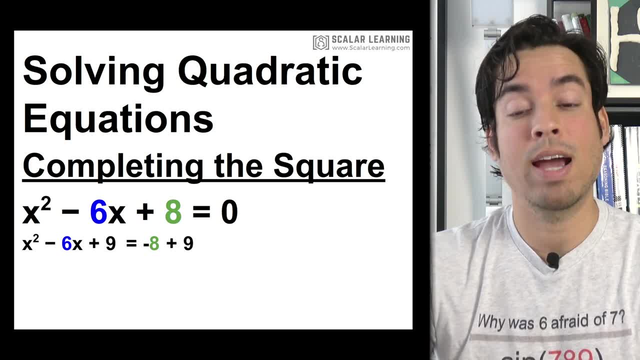 do to the right side. so, of course, 3 squared is simply 9, so I'm adding 9 to both sides. okay, what I've done on the left side is created a perfect square, meaning, meaning it's perfectly factorable, and that's the whole point. what does that factor to? it's simply x minus 3 times x. 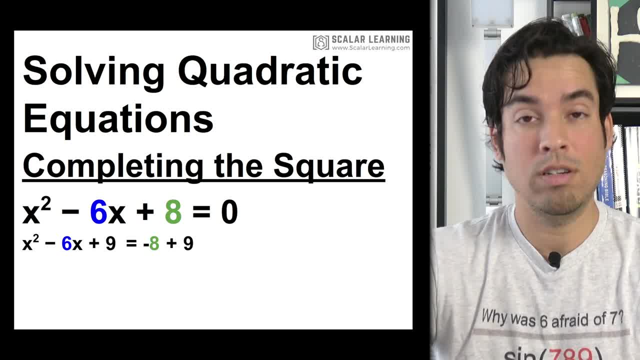 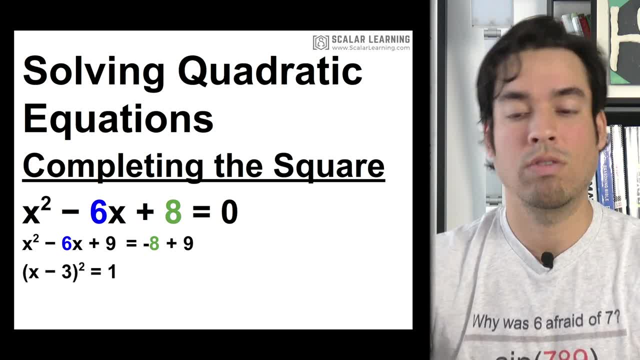 minus 3, and so when we, when we sort of engineer the trinomial in this way, we're creating a perfect square. so now, on the left side, I can factor that to x minus 3, squared, and of course, on the right side, negative, 8 plus 9. just simplifies. 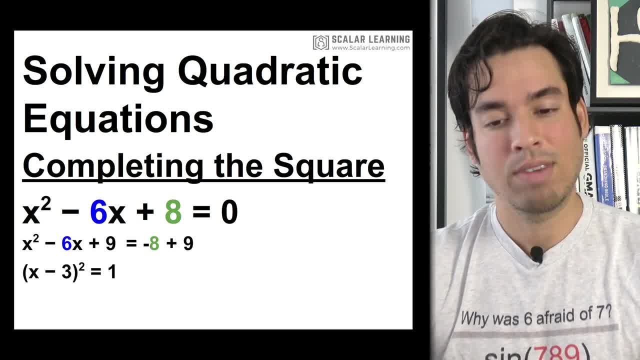 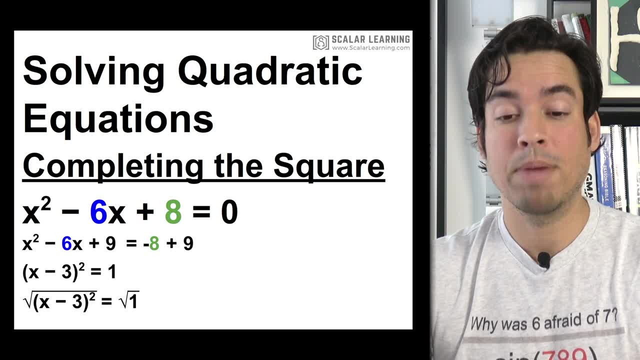 to 1. now we're in a great position because I've got a square on the left side. how do I undo that? simply take the square root of the left side and the right side as well. we have to keep the balance. so now it becomes: we get two equations. we get x minus 3 without the. 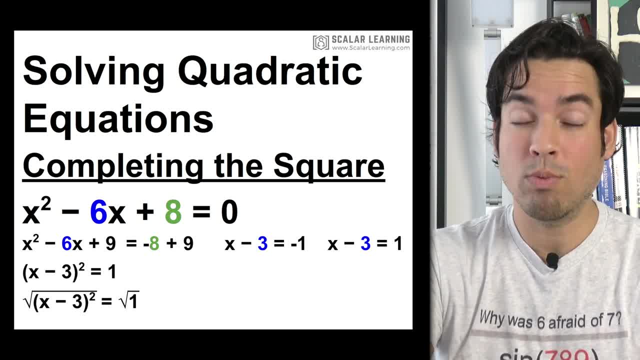 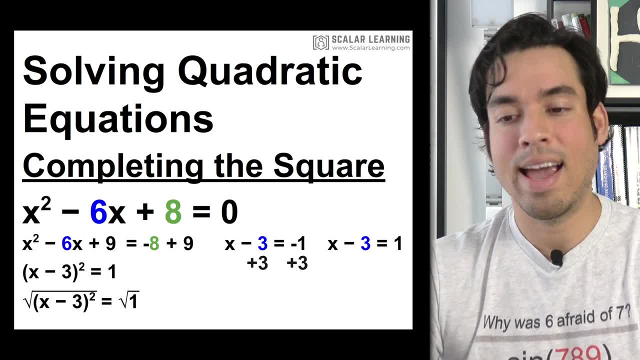 square equals positive 1 and negative 1, because the square root of 1 is both is plus or minus 1. all right, now we have two great equations and we can solve both of those. so on the left side, we're simply gonna add 3 to both sides and we 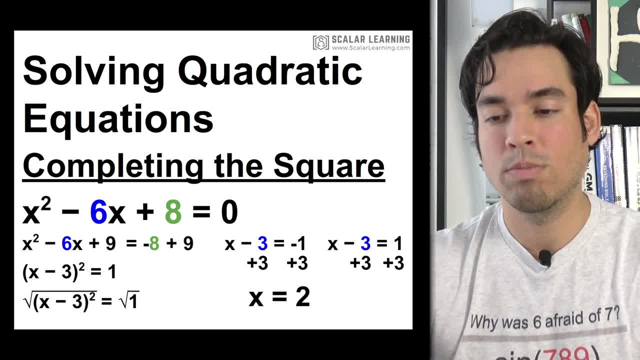 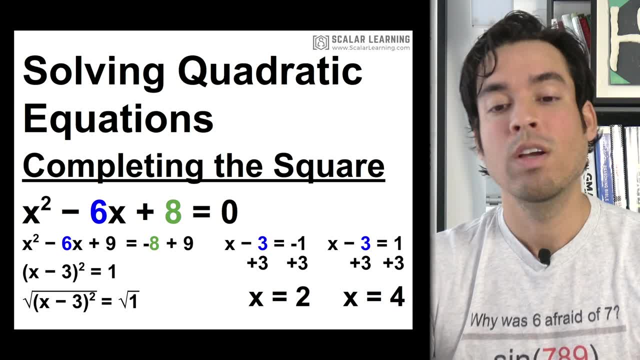 get x equals 2. beautiful, on the right side. same thing. add 3 to both sides and we get x equals 4. and if you want to double check your answer, take both of those solutions and plug them into the original equation. so the first one it'd be 4 minus 12, which is 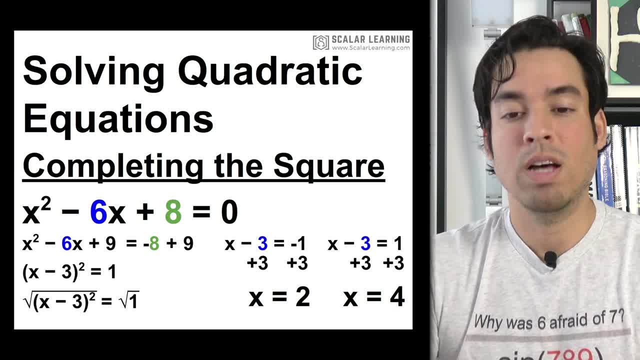 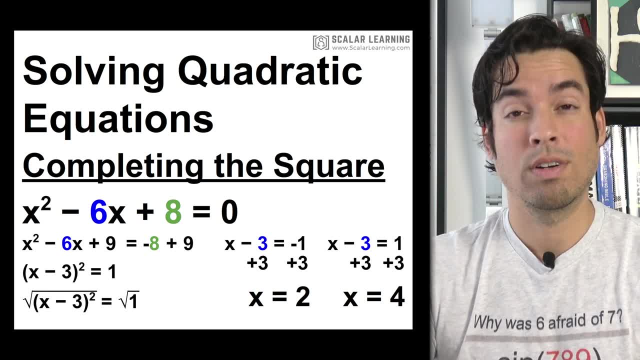 negative. 8 plus 8, 0, boom, it works. with a positive value of 4, it'd be 16 minus 24, which is again negative. 8 plus 8 is 0. now let's talk about one of the best ways that was is just foolproof. it will always work- is the quadratic formula. so 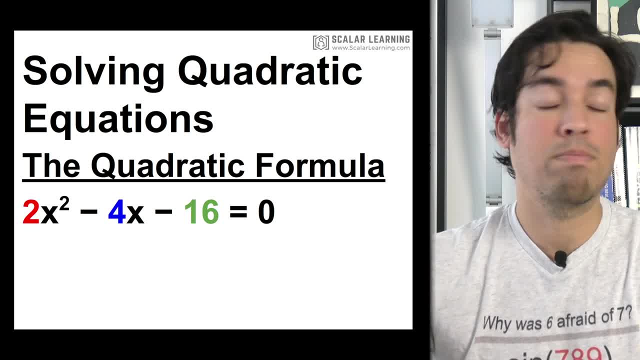 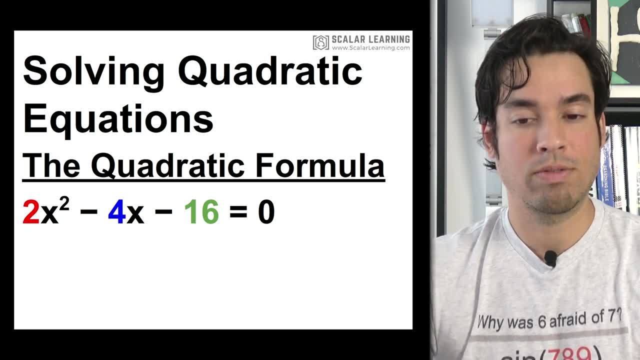 the quadratic formula. we're gonna use this set up here and plug it in and show you how it works. now, to demonstrate the quadratic formula, we're gonna start with this quadratic equation. so again, we're solving for X and here's how it works: the quadratic formula. is there? just something you got to memorize. you've got. 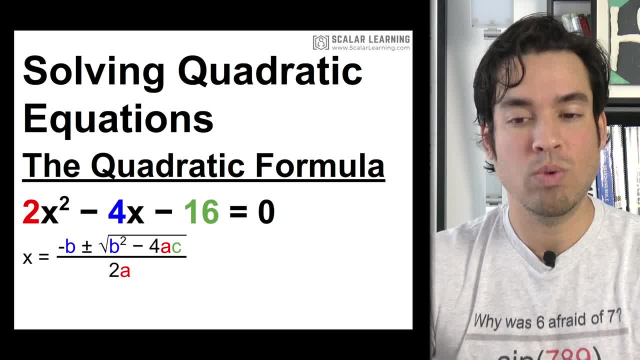 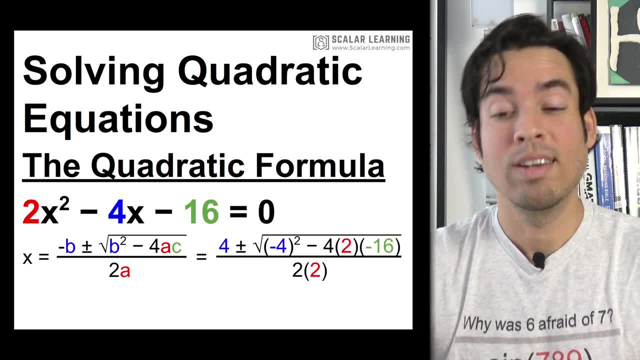 to commit it to memory: negative B plus or minus the square root of B squared minus 4ac over to A. but now if you know that it's just straight plug-and-chug, right. so guess what? the negative 4 is the B, the 2 is the A and the negative 16. 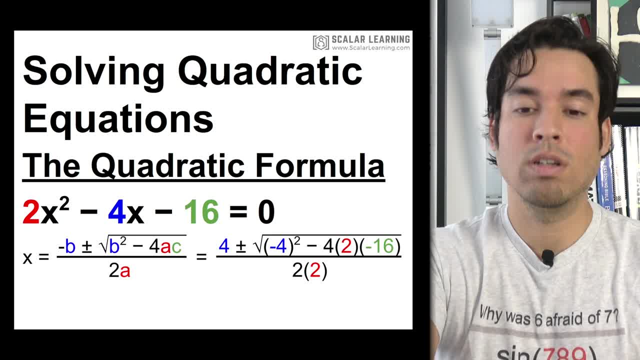 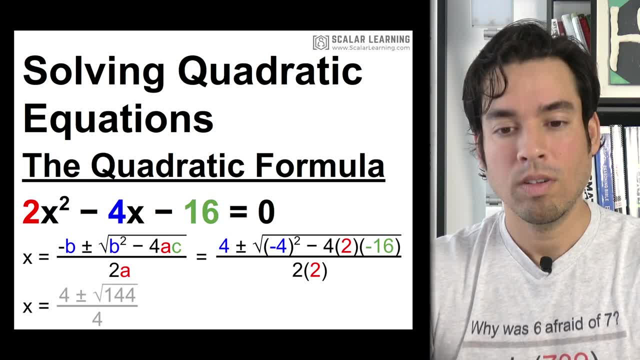 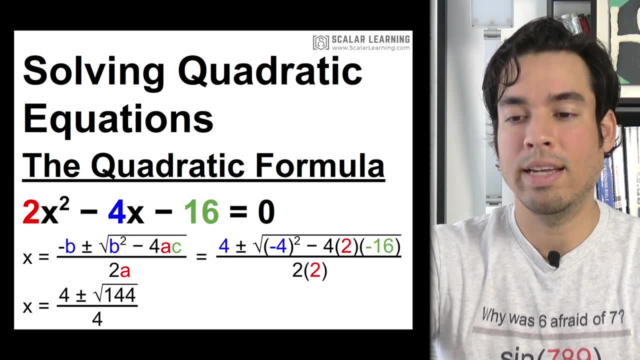 is the C. so you noticed. I just plugged all those in. I used blue to denote B, green to denote C and red to denote a. now we just multiply this out and you notice right on top that 16 and then it ends up becoming plus 128. gives you that 144. 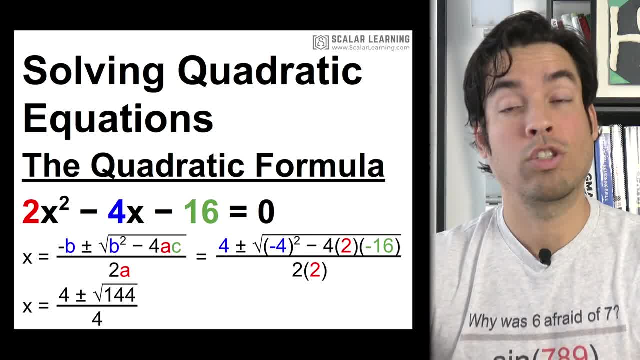 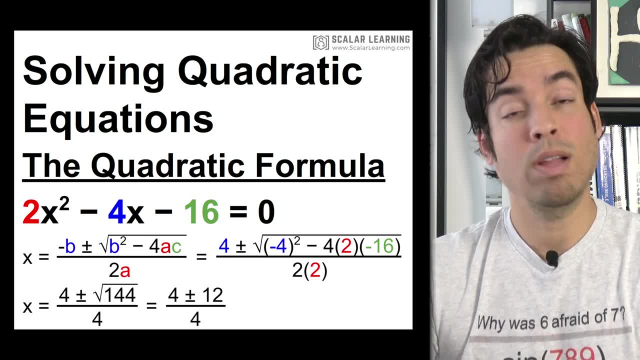 under the square root and the 4 2 times 2 at the bottom is 4. what's the square root of 144? it's simply 12. so now you got 4 plus or minus 12 over 4. so again it's 4 plus 12 over 4, which is simply 4, and 4 minus 12 over 4, which again gives. 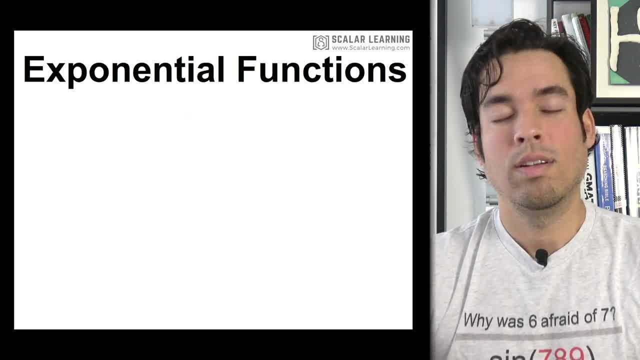 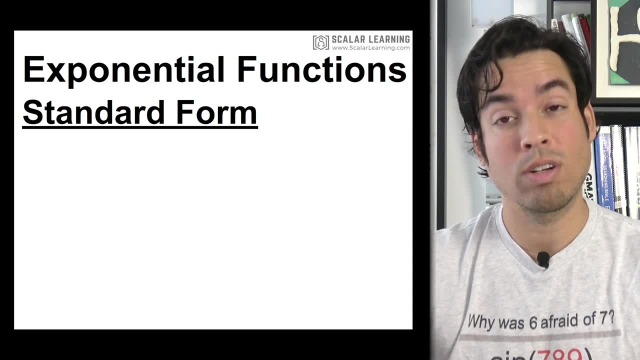 you negative 2. so those are the two solutions of this quadratic. next we're talking about exponential functions. this is also something that is tested on the SAT, and first we're going to start with the standard form, because you can learn a lot from the standard form. so standard form is: Y equals a times B to the X. 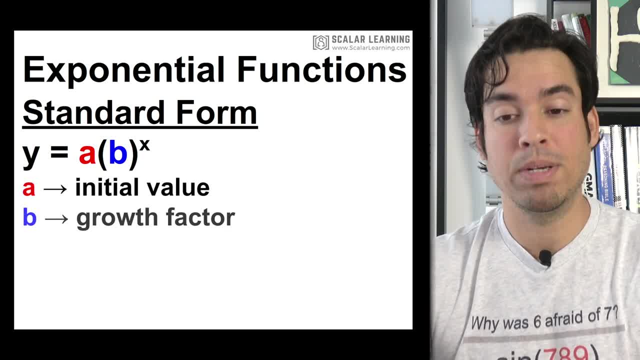 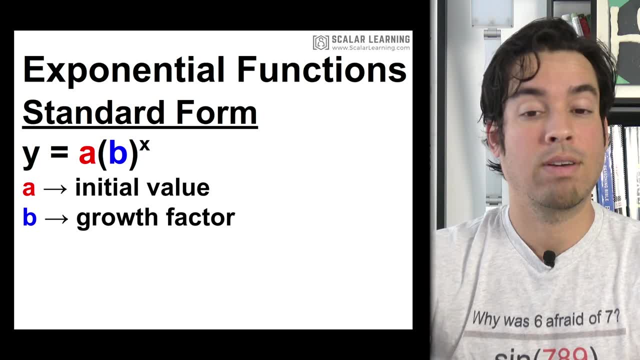 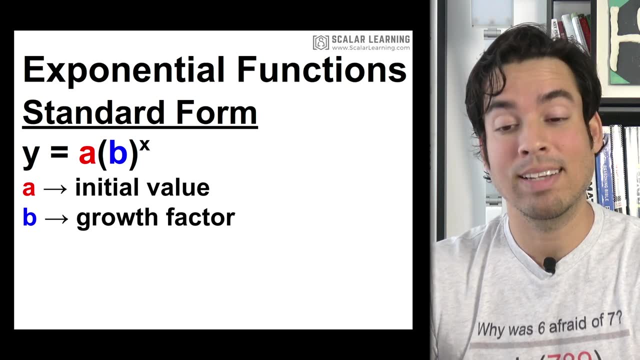 where a is your initial value or starting value and B is the growth factor, so the initial value. if we want to think about a, a bacteria strain growing, we might say, okay, initially we have 500 cells, 500 bacteria and b is the growth factor, meaning hey, it's growing by maybe five percent every hour, something like. 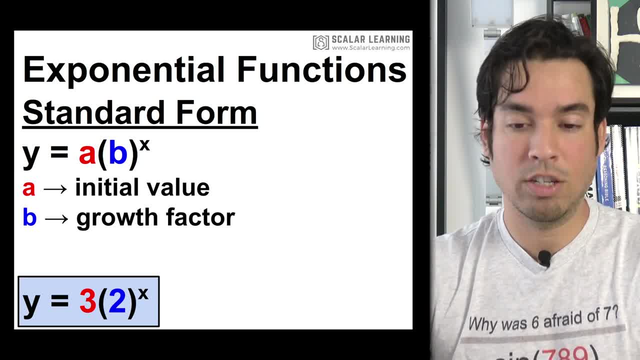 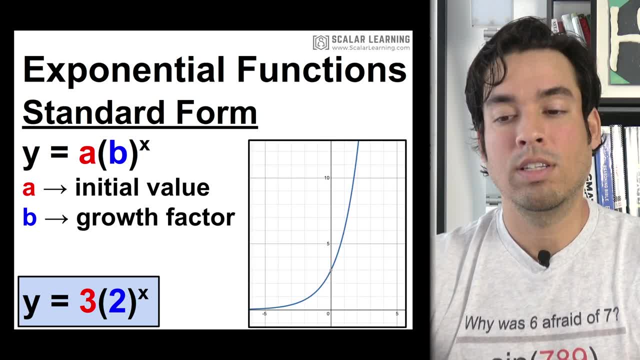 that now in this example down here, we have three being the initial value and here's a growth factor of two, meaning it's doubling every time unit, whatever the time unit is, whatever x is. this is what the graph of this function would look like, so you notice that upward sort of curve shape. 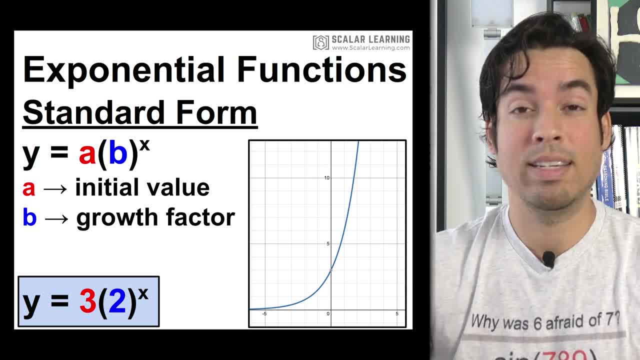 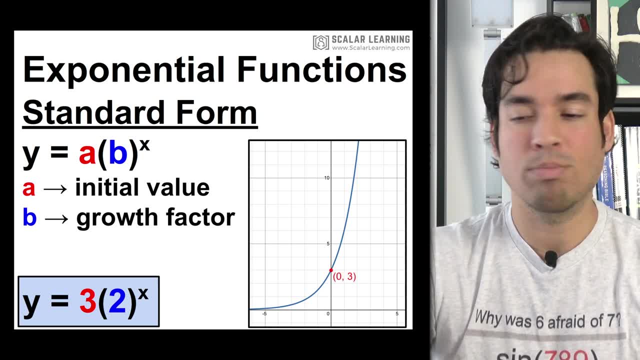 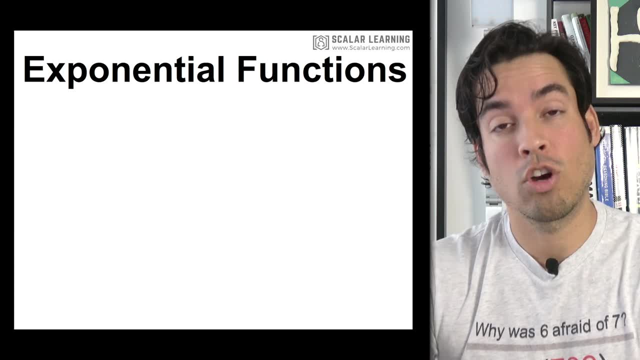 now remember I said that the three corresponds with the initial value. well, guess what? that also corresponds with that y intercept. so it's you notice a trend. initial values are the starting points- corresponds usually with that y intercept value. now there are two ways that exponential functions can go. they can either show growth or decay, where actually the value is declining, or 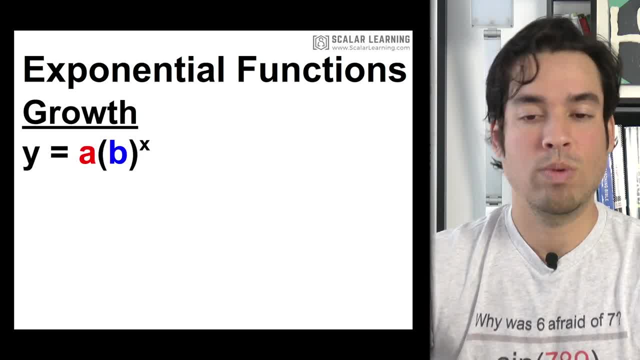 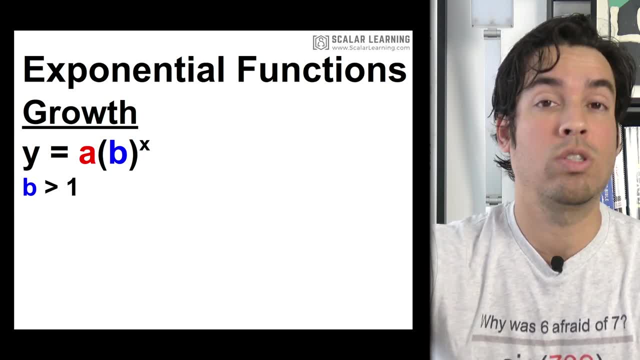 decreasing. so first let's talk about growth. so in the case of growth, we again have this standard form, and in this case b has to be greater than one. it can be 1.1, it can be 1.001. that's still exponential growth. when we talk about percentages, this is 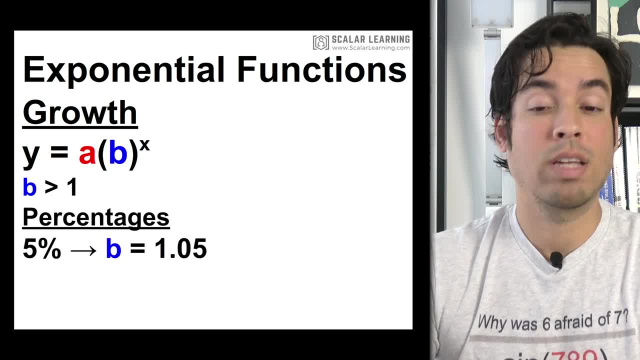 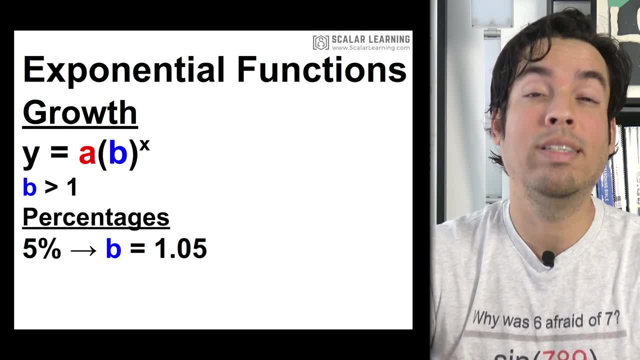 what it looks like. let's say somebody says: hey, it's growing by five percent every year. that means that the b is going to be 1.05. so what we do is we take that percentage, convert it to a decimal- it's decimal equivalent- and add it to one. okay, we gotta add it to one, don't just put 0.05 in there. 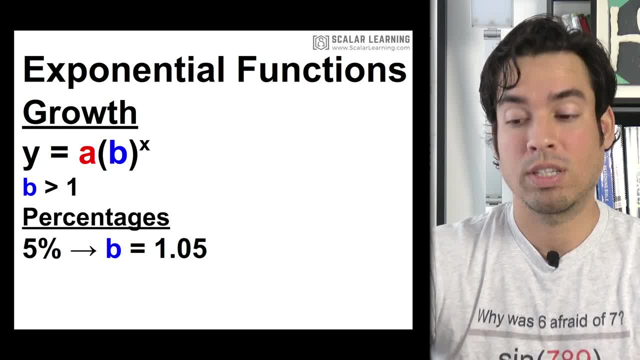 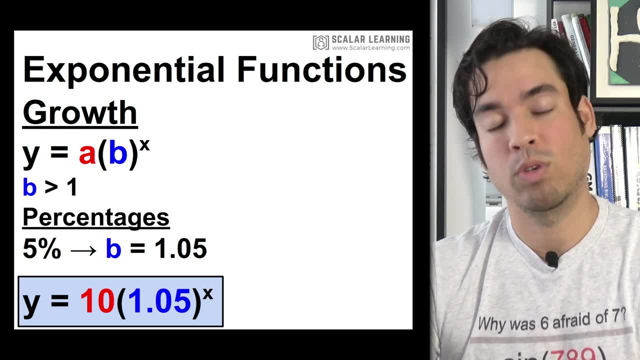 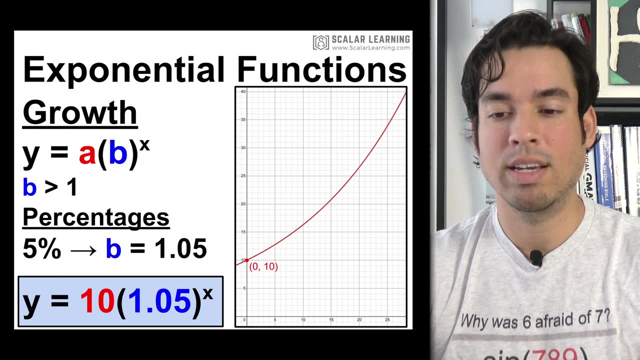 that would actually be decayed. so now it's growing by five percent every year. so here now we have something with an initial value of ten, with a growth rate of five percent per year, week, month, whatever the unit is, and again that graph looks like this, with our nice y intercept again starting. 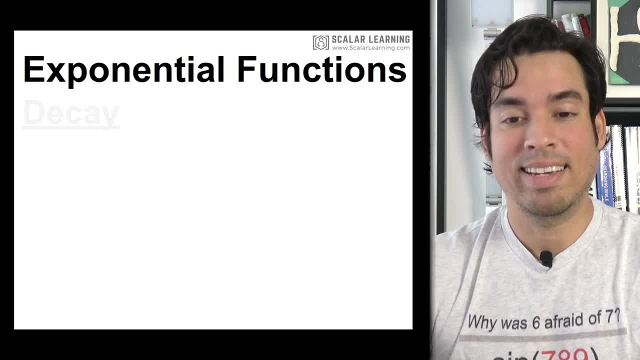 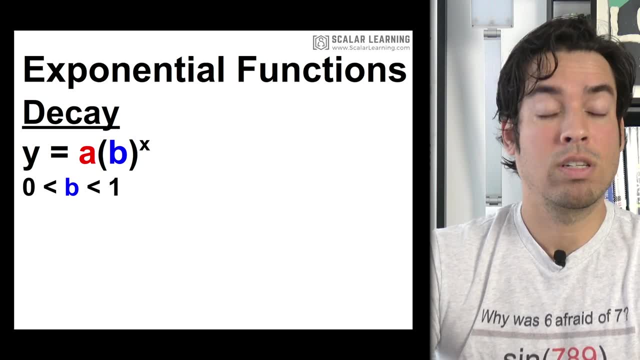 at the initial value of 0.10. now let's talk about decay. decay is going the other way. it's starting high and going low. so in this case, with our standard form, the b value is going to be between 0 and 1.. okay, not negative, it's going to be between 0 and 1.. so if we again we talk about 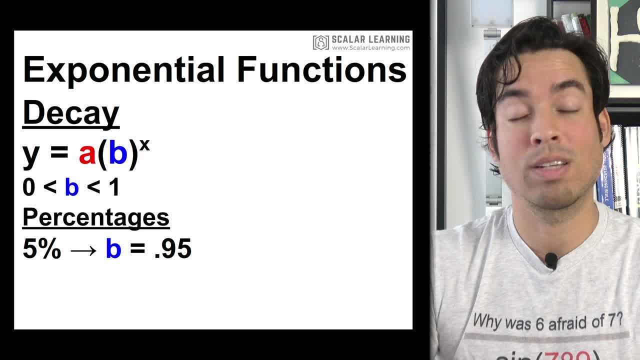 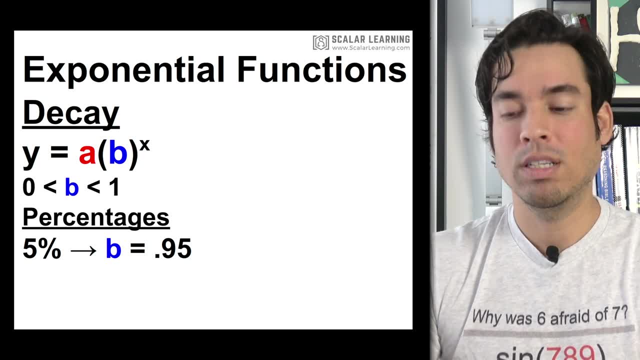 percentages. and now we're saying it's decreasing and decreasing. it's decreasing and decreasing by 5%. you don't put 5% in there, you put 0.95, okay. why does that make sense? because if I'm dropping by 5% every year, well, what am i retaining? I'm retaining. 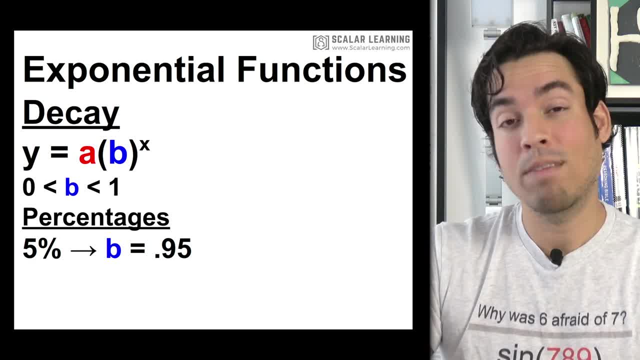 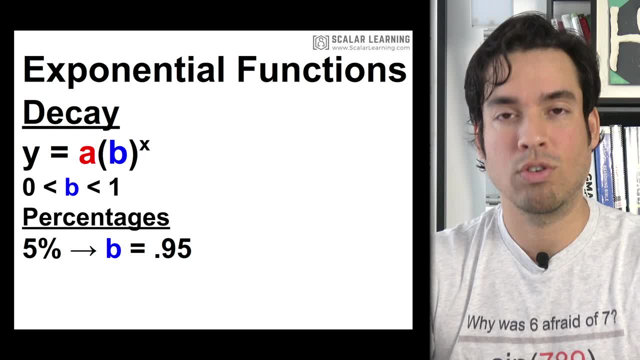 95%. so every year I'm having, I'm getting 95% of what I had the previous year. the other way to think about it is: if it's 5% decay, you do 1 minus 0.05 and you get 0.95. so again using that same example, a starting population of 10 decreasing by 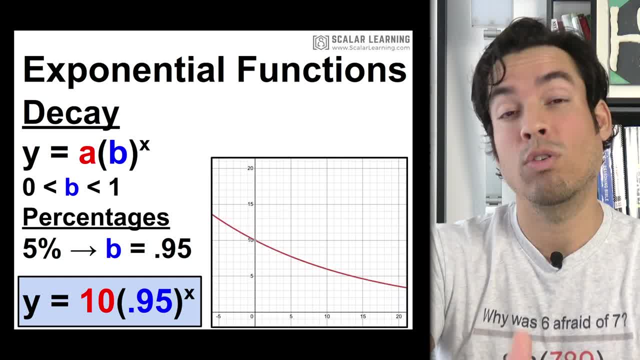 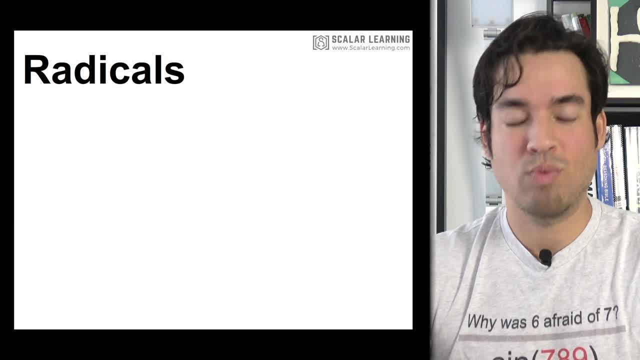 5% every year and that graph looks like this. now notice it's got a negative slope, it's sloping down, but that initial value, same y-intercept, a 0.10. now let's talk about radicals. we're taking roots, square roots, cube roots, all that stuff. 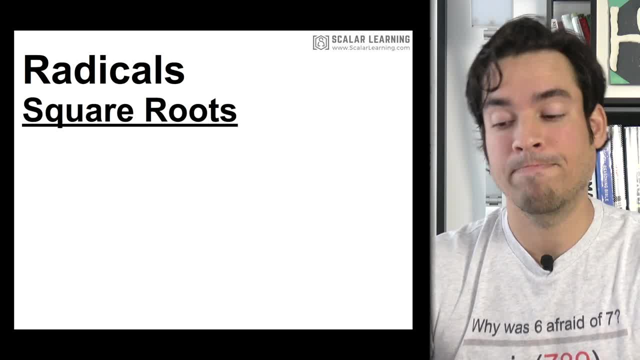 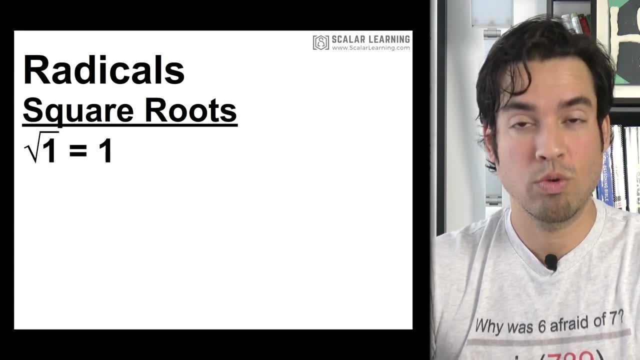 so we're gonna talk about the most basic one, which is the square roots. okay, square roots ask the question: what number times itself equals a given number? so, for example, square root of 1- and let's just think about the positive roots for now. of course we can have negative roots, but square root of 1 is: 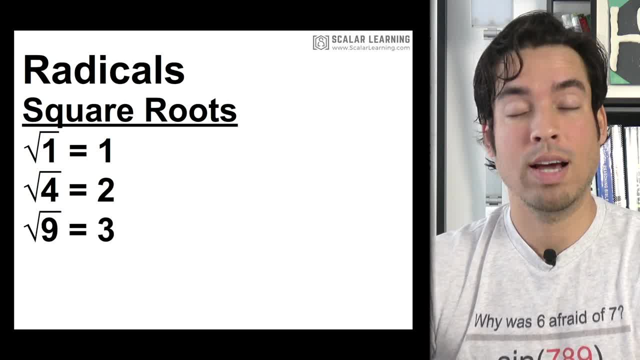 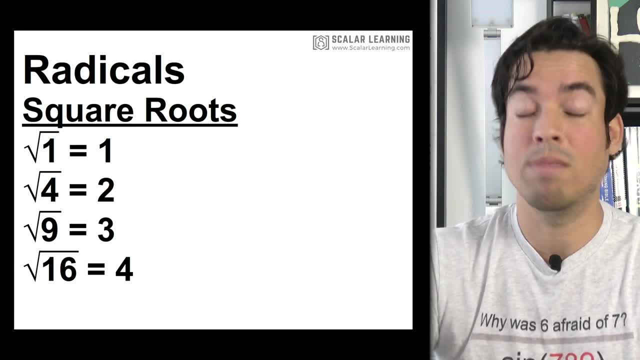 just 1. square root of 4 is 2. square root of 9 is 3. right, 3 times 3 equals 9. square root of 16 is 4. now notice I'm kind of skipping 10, 11, 12, 13, 14, 15, because they. 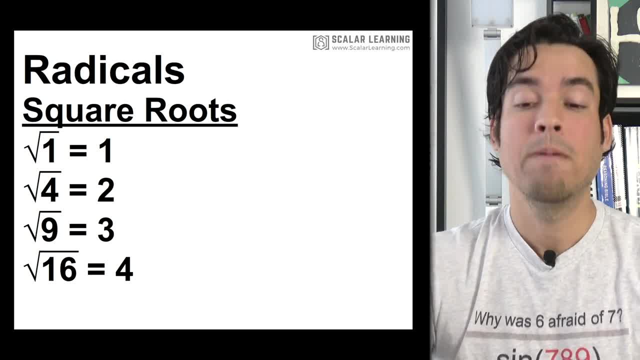 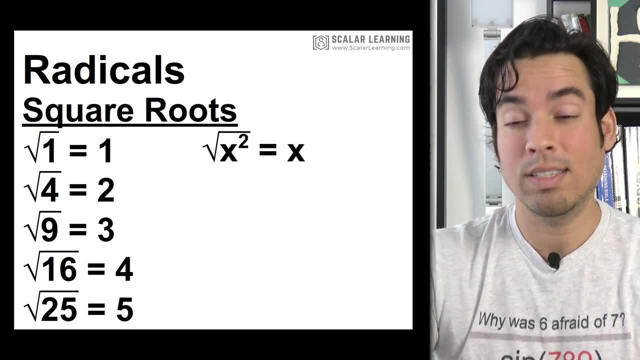 don't have nice perfect squares. they do have square roots, but they are irrational numbers. square root of 25 is 5. now if we look at variables, what's the square root of x squared? that's really simple, it's just X. we're sort of undoing that. 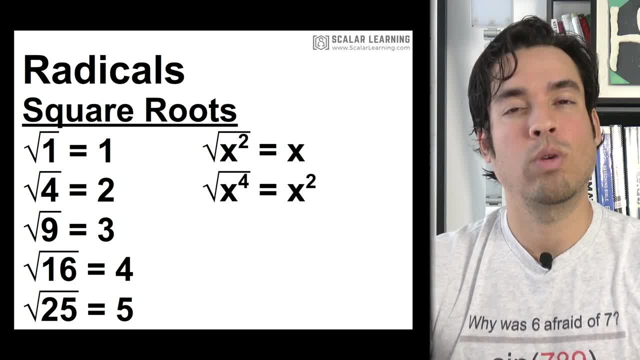 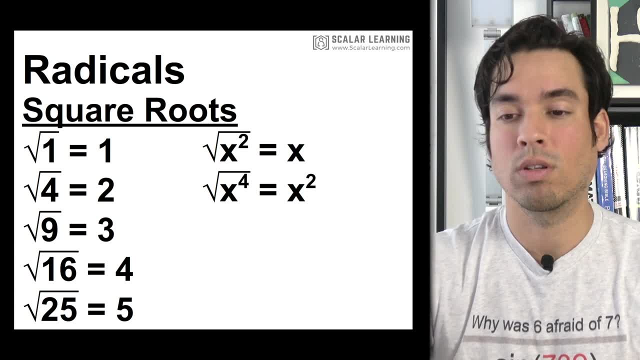 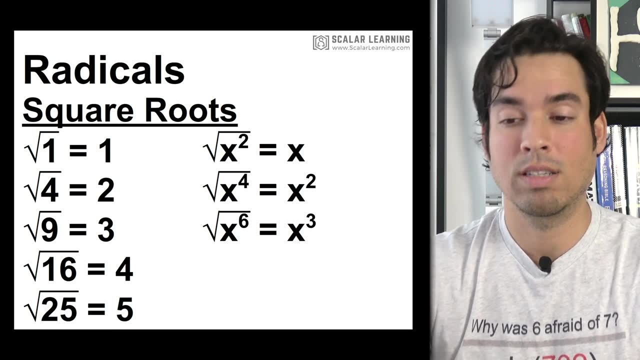 squaring operation, X to the 4th is x squared. why does that make sense? because we know x squared is x squared. an exponent with x squared is x square root. so what examples can we get of 이제? okay, so let's not do this forмиung. going on till. therefore, we have 2 x squared. 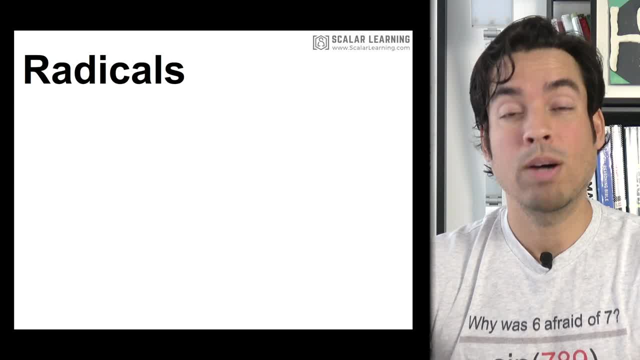 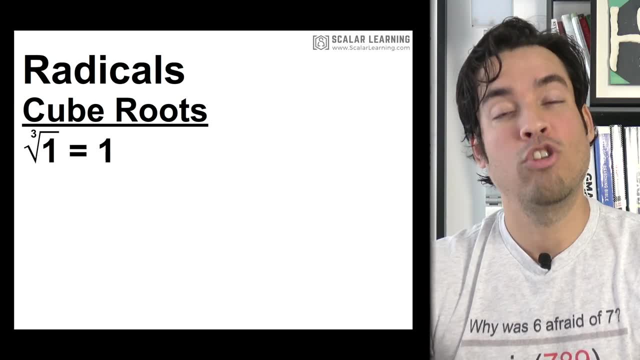 times x squared. we'd add the exponents and we'd get X to the 4th, likewise X to the 6th. I do X cube times X cubed. we'd add the 2, 3's, 3 plus 3 and we get 6. X to the eighth. square root is x to the 4th and finally X to the 10th. 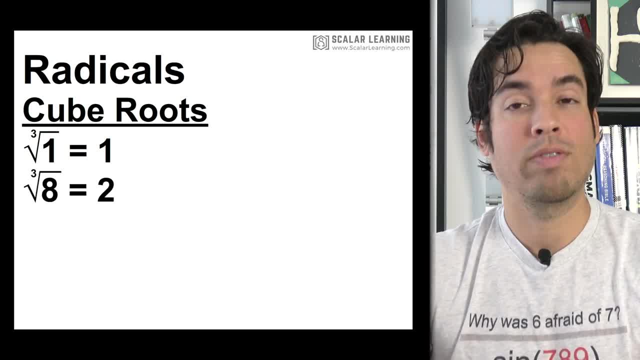 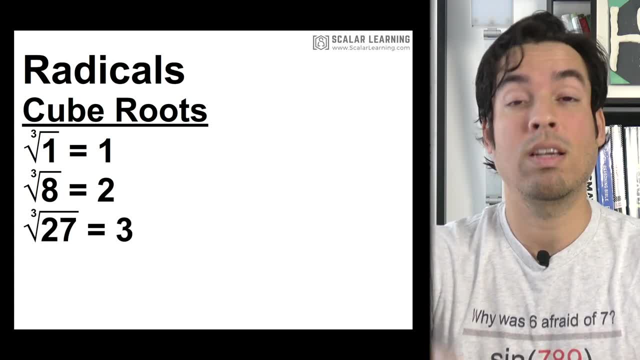 1 is 1.. What about the cubic root of 8?? Cubic root of 8 is 2, because 2 times 2 times 2 is 8.. A few more examples: cubic root of 27 is 3, and notice, I'm picking. 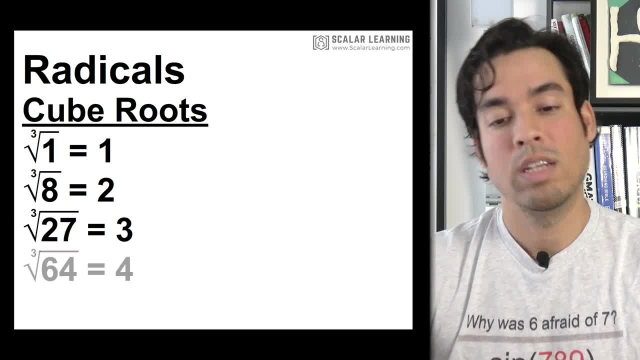 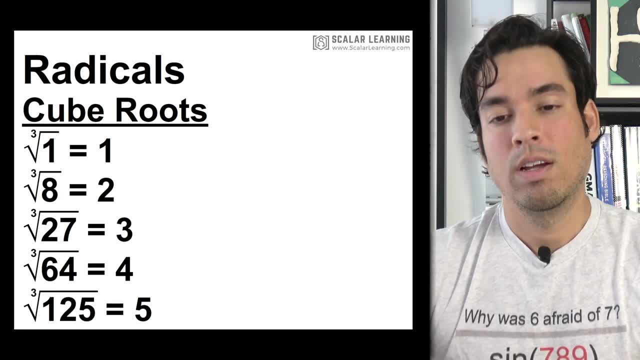 perfect cubes again on the left side: 1,, 8, and 27.. Next would be 64,. cubic root of 64 is 4, and, last but not least, cubic root of 125 is 5.. Now we're going to talk. 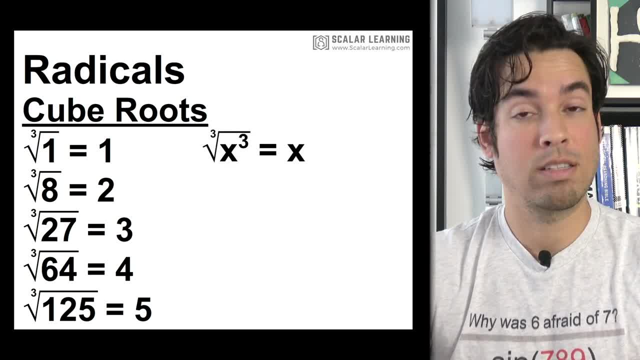 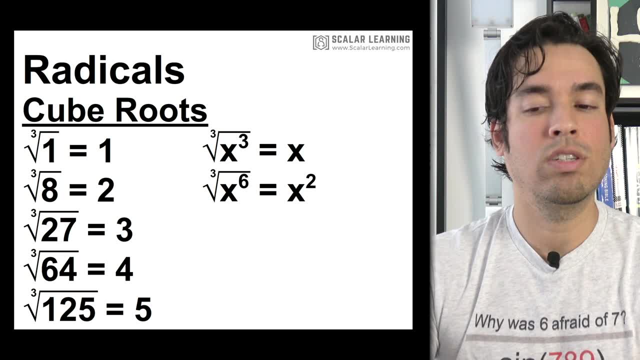 about with variables. again, cubic root of x- cubed has to be x. that makes sense. but now we have something like x to the sixth. it's x squared. So you'll notice a trend. it's almost like I'm dividing that exponent by the root right 6 divided by 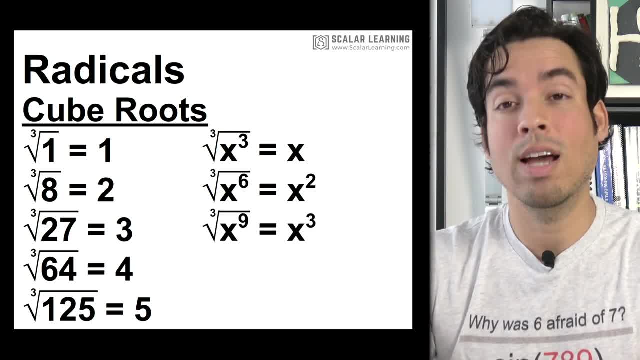 3 is 2,, 9 divided by 3 is 3, and if you're not sure if this is right, again always double check. what's x cubed times, x cubed times, x cubed? We add all three of. 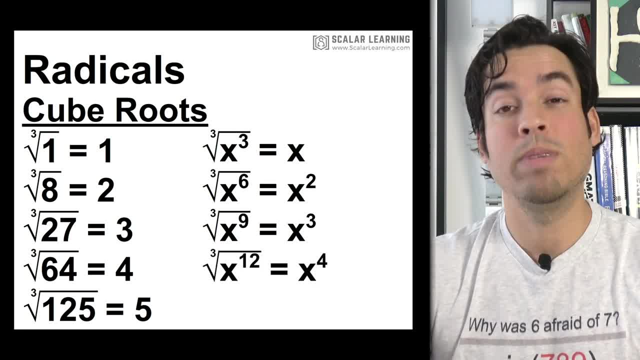 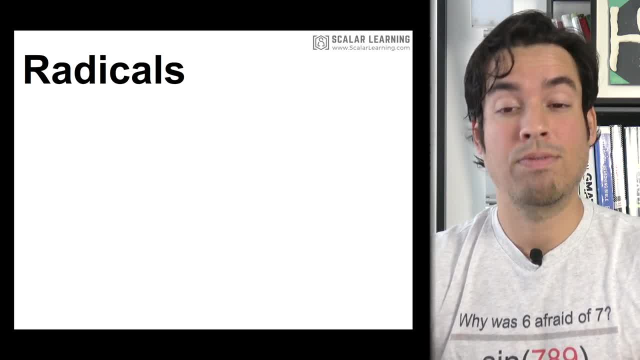 those exponents we get: x to the ninth, x to the twelfth would be x to the fourth and, last but not least, x to the fifteenth would be x to the fifth. Now let's talk about simplifying radicals, okay, and simplifying these roots. So here's a. 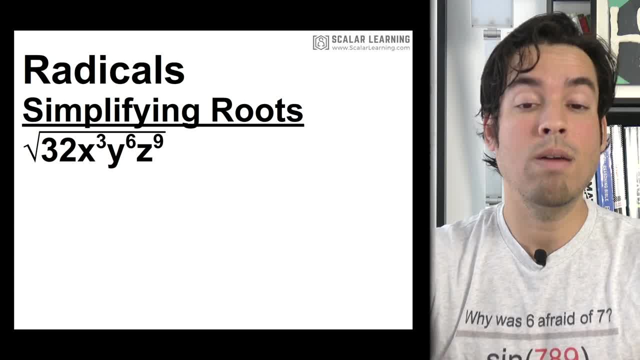 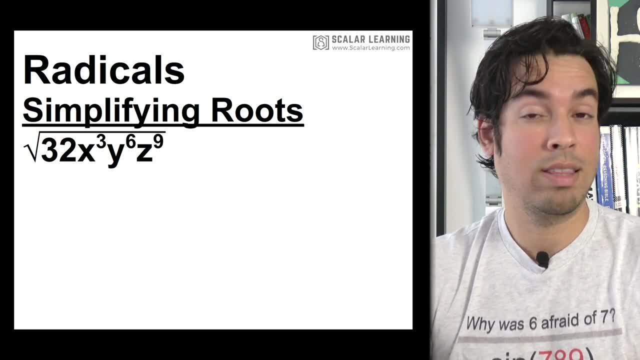 perfect example. we're going to start with the square root. Now you notice there's no number. When there's no number, you assume it's a 2, so it's just a square root. So how do we take the square root? This is my way of doing it and I 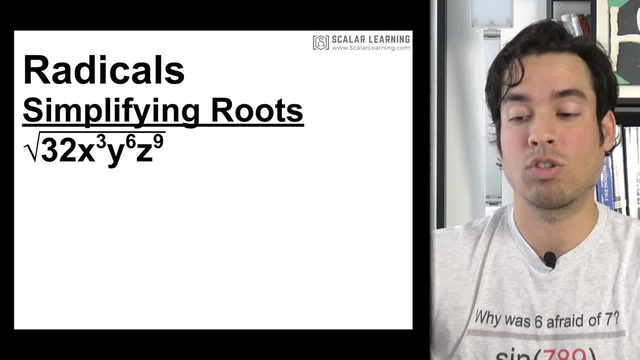 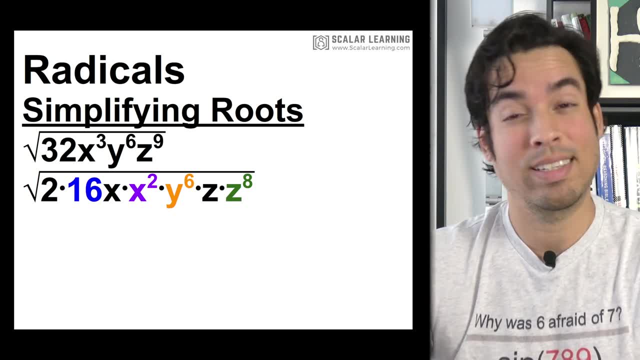 think it's really helpful. I like to break everything up into perfect squares. So, for example, I'm taking from that 32, I'm saying I'm representing that 32 as 2 times 16, because 16 is a perfect square. I'm taking that x cubed and I'm 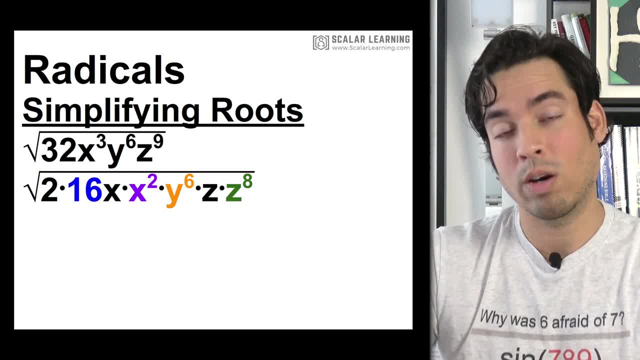 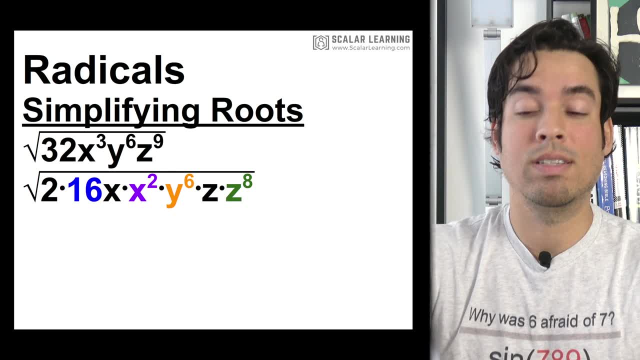 representing it as x times x squared, Because at least I've got one perfect square in there: x squared. Y sixth is already a perfect square because it's a nice even exponent. And then I'm taking that z and I'm breaking it up into z times z to the eighth, because z to the eighth is a perfect square. Okay. 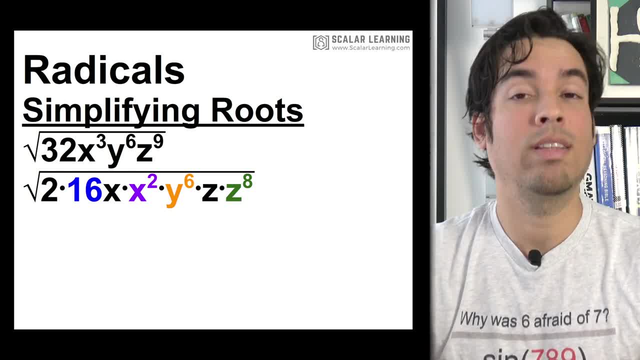 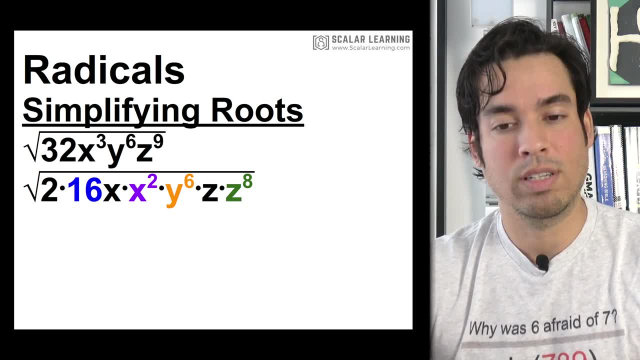 Why do I do this? Because I think of a square root as a prism. The only thing that can come out is perfect squares, and it comes out as the square root. So, for example, I can now take the square root of 16,, which is 4.. Beautiful. I can take the square root of x, squared, which. 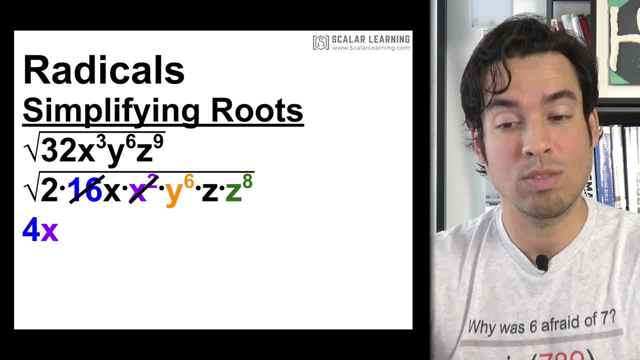 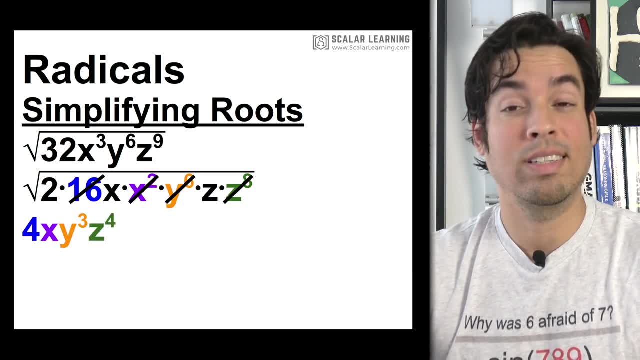 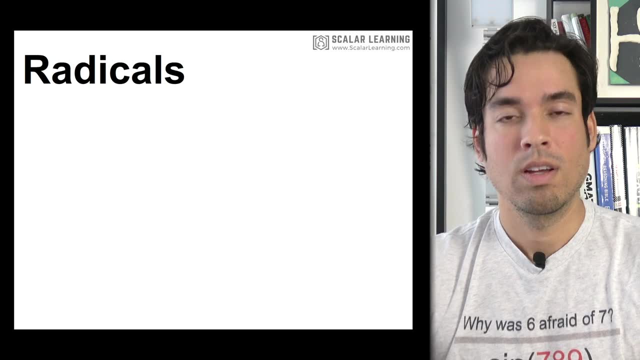 is x. I can take the square root of y to the sixth, which is y to the third, And I can take the square root of z to the eighth, which is z to the fourth. Everything else is stuck inside that square root prism, So the 2xz stays inside, and then we have it as fully simplified. 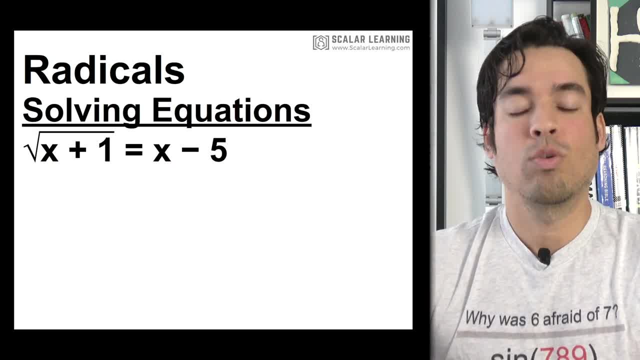 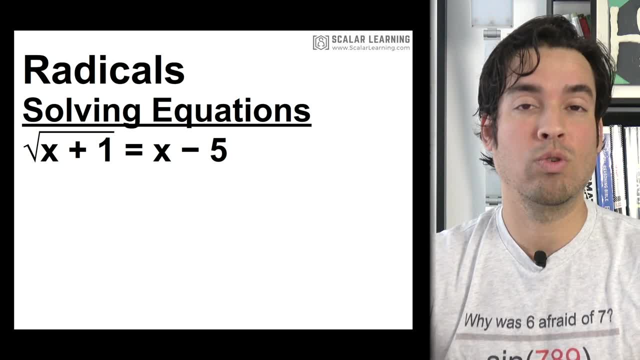 Now let's talk about solving equations involving radicals. So we start off with something like this: The square root of x plus 1 equals x minus 5.. Okay, Job number one is to get rid of that square root. How do we do that? 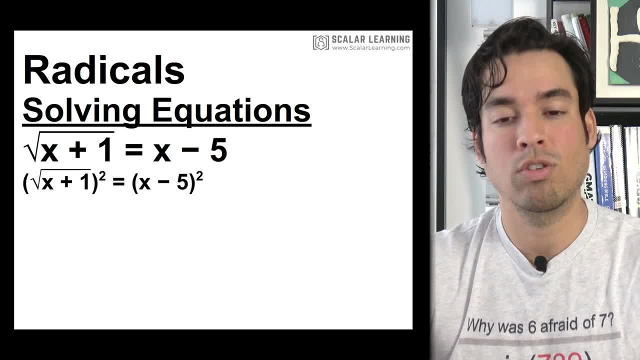 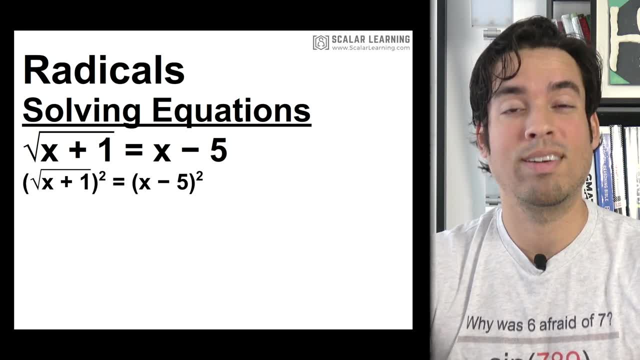 We do the inverse operation. We're going to do the inverse of what you did with the square root of x plus 1, which is squaring both sides Right. So you notice, I got to square the left side and the right side, But that right side is a binomial, So don't make it x squared plus 25.. Okay, It's. 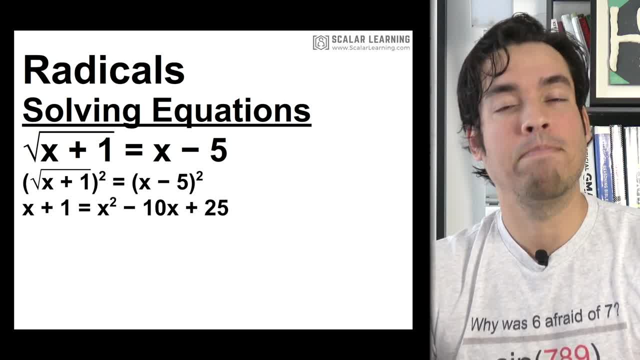 a big mistake. Instead, it's x minus 5 times x minus 5.. So you've got to FOIL right And we get x squared minus 10x plus 25.. And if you're not sure I did that, remember it's. 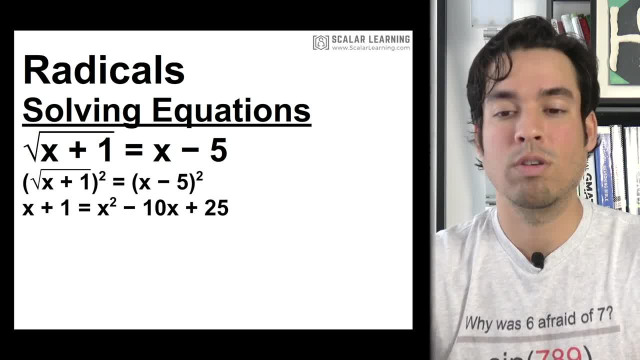 going to be x minus 5 times x minus 5.. And you've got to do that FOILing process and then you'll see you get x squared minus 10x plus 25.. to subtract x and subtract 1 from both sides, because I want to get 0 in this. 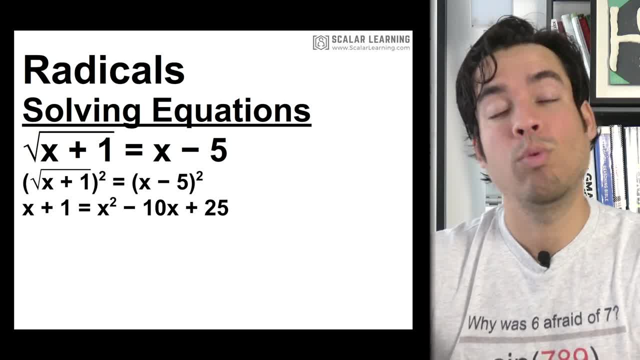 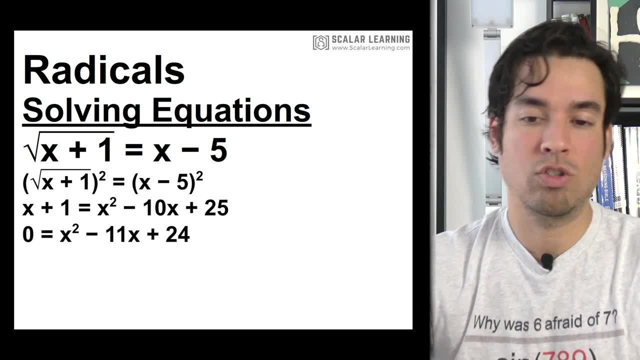 Anytime we're dealing with a quadratic, again, degree of 2, we want to get everything equal to 0.. So 10x negative, 10x minus x is negative 11x, and 25 minus 1 is 24.. So we got x squared minus 11x plus 24.. Now, if possible, I'd love to 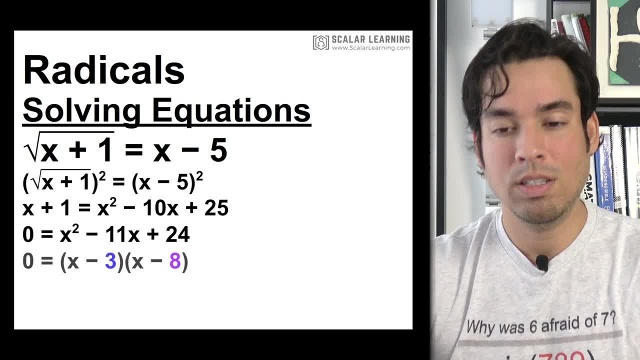 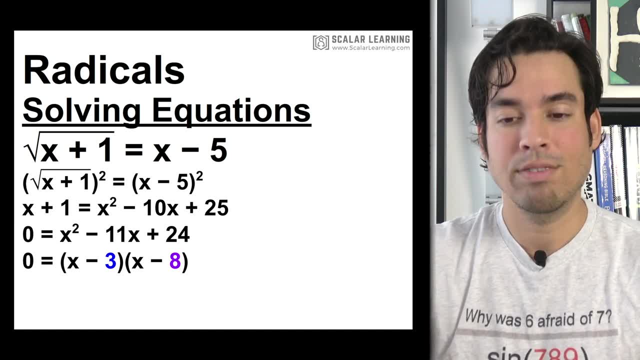 factor. If that doesn't work, of course we got the quadratic formula, But this is factorable. Again, we're asking the question: what multiplies to 24 and what adds to negative 11. That's negative 3 and negative 8.. So what are the zeros or? 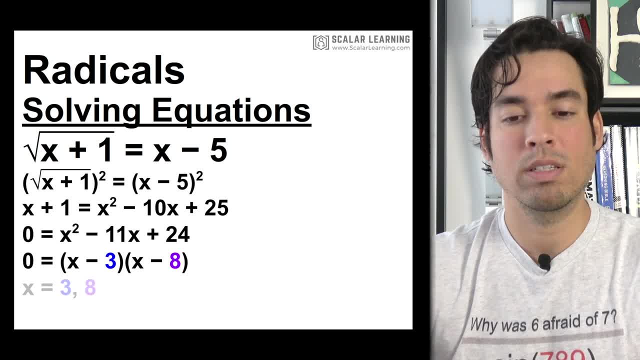 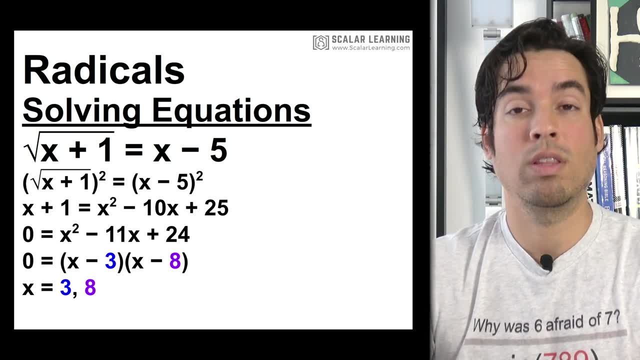 what are the solutions? What makes each binomial go to 0? It would be positive 3 and positive 8.. But there's a final step. with these radical equations, You've got to check both zeros to make sure they are legitimate solutions. they're. 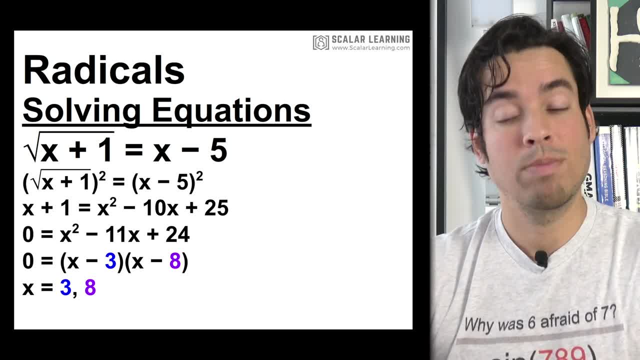 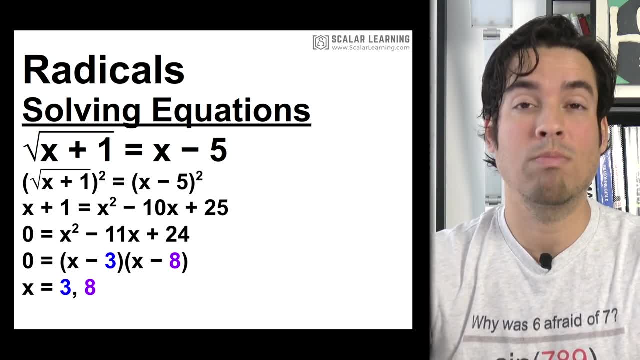 not extraneous solutions. So how do we do that? All right, we're going to plug them into our original equation. And notice: here now we're only talking about the positive roots, not the negative roots. Remember what we said before: square root of 4. 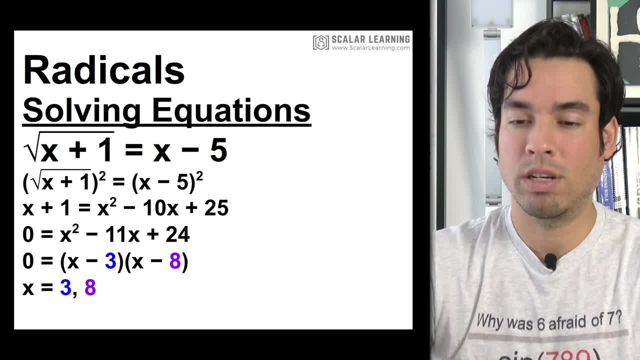 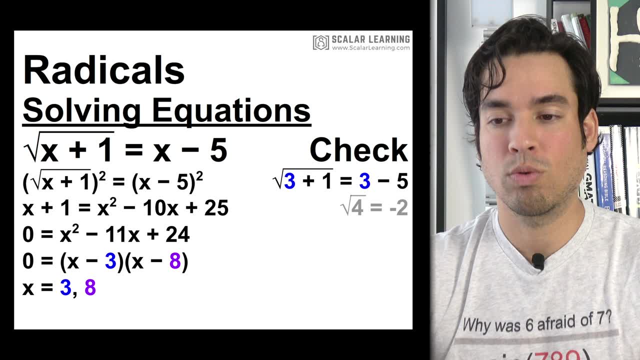 at both two and negative two. We're only taking the positive one here. So first let's check that three value. So you notice I'm plugging three in for x. So three plus one on the left side gives us the square root of four. 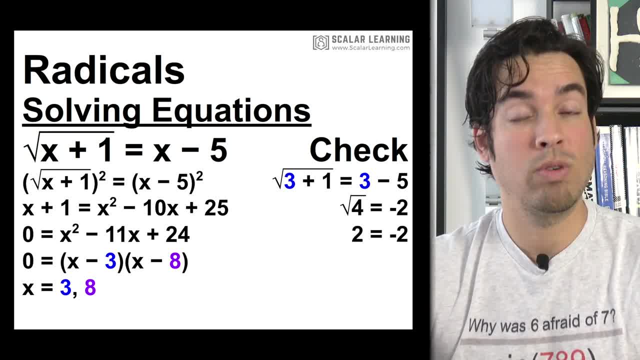 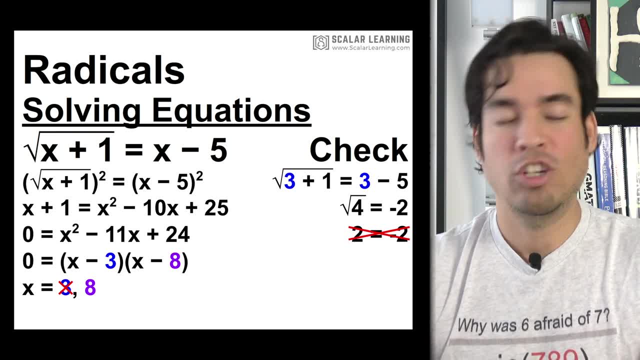 On the right side we get negative two. Square root of four is positive two. Again, we're only taking the positive root. in this case, Two does not equal negative two. therefore, three is extraneous. Now, chances are if one's extraneous. 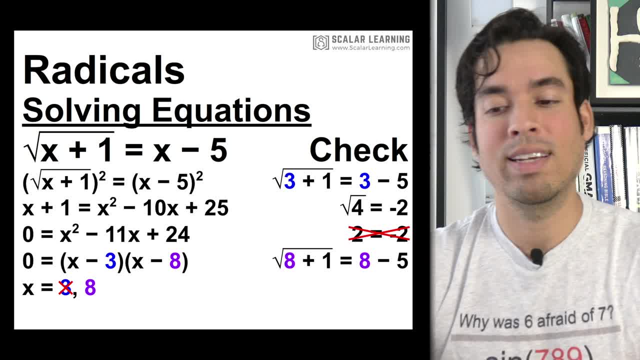 the other one's probably gonna be legitimate, but we have to check anyway. So now I'm plugging in the eight. I get eight plus one on the left side, eight minus five on the right. That becomes the square root of nine equals three. 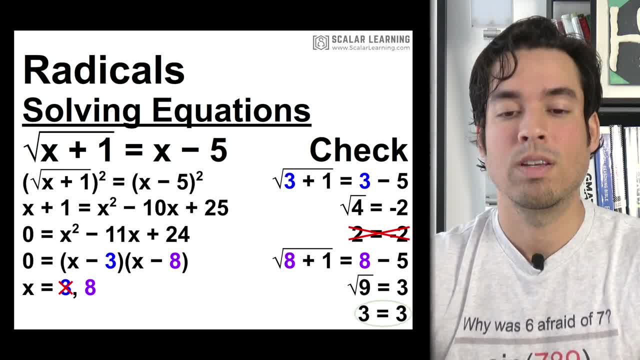 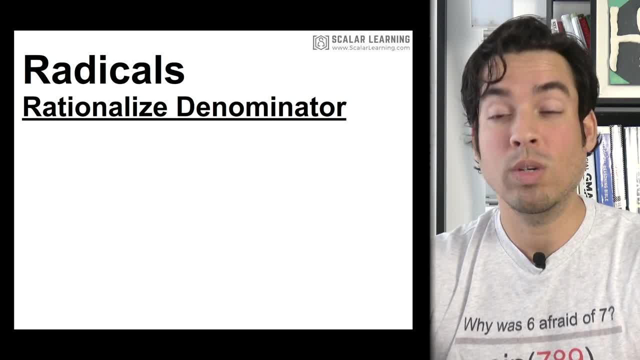 And guess what? Square root of nine is positive three. in this case, That solution is valid. Something else we might come across with radicals is rationalizing denominators. What does this mean? It means that if I take a radical like three over square root of five. 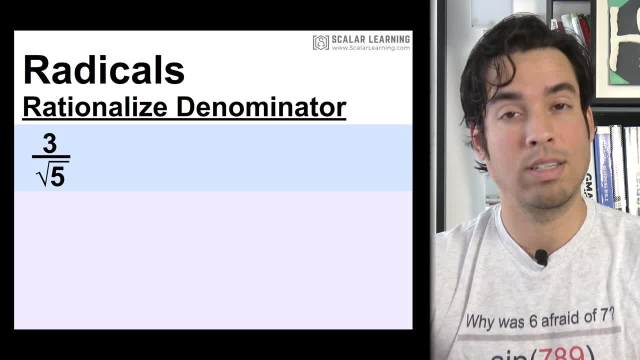 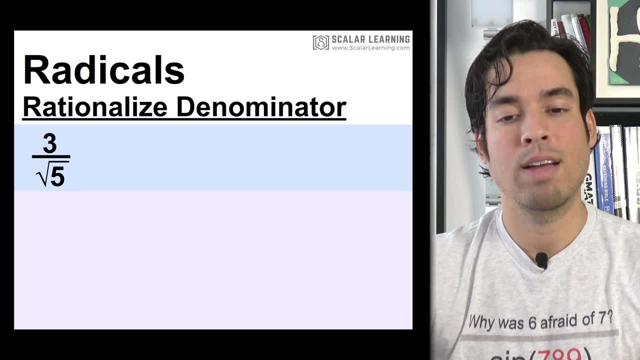 we have a rule in mathematics that we don't want to have a radical in the denominator. It's just something you have to become familiar with. It's a formatting thing, almost syntax. So we see a square root of five in the denominator. 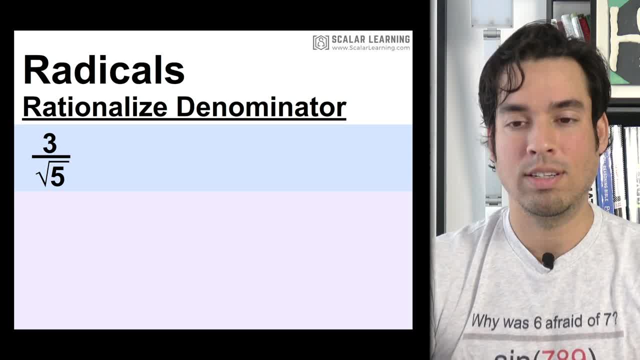 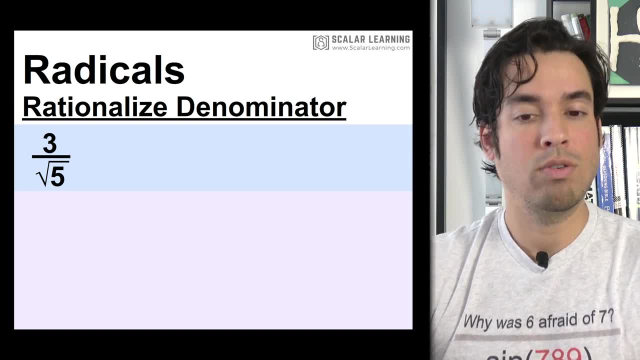 Chances are that the answer choice is not gonna have a radical in the denominator. So we must rationalize the denominator, Believe it or not. this is actually pretty simple, because I can obliterate that square root five simply by multiplying it by square root of five. 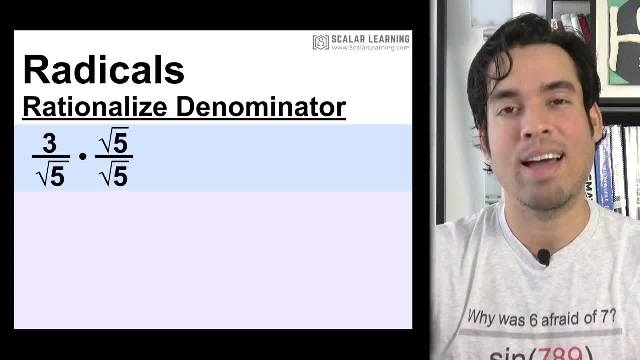 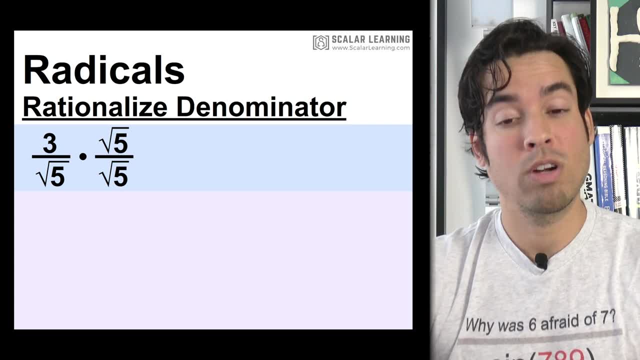 But again, I can't just multiply the denominator, right, I have to also multiply the numerator by the same value, Otherwise I'm changing the value of the fraction. So I multiply top and bottom by square root of five. The nice part about. 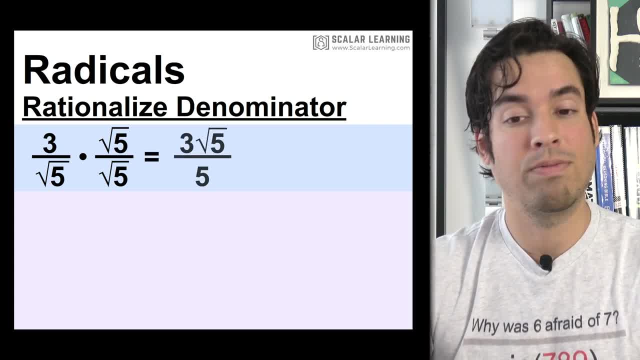 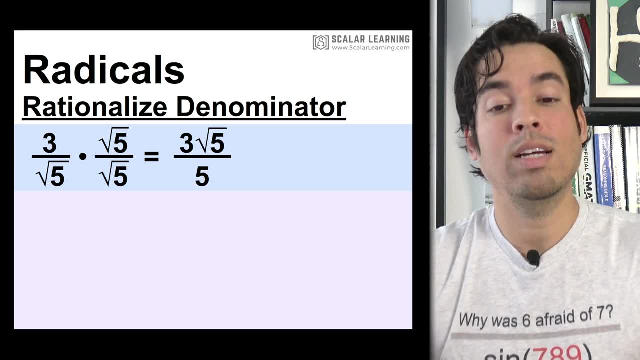 square root of five times square root of five on the denominator is it's simply five. And then top we get three radical five. So now we've rationalized the denominator. This is the proper format. So a lot of times when they say, to simplify, 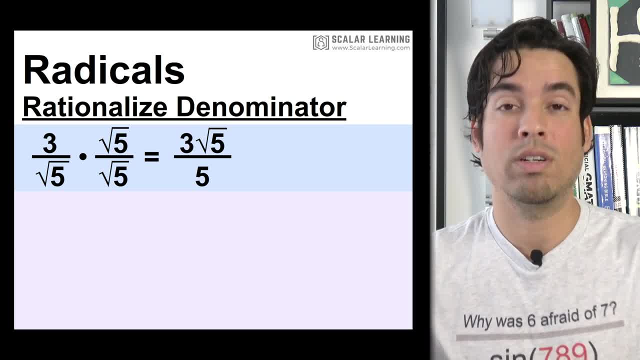 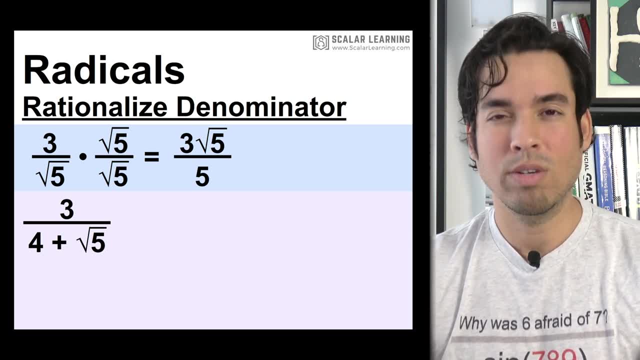 an expression with a radical. all they're asking you to do is get rid of that radical in the denominator. Let's take a more complex example where we have three over four plus square root of five. Now it's not so easy, because if I just multiply it by root, five over root five. 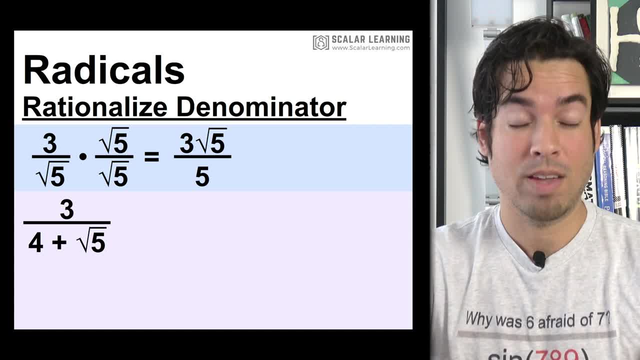 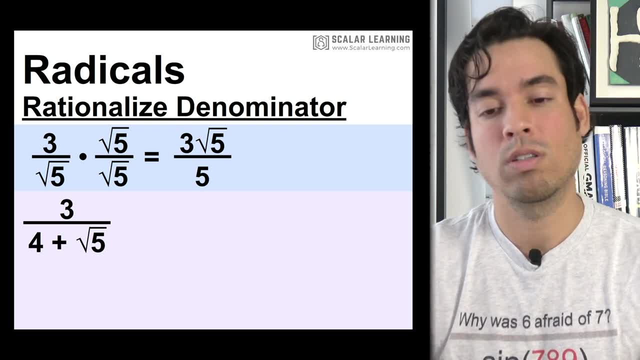 the problem on the bottom is that root five is going to distribute and I'm going to get four root five plus five. It's no good because I still got a radical. Now we have to be a little smarter and we have to use something called the conjugate. 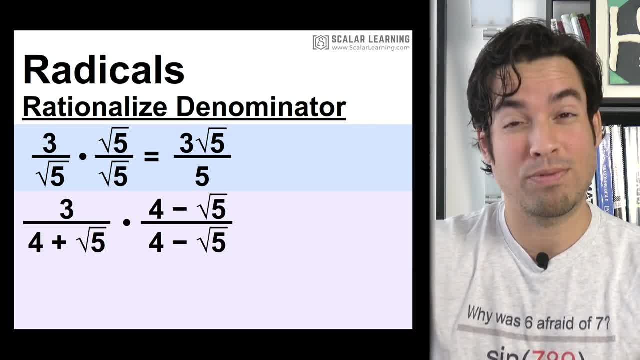 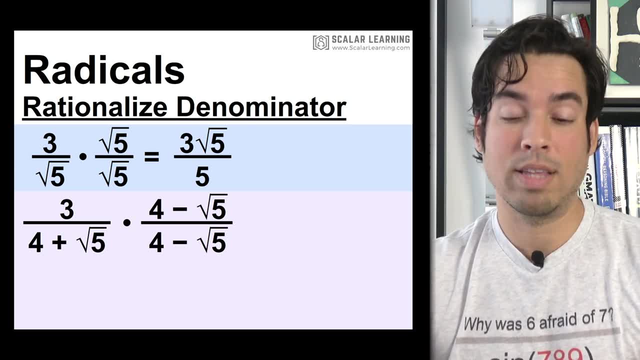 So it's the same thing as four plus radical five, except we just flip the plus to a negative. If it was a minus, we'd flip it to a positive, So we just make it opposite. Okay, again, now we FOIL that denominator. 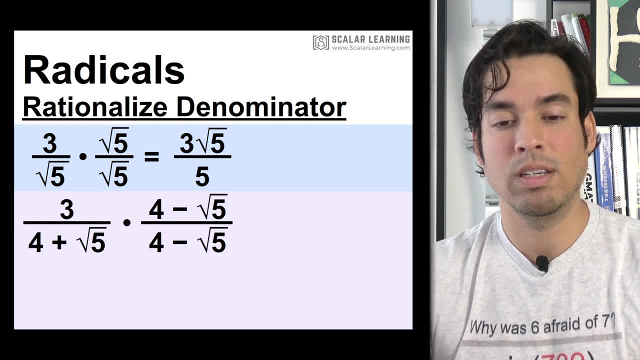 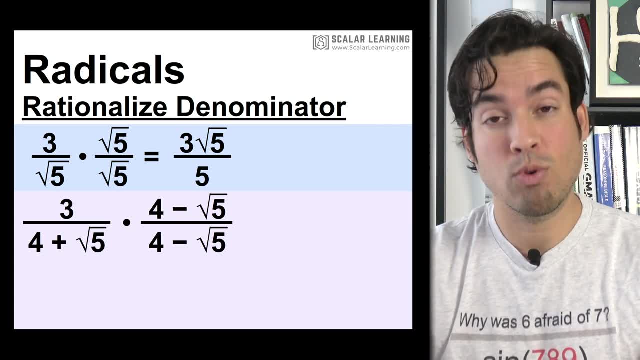 but you don't even really have to FOIL, because it works out perfectly so that the middle terms cancel out, Because what you get is 16, minus four radical five plus four. radical five minus five. But the middle terms cancel out because they're opposite. 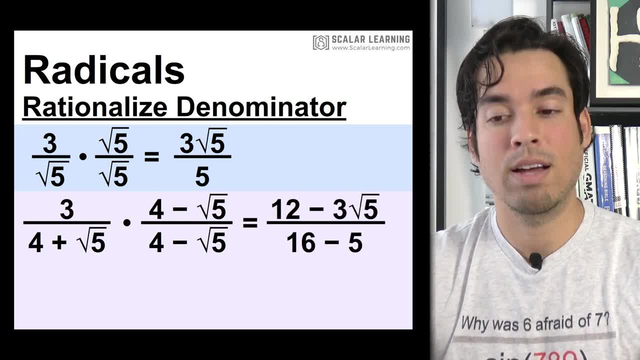 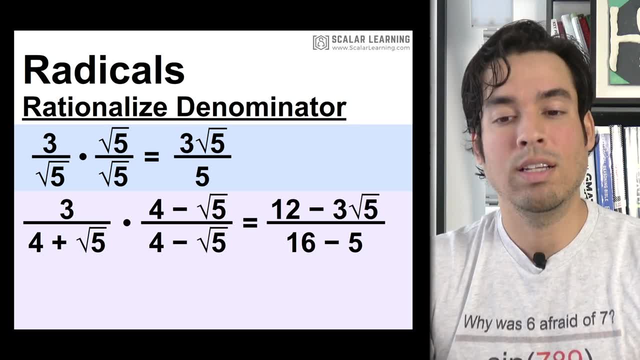 So all we get is 16 minus five on the bottom. So super nice, right. And again, radical five times radical five just turns into a five, but there's a minus there, so it's negative. And on the top, we just distributed the three. 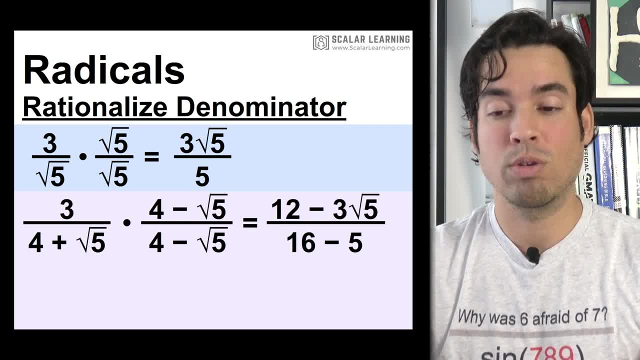 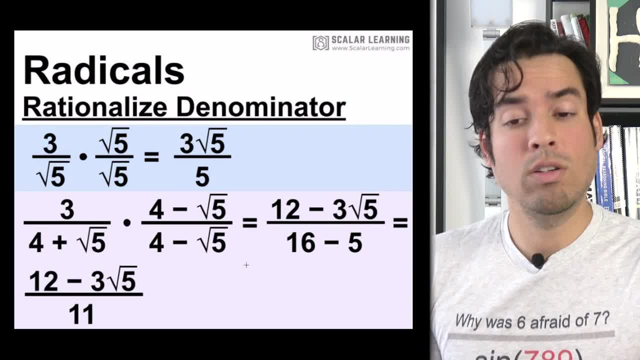 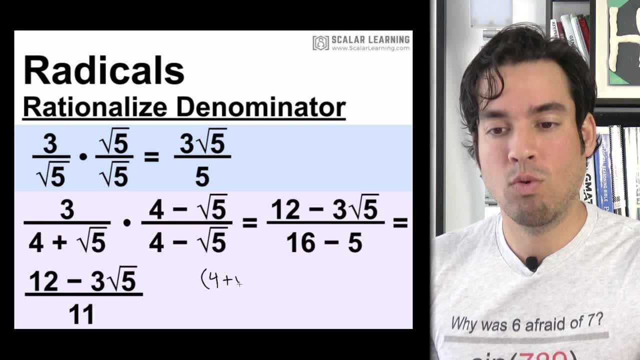 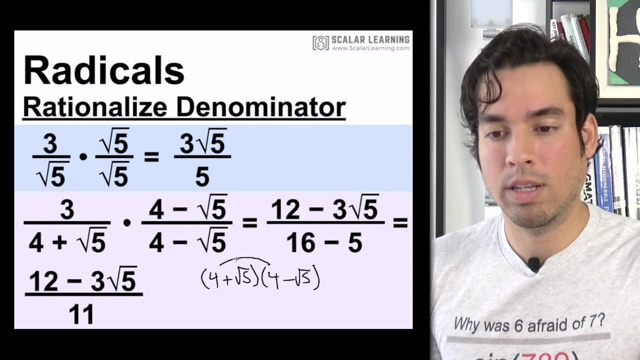 nice fraction with a rational denominator. Just as a little explanation of how this times this gives me this, let me just show you how it would FOIL. We'd have four plus square root five times four minus square root five. This would FOIL like that and like that. 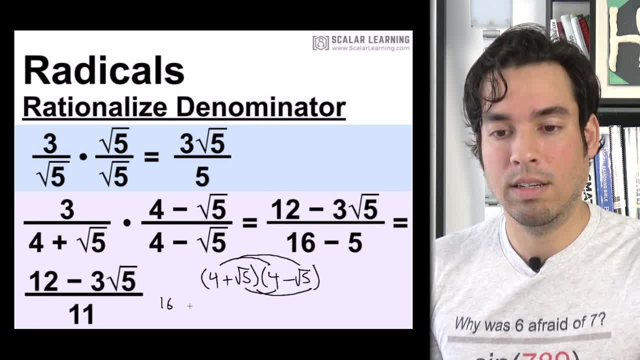 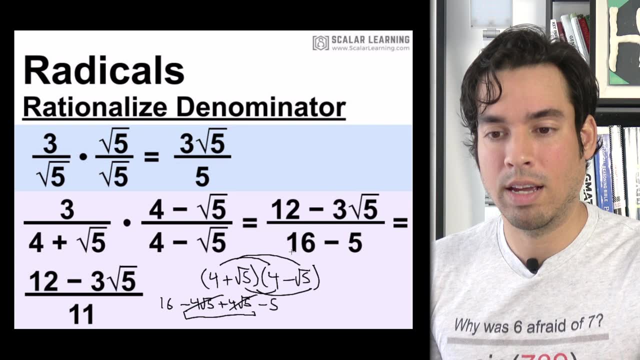 So what do we get? We get 16 minus four rad five plus four rad five. five times negative rad five is just negative five. The square roots go away. These guys are opposite. They cancel, and hence we're left with 16 minus five. 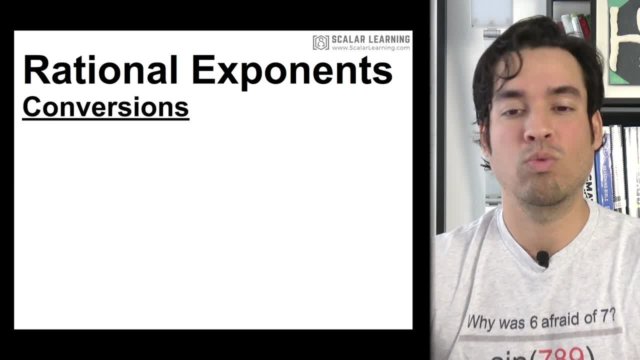 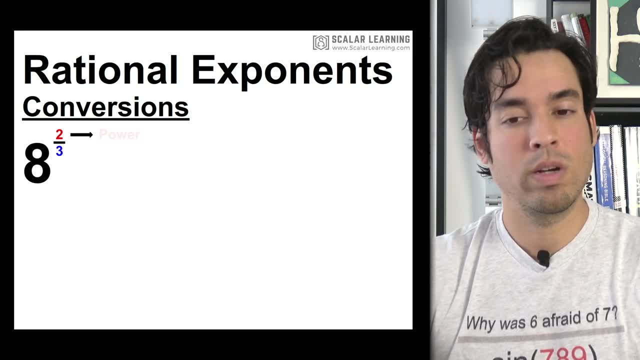 Now we're gonna talk about rational exponents, a little bit of exponent rules. So check it out. If I have a to the two thirds power, what does that mean? Well, we look at the numerator always as the power and the denominator as the root. 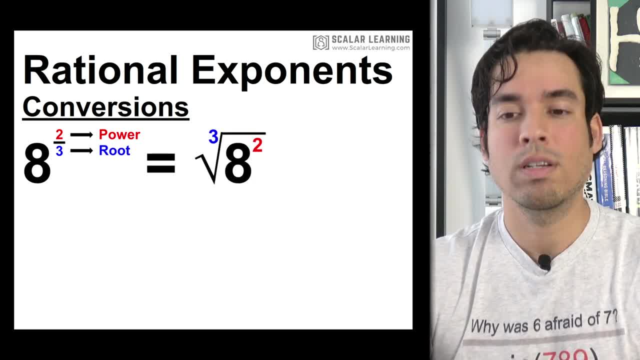 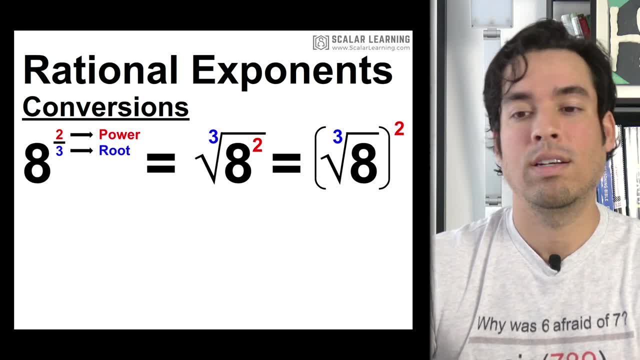 So how can I rewrite this as a radical? Okay, it's super nice. I can say that it's eight squared and the cube root of that. I can also write it in the opposite way, where I can take the cube root of eight first. 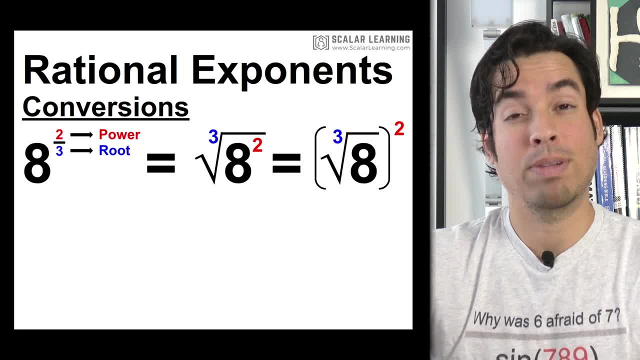 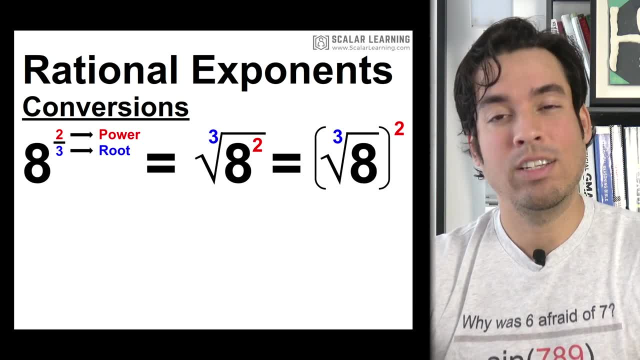 and then square it afterwards, which means that the order in which I apply these exponents- whether it's a root or a power, it doesn't matter, We're gonna get the same answer, and I'm gonna show you now why. So first we do that: eight squared, which gives us 64.. 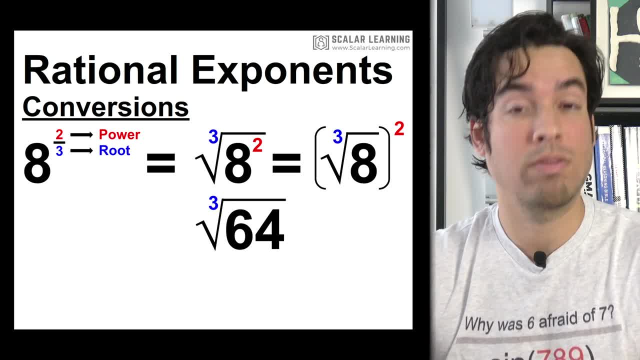 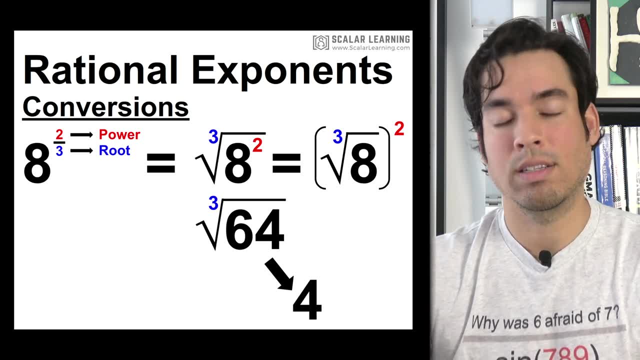 What's the cube root of 64, meaning what number times itself and then times itself again? is 64?? That's four. What about if we go to the right side? first, What's the cubic root of eight? It's four, And then what's two? 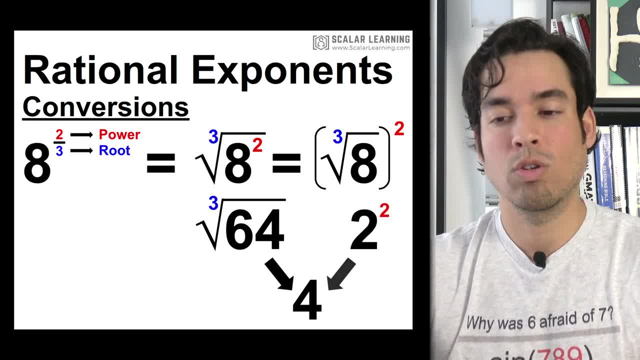 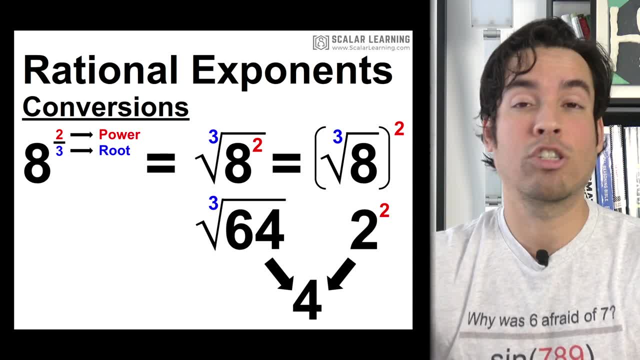 Because two times two times two is eight, And then what's two squared, It's also four. So notice, you get the same thing both ways, And I usually prefer the method on the right because I like to go small, then big, not really big. 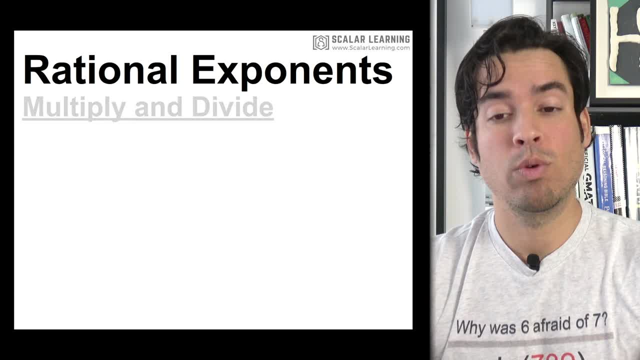 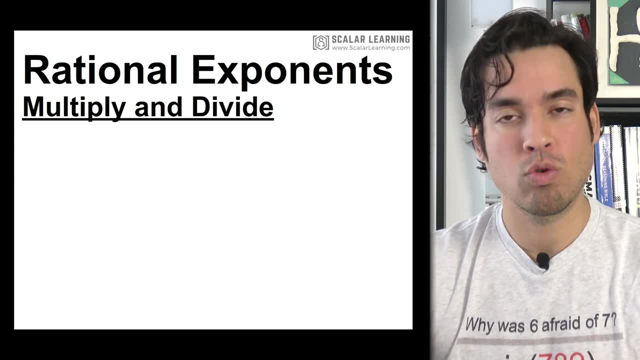 and then have to come back and go small, It's usually easier. Another quick rule that we want to be aware of is when we multiply and divide involving exponents. So, really quickly, I'm gonna give you two short examples that are tested quite frequently. 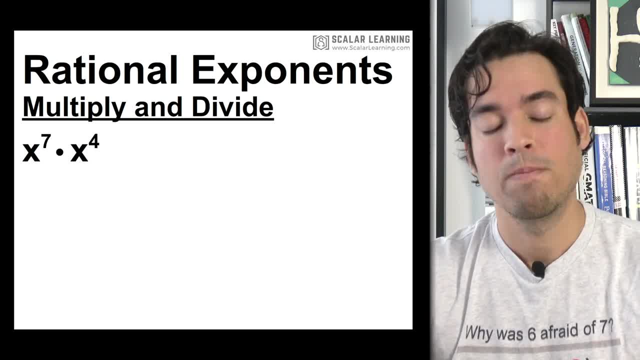 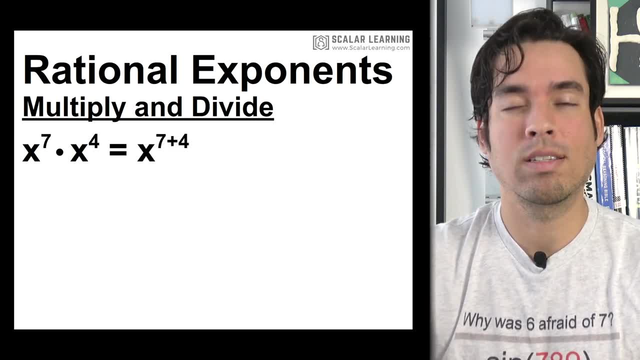 So remember, let's say, I've got the same base, has to be the same base. So we got the same base of x and I've got x to the seventh times, x to the fourth. What does that equal? That equals the sum of those exponents. 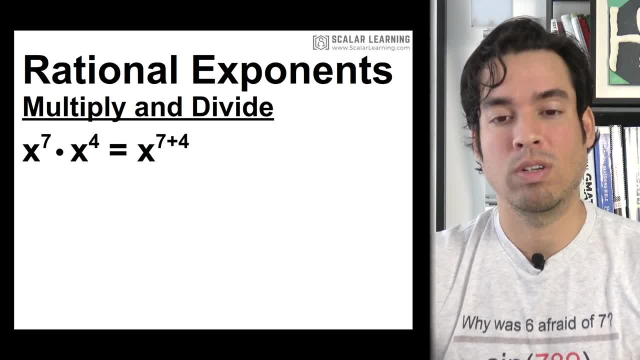 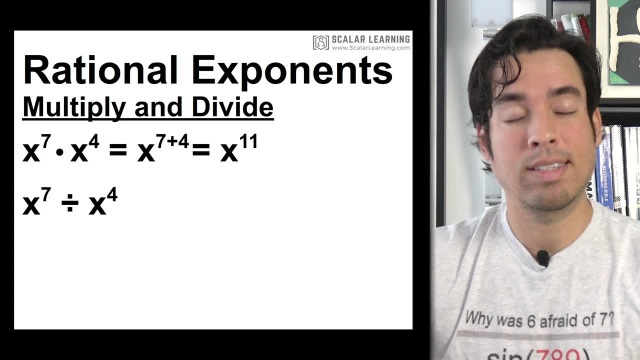 So when we multiply, we're really adding the exponents, So it becomes seven plus four, which is x to the 11th. What about when we divide? So let's say now we got the same thing: x to the seventh divided by x to the fourth. 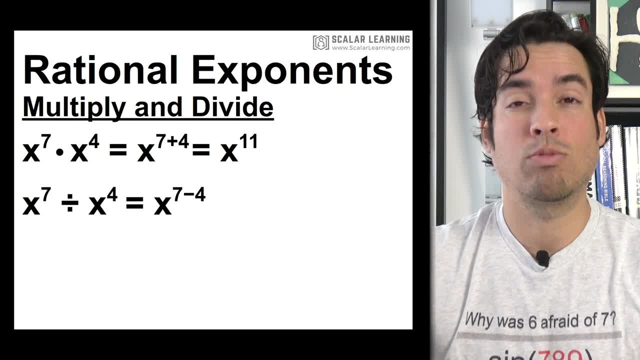 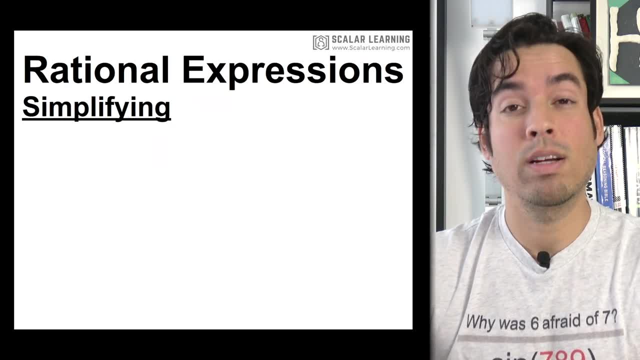 Again, it has to have the same base. And now, instead of adding, we subtract the exponents, So it's seven minus four, which equals x to the third power. Next, we're gonna talk about simplifying rational expression. So I'm gonna give you an example of a rational expression. 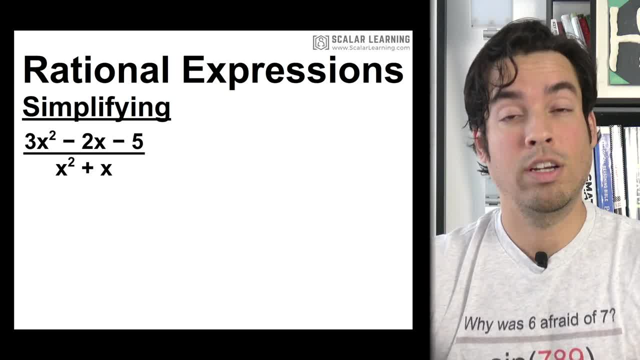 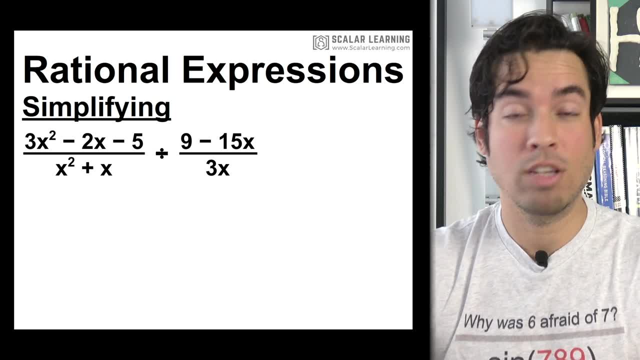 which is basically a fraction of expressions. So we got this one here, but then let's make it more complicated. We're dividing by this other crazy rational expression, All right, so there are a couple of steps that you just gotta follow, no matter what. 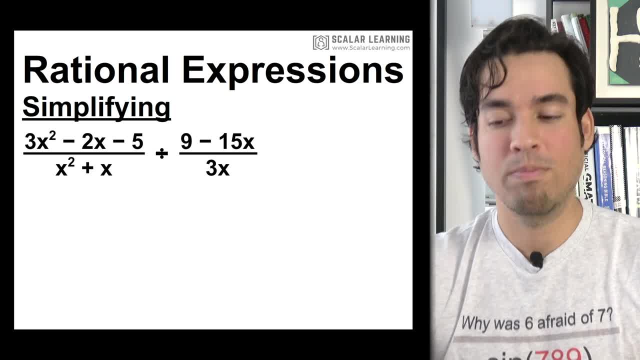 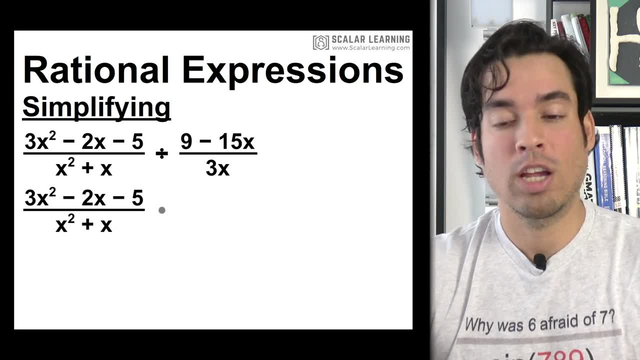 First of all, when we're dividing. we don't wanna do that, We wanna immediately shift that to multiplication. So we employ: keep, change, flip. I keep the first rational expression, I change that to multiplication and I flip the other one to 3x over nine minus 15x. 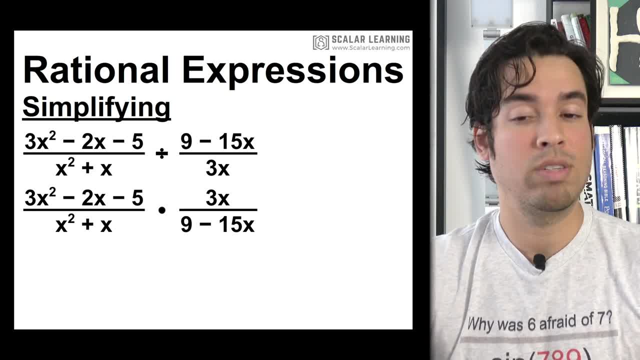 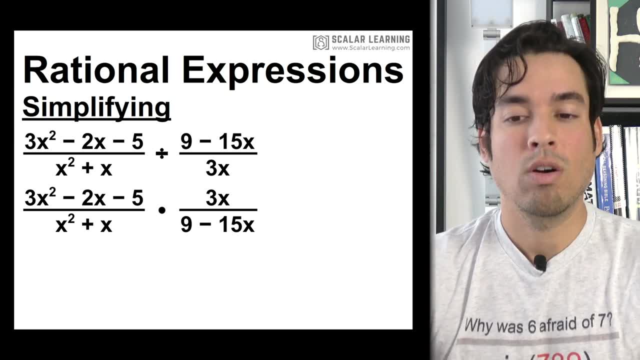 Then we go into a rule that I advise to everybody, that when you see a quadratic like this and you're not sure what to do, simply factor. So now I'm gonna start factoring everything, So we're gonna factor all these expressions. 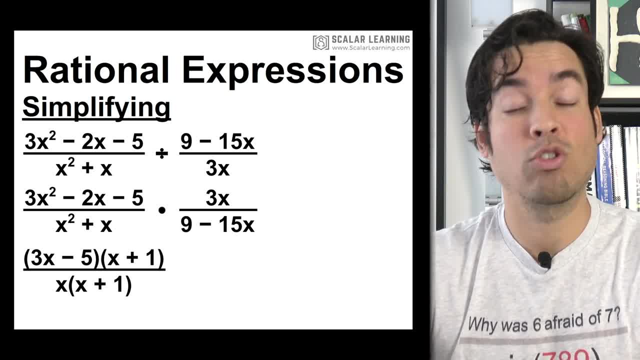 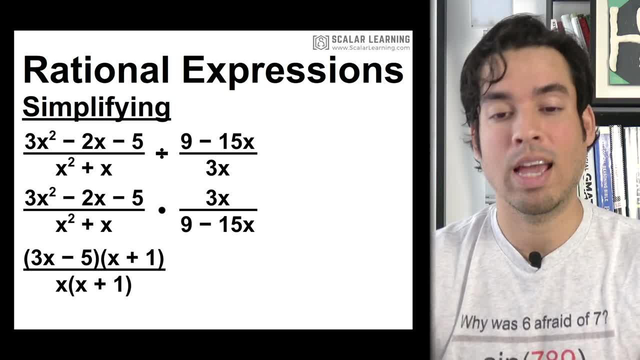 So on the left, the 3x squared minus 2x minus five factors to 3x minus five times x plus one. On the bottom we factor out an x and it's just simply x times x plus one. On the right, 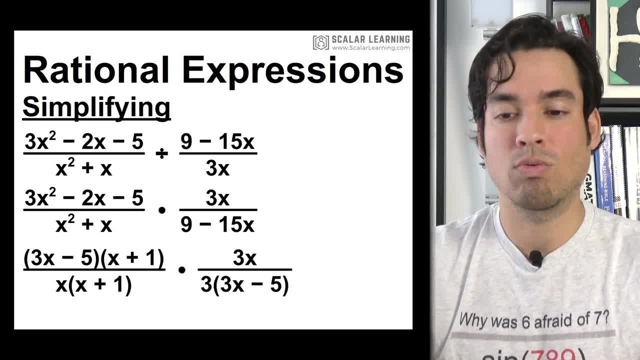 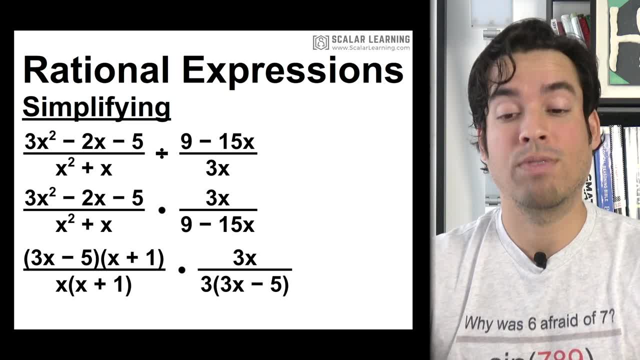 the top. we can't do anything but the bottom. we can factor out a three and it's three times 3x minus five. Now it's almost like one giant fraction because it's all multiplying, So the numerators and the denominators kind of combine. 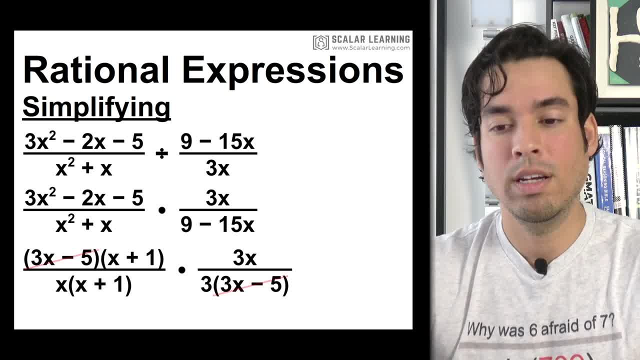 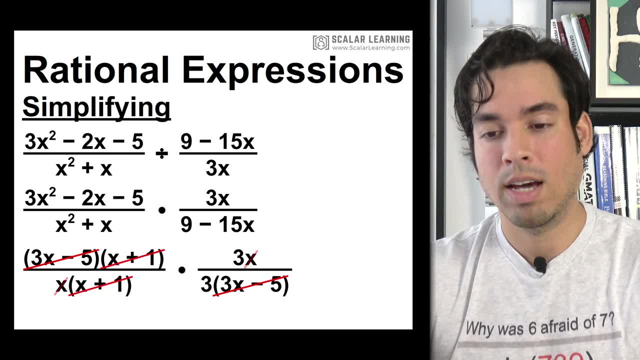 which gives us a great opportunity to cross cancel. So I see I've got those 3x minus fives that I can just knock out. I've also got x plus ones on the top and bottom that I can knock out. I've got a x on the top and bottom. 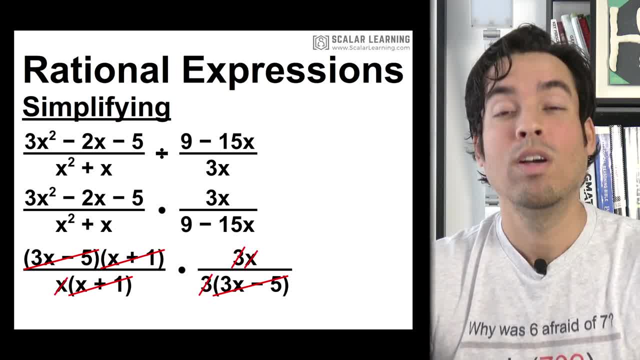 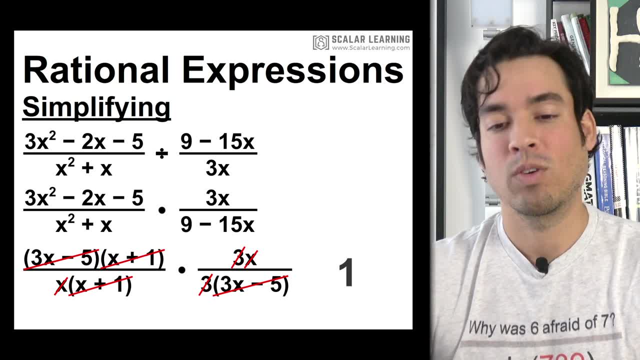 that also can get knocked out, And also those threes: knock out, knockout. What happens when everything knocks out? When everything knocks out, you don't have zero, by the way, you have a one, okay. So everything on top is equal to everything on bottom, It's just. 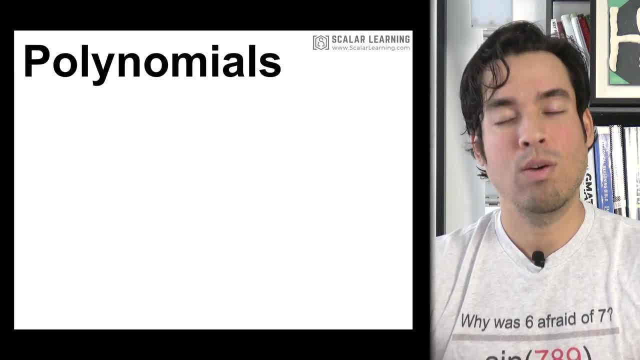 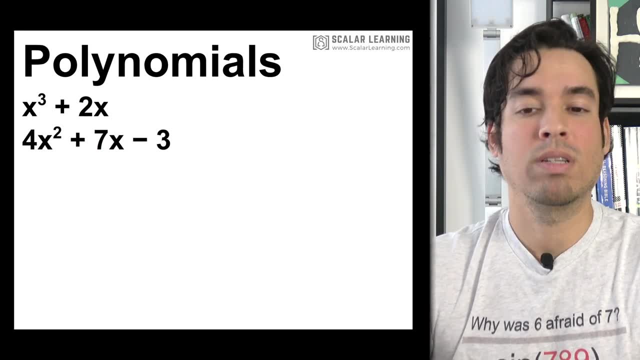 like five divided by five or 10 divided by 10.. It's one. Now we're going to talk about polynomials. What's a polynomial? This is a polynomial: x cubed plus 2x, 4x squared plus 7x minus 3.. That's. 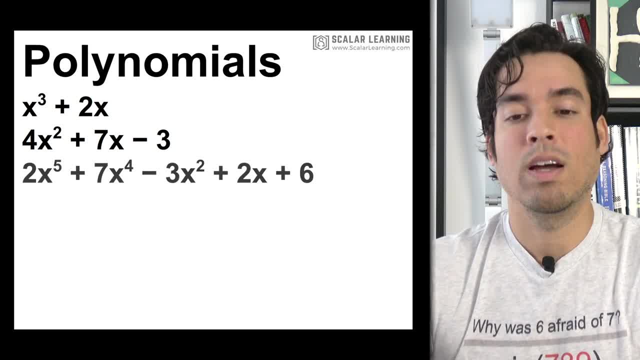 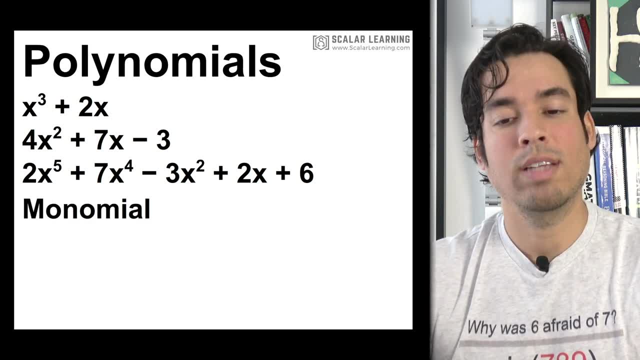 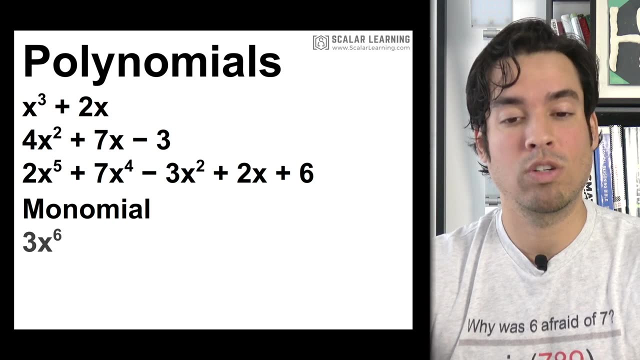 a polynomial. Poly meaning multiple terms. okay, This is a polynomial. This has five terms, right, And a degree of five, because the highest exponent is five. Okay, what is a monomial? Not so much that you need to know these names per se, but a monomial is, again, not many, but simply one term. 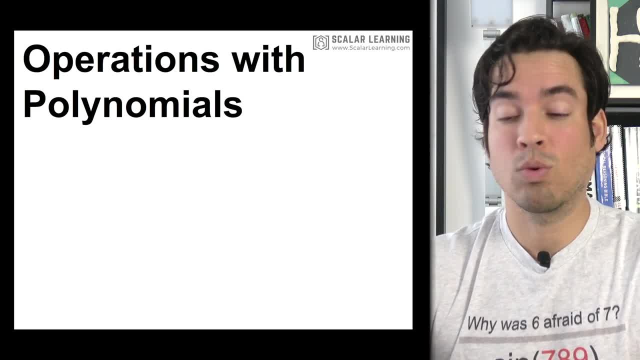 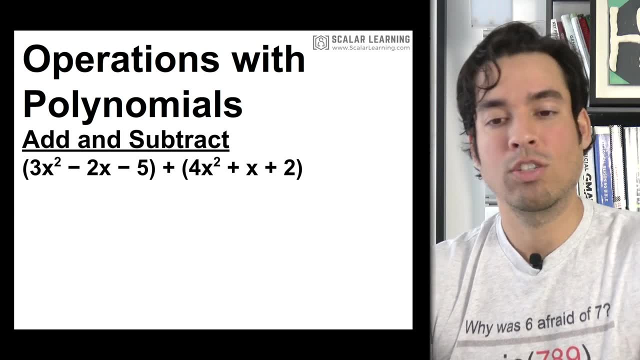 like 3x to the sixth. Now let's talk about operations with polynomials. So again, adding and subtracting is pretty straightforward. So let's take this example: We've got 3x squared minus 2x minus 5 plus 4x squared plus x plus 2.. The first thing you see is that they are in. 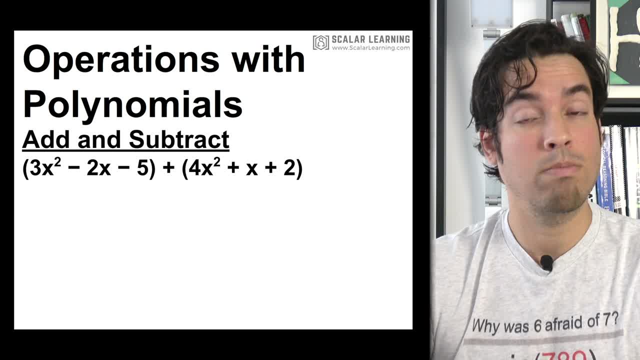 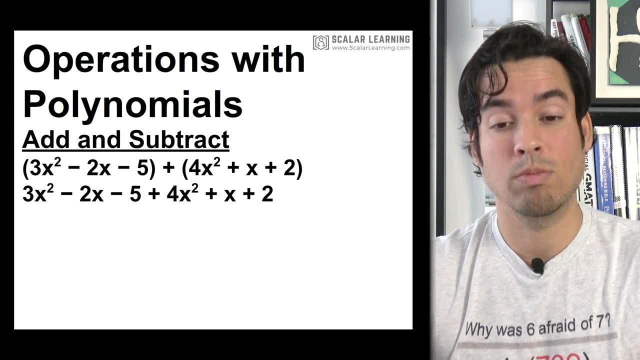 parentheses. but are the parentheses doing anything? No, there's nothing out there. multiplying, There's no minus sign. So I'm just going to get rid of those parentheses. And now I combine like terms. So you notice we have the x squareds, right, Those. 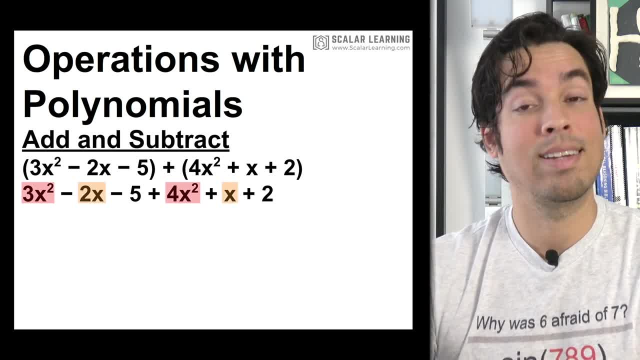 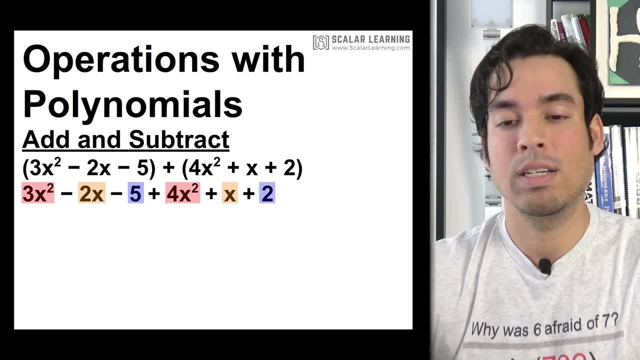 are like terms. We have the just simple x's, And again that's a negative 2x- Don't forget that minus. And then we got the 5 and the 2,, but again a negative 5 and 2.. Now we combine So the 3x. 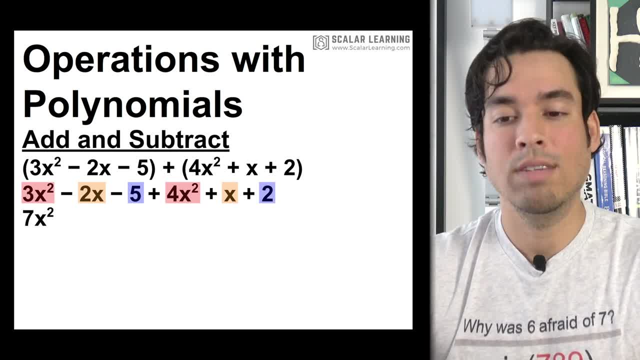 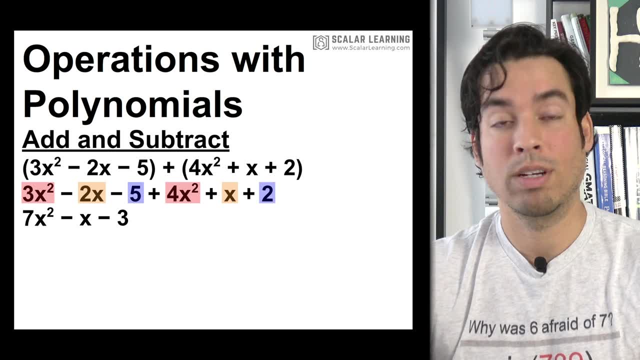 squared and the 4x squared becomes 7x squared. Negative 2x and positive 1x becomes negative 2x, And negative 5 and positive 2 combine to become negative 3. And that's that. Well, what about if we had a subtraction going on here? Okay, So now. 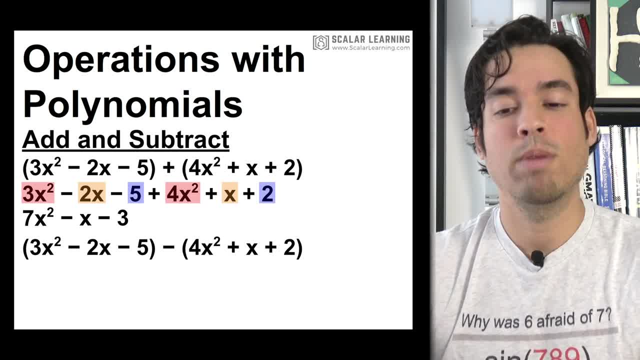 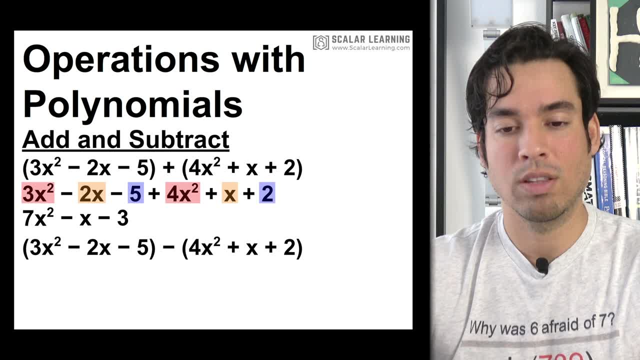 we can't just get rid of the parentheses so easily. We have to remember that on the right side that's really like a negative 1. So we have to distribute that minus across those three terms on the right. So now we have the same thing. on the left, We have minus 4x squared. 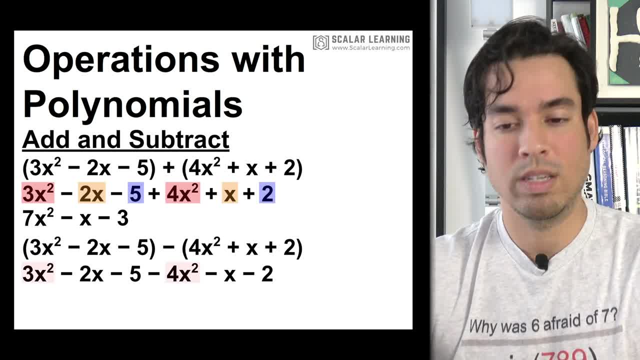 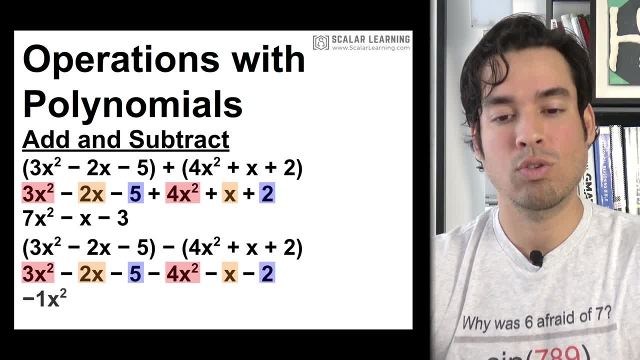 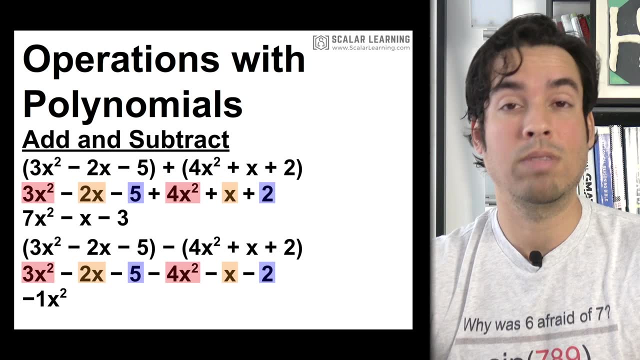 minus x, minus 2.. Again, let's identify the like terms with the x squareds, the x's and and the constants. 3x squared minus 4x squared is negative x squared And I put the 1 there, you don't have to- but it is negative 1x squared, The negative 2x and negative x, both same team. 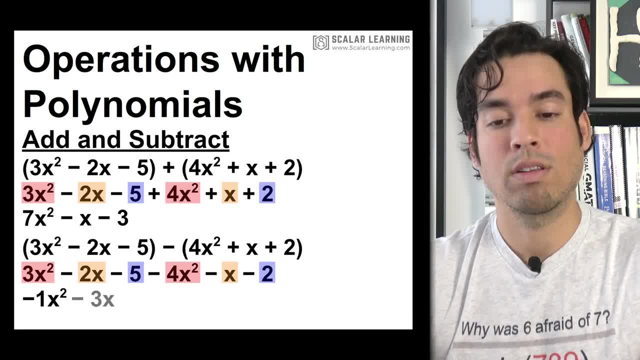 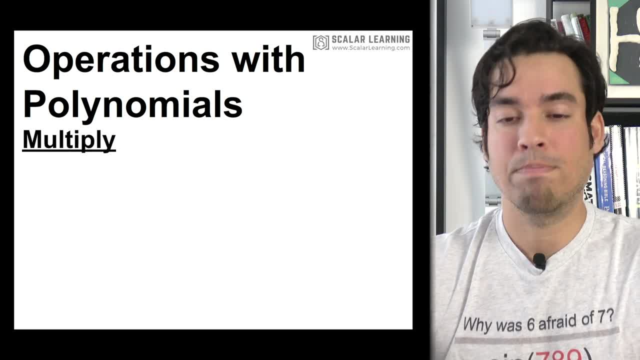 both negatives. So we got negative 3x And, last but not least, negative 5 and negative 2 make negative 7.. Now let's talk about multiplying polynomials. So we've got 2x minus 5 times 4x. 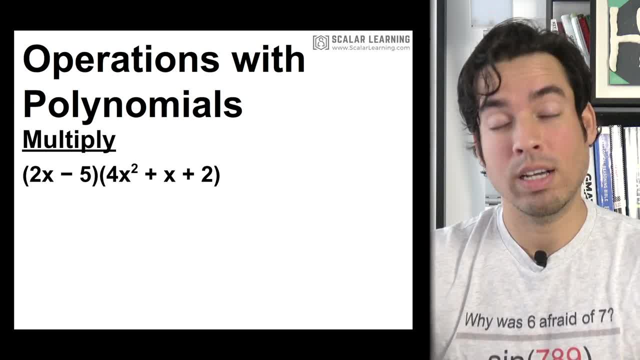 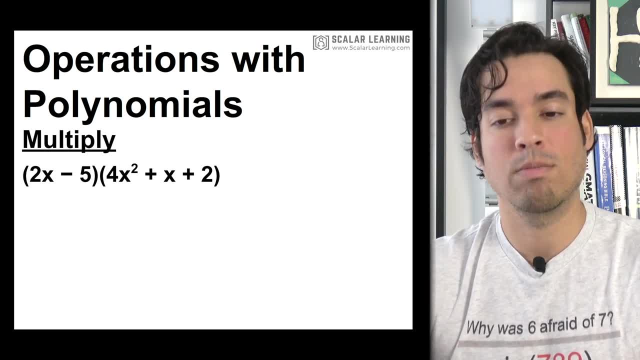 squared plus x plus 2.. Again, we're sort of doing the foiling operation. So if you guys have questions about that, this is how it works. Very straightforward. Essentially, everything in the first one has to multiply at some point everything in the second one, And this is a nice order to go. 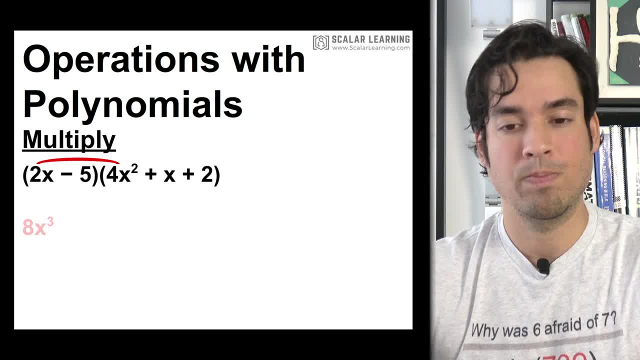 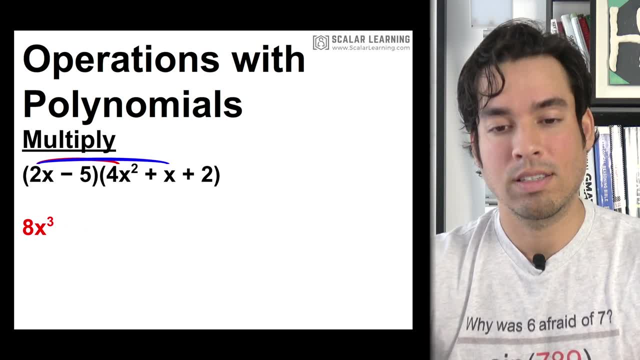 in. So first I do 2x times 4x squared, which gives me a nice 8x cubed. Again the exponents are being added And that x is also x to the first. 2x times x gives me 2x squared, And then 2x times 2 gives. 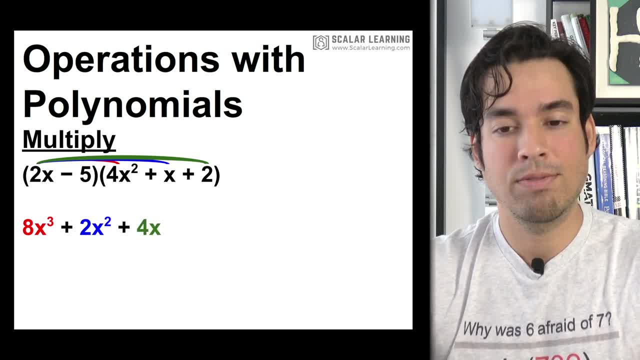 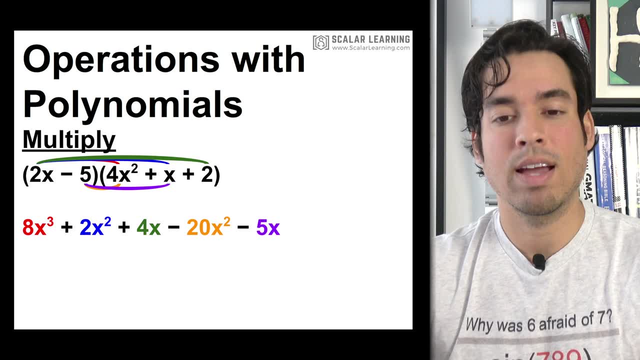 me a nice 4x. Now we start with the negative 5.. And we say negative 5 times everything. Negative 5 times 4x squared is negative. 20x squared Negative 5 times x is negative. 5x And, last but not least, negative. 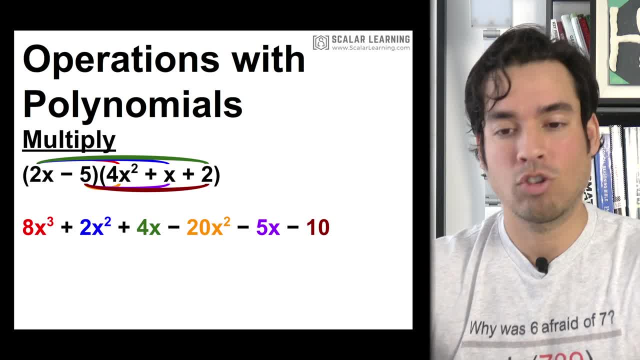 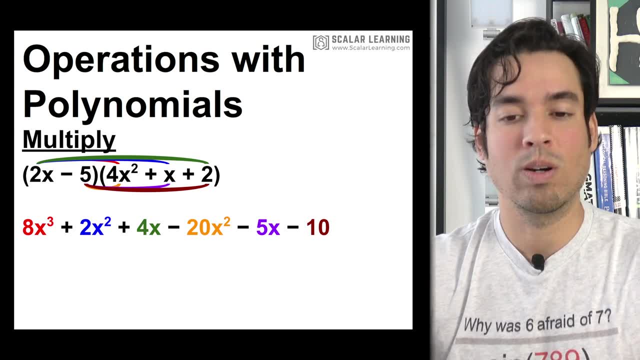 5 times 2 is negative 10.. Now if we have any like terms, we should combine And I see 2x squared and 2x's. So 2x squared plus negative 20x squared is going to give me negative 18x squared And 4x. 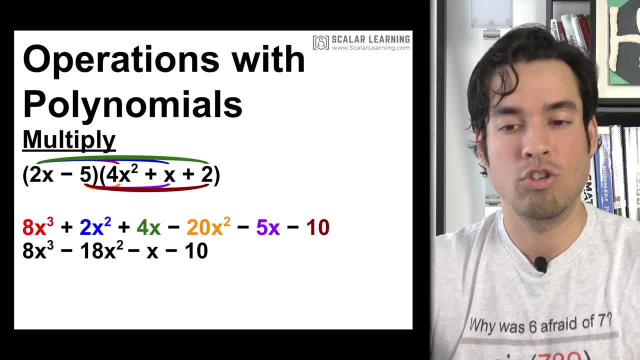 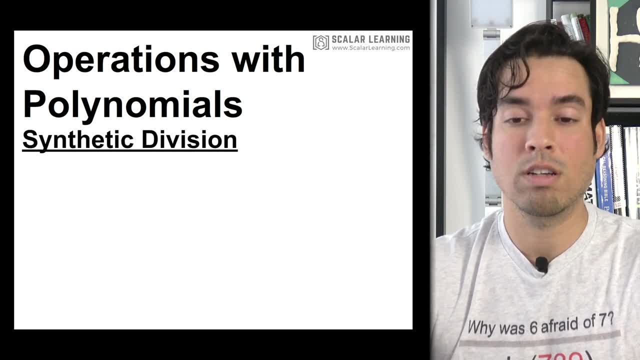 plus that negative 5x gives me a negative x, The 8x cubed and the negative 10 stay as they are. Next, let's talk about synthetic division, which does come up- not super often, but it does come up. 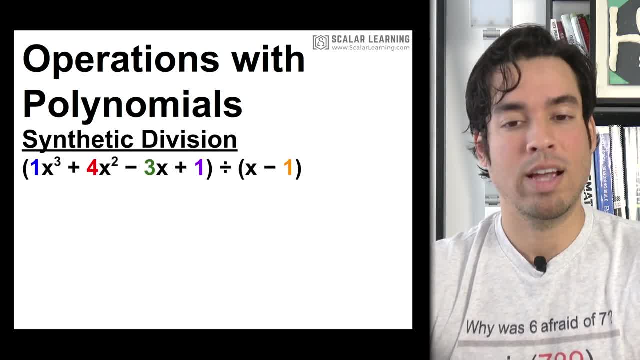 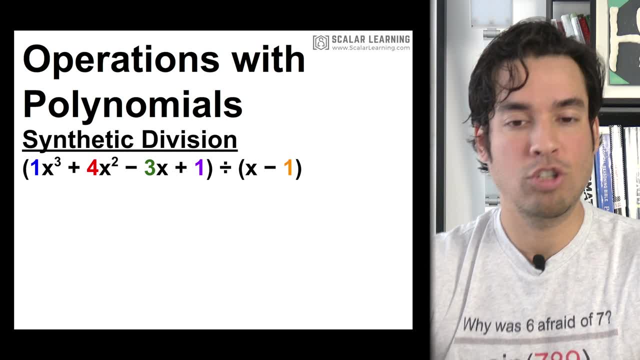 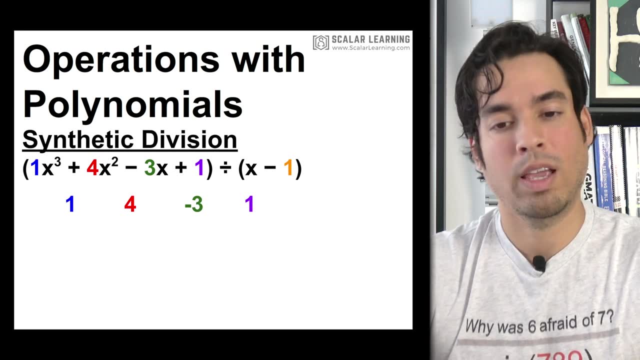 And this is where we're dividing polynomials. I've got this polynomial here: x cubed plus 4x squared minus 3x plus 1 divided by x minus 1.. So here's a little refresh on synthetic division. What you do is we drop all the coefficients from that original polynomial. Okay, I got a 1,. 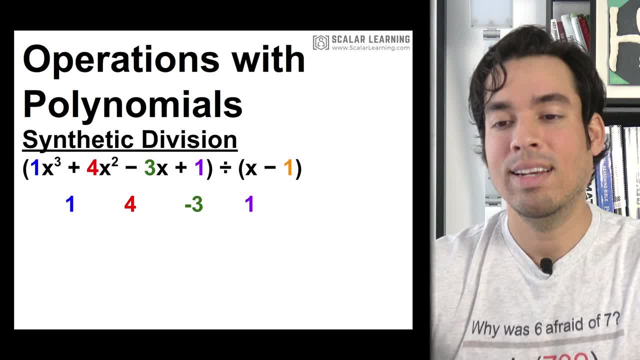 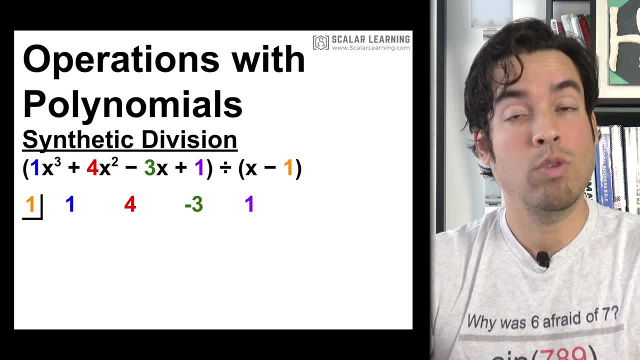 I got a 4,, I got a negative 3, and I got a positive 1.. Boom, Then I take the opposite of that other binomial, that it's dividing by, And this only works, by the way, for dividing by a. 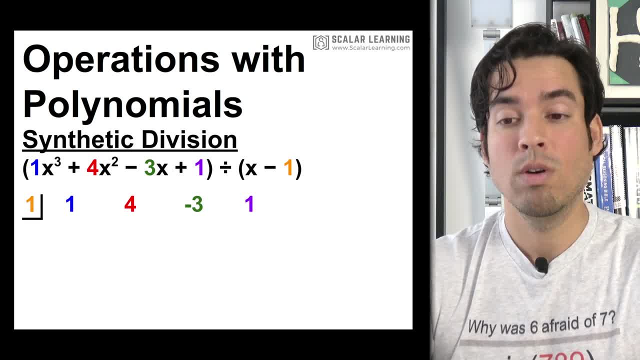 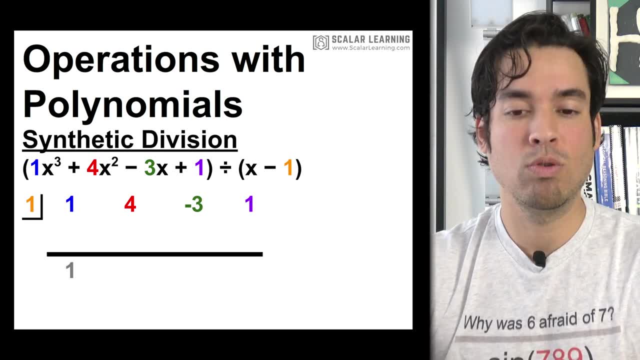 binomial And we've got no coefficient in front of the x, So I'm taking not a negative 1, but a positive 1.. Now here's the process. Throw a line down here. First thing is we just drop the blue 1.. 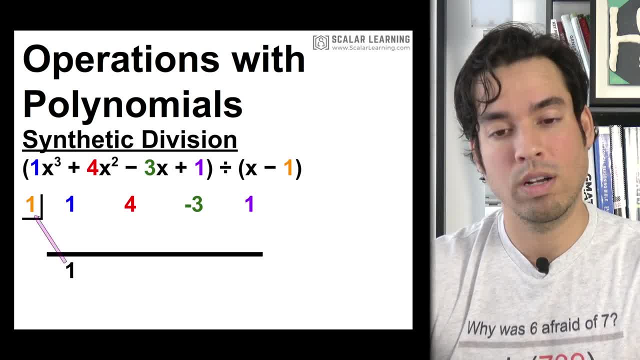 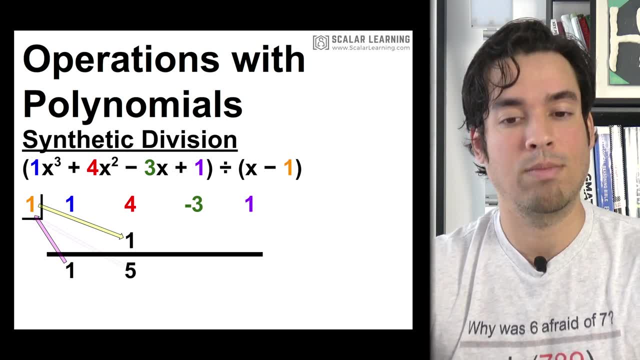 Then we take that and we multiply it against the 1 in the box And then take that product and throw it down here And again we add: 4 plus 1 is 5.. Repeat: 5 times 1 is 5. And we throw the 5 over. 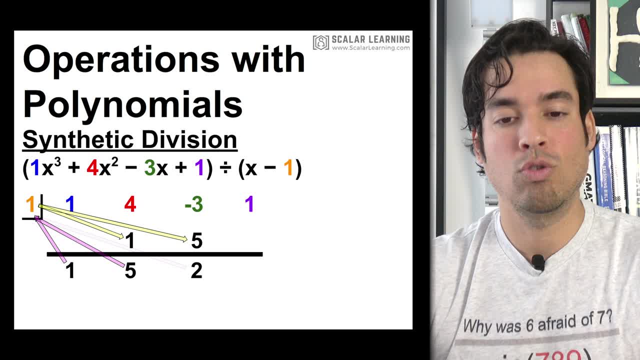 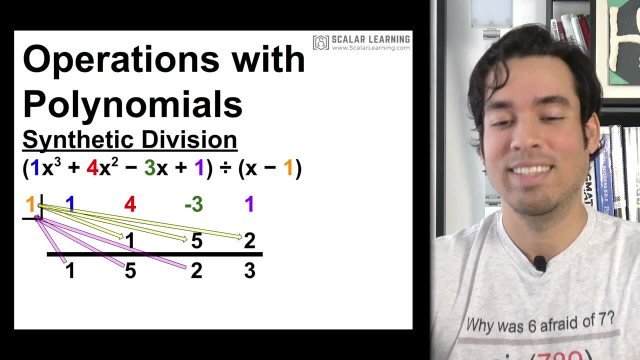 here: 5 plus negative: 3 is 2.. Again, repeat 2 times: 1 is 2.. Throw that over here: 1 plus 2 is 3. And we're done. But what is this? These are just numbers. Okay, this is how it links back. 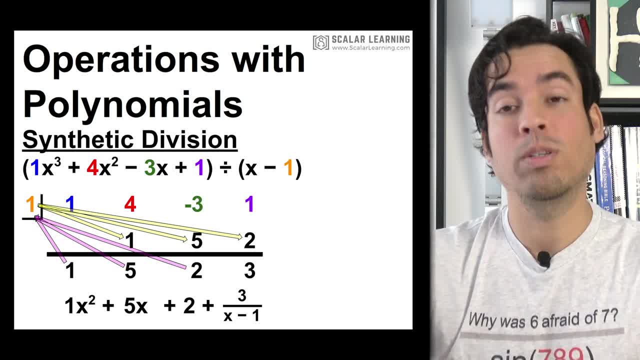 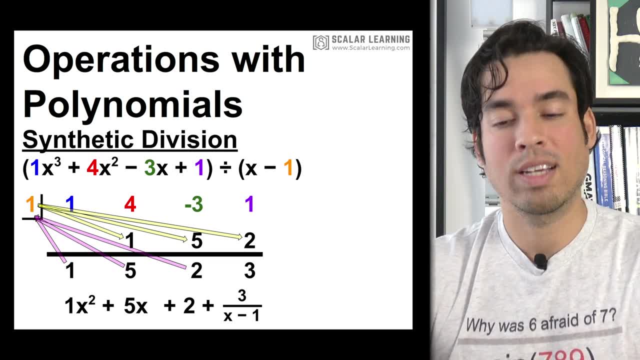 That 1 is the coefficient of notice, an x squared, not x cubed, because we divided right, So the result is going to be a degree lower. The 5 goes with the next one, x 5x. The 2 goes as a. 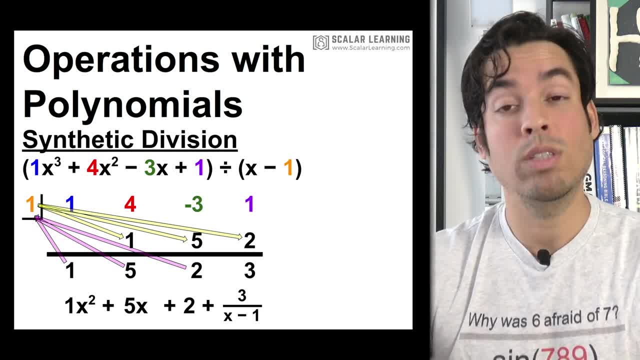 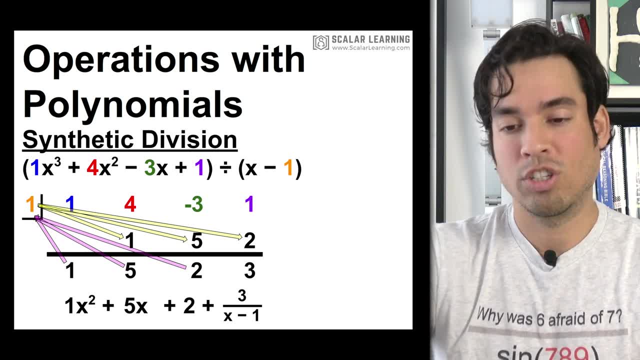 constant, And then we actually have a remainder. Now, if you end with a 0, it means there's no remainder And you're done. But since we do have a remainder, we have to throw it on top of that original divisor, which is x minus 1.. And there you go, By the way, the fact that we have a remainder. 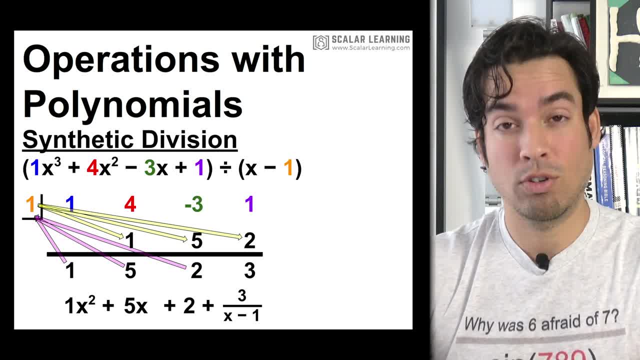 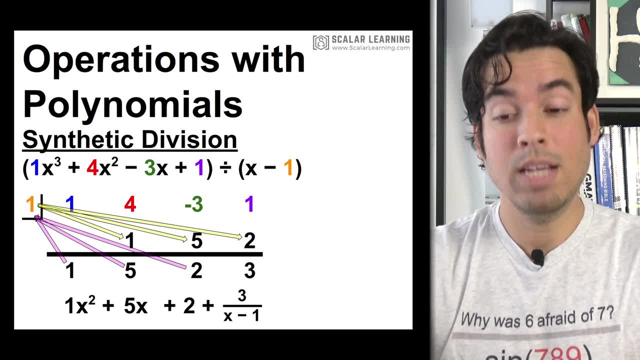 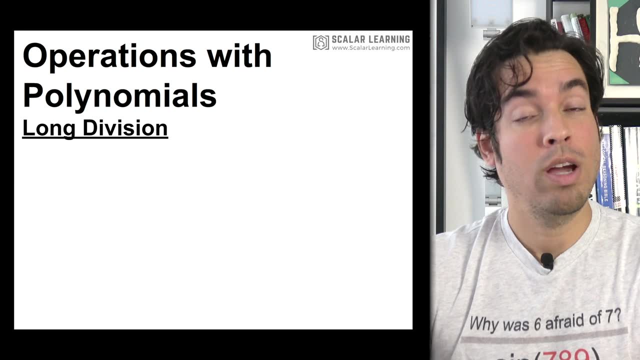 means that 1 is not a factor of this original polynomial, the polynomial on the left, Meaning if I plug 1 in I won't get 0. In fact, the remainder theorem states that if I plug 1 into that polynomial on the left, I will get that remainder of 3.. Now I'm going to show you how. 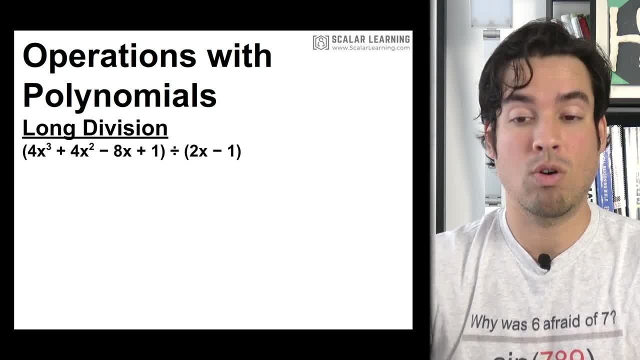 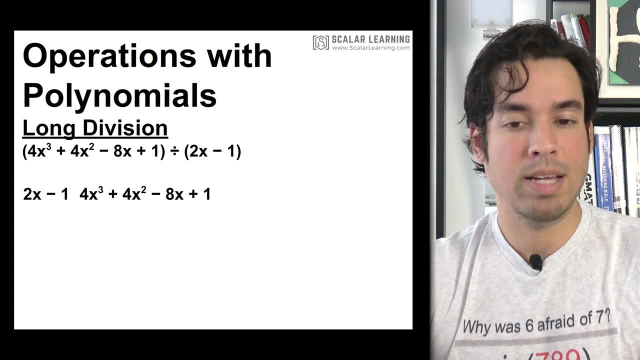 we do long division because long division comes into play When we do have a coefficient in front of that x value. So let me show you how this works. We take the original polynomial, then divide it by that binomial and we have an actual long. 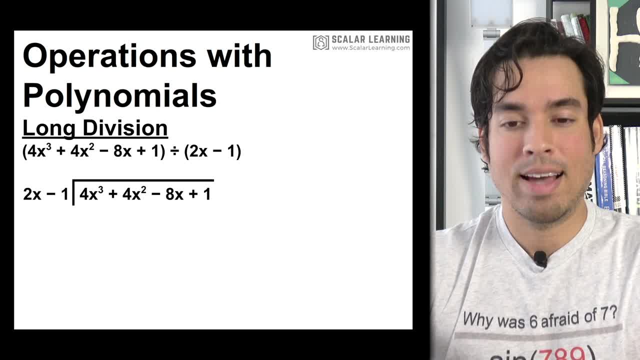 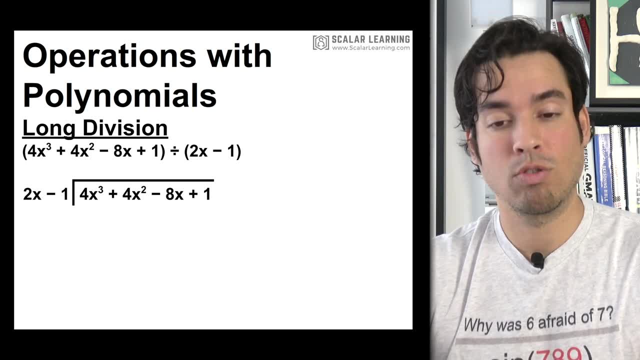 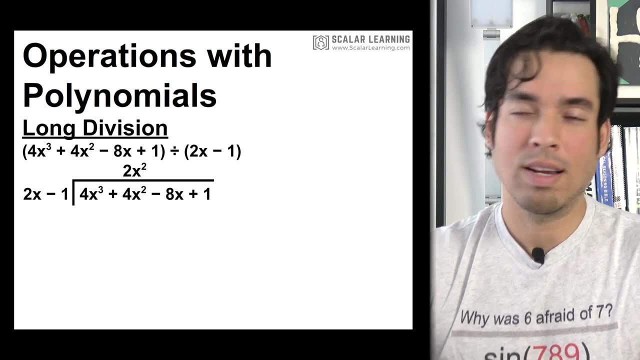 division symbol. Now the first thing that I ask is: I only look at that leading term, the 2x, and the biggest one, starting with the biggest one of the inside polynomial, which is 4x cubed, And I say what times 2x gives me 4x cubed? That would be 2x squared. Then I multiply the 2x squared times. 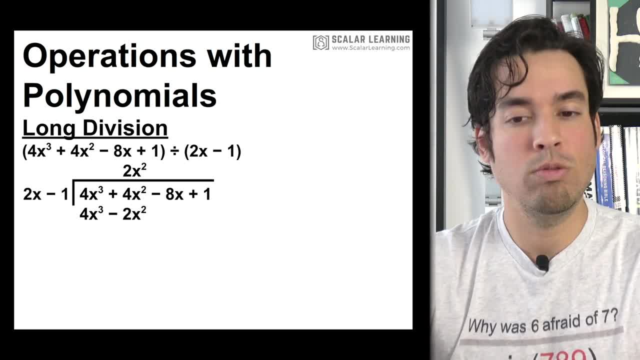 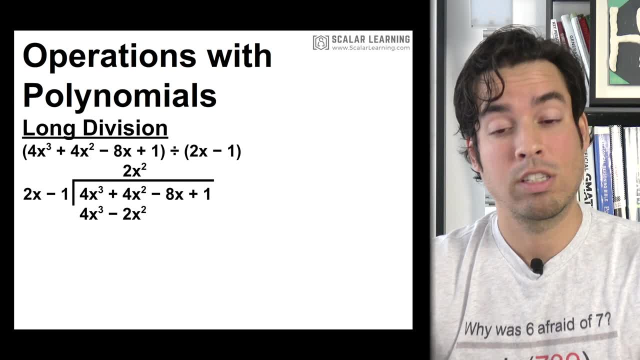 that entire binomial. So I get 4x cubed right. add the exponents minus 2x squared, Because 2x times 2x squared times negative, 1 is negative 2x squared. Now I subtract the bottom numbers. 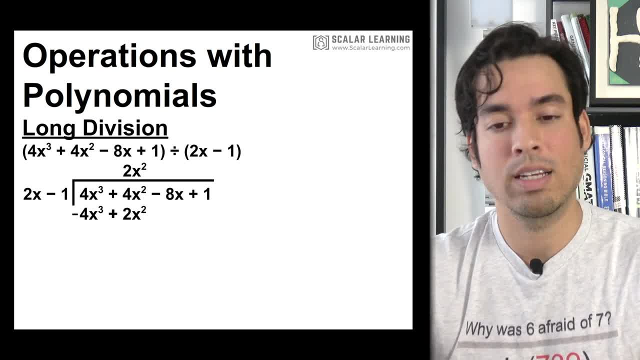 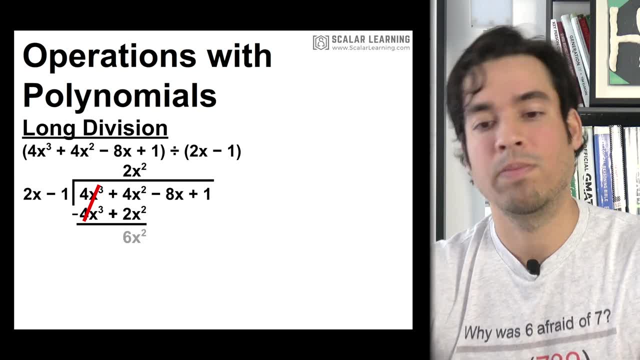 so I do it like this: I negate and negate right, I'm distributing a negative And the negative 4x cubed and the 4x cubed cancels out. That's what I wanted. 4x squared plus 2x squared gives me 6x. 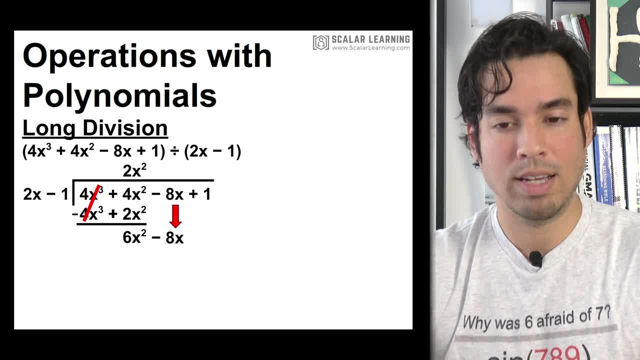 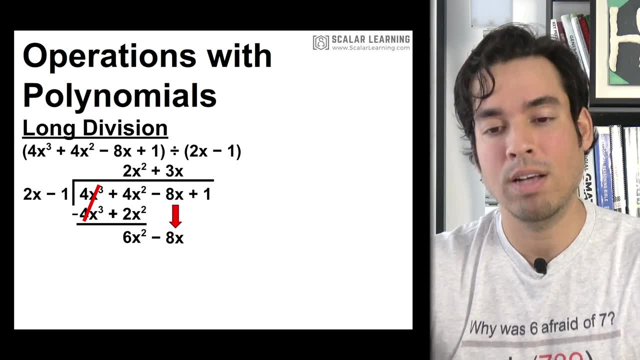 squared. Now, just like in long division, I drop the next term of negative 8x. Now again, x gives me 6 x squared. that would be 3 x positive, 3 x times 2. x is 6 x squared times that negative. 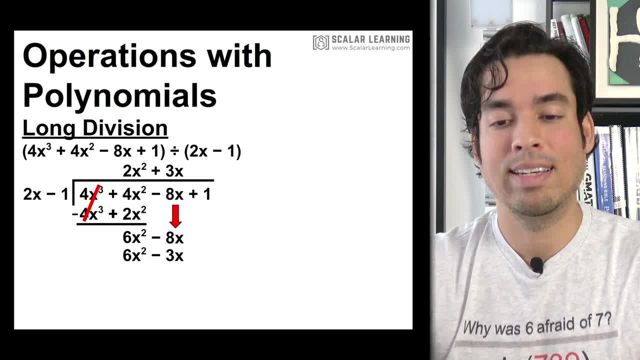 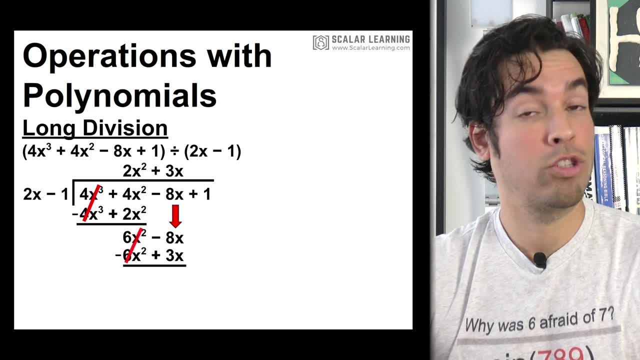 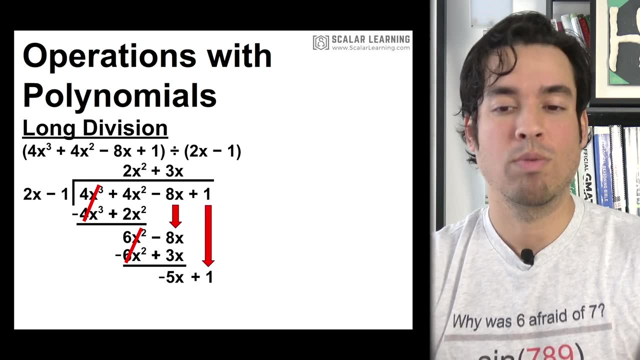 1 is negative, 3 x, again i negate. negate because i'm subtracting: 6 x squared minus 6 x squared gives me nothing, which is what i wanted. and then negative 8 x plus 3 x is negative 5 x- again i drop the 1 and we repeat it one more time. so what times? 2 x gives me negative 5 x. that would be. 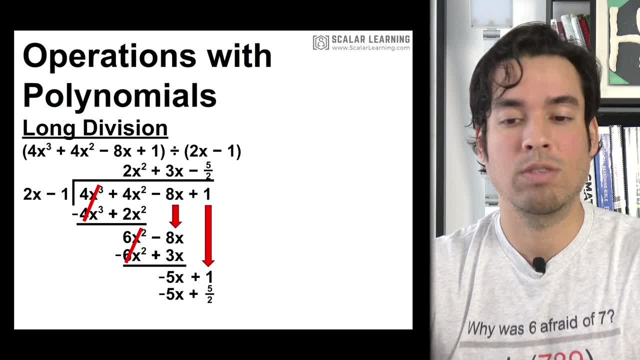 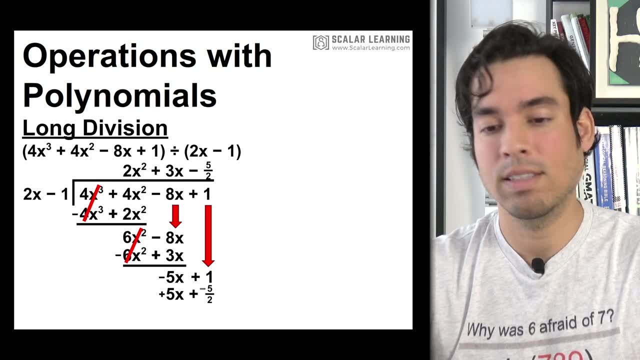 negative 5 over 2. negative 5 over 2 times 2. x gives me negative 5 x and then negative 5 over 2 times negative. 1 gives me positive 5 over 2, negate, negate and again negative 5 x plus 5 x. 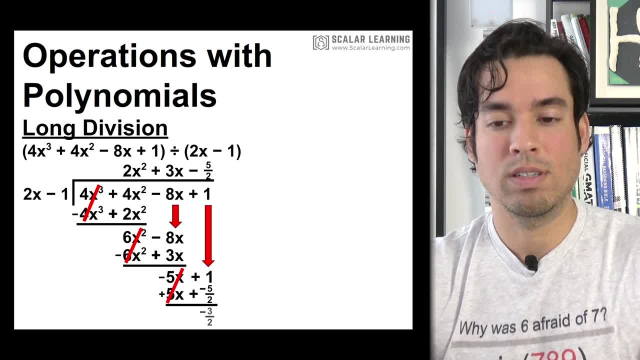 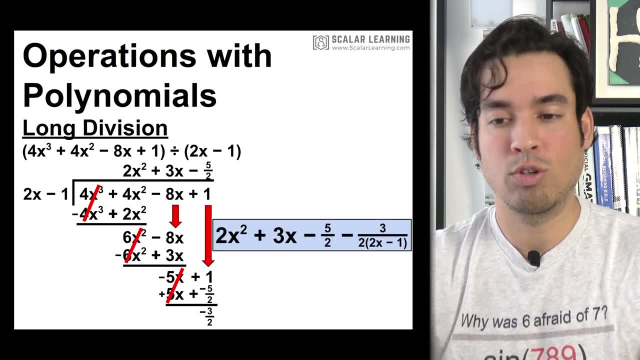 is nothing, and the 1 plus negative 5 over 2 is negative 3 over 2. so again i have a remainder of negative 3 over 2 and the final polynomial looks like what i got on the top: 2 x squared plus 3 x minus 5 halves and then minus 3 over 2 over that original. 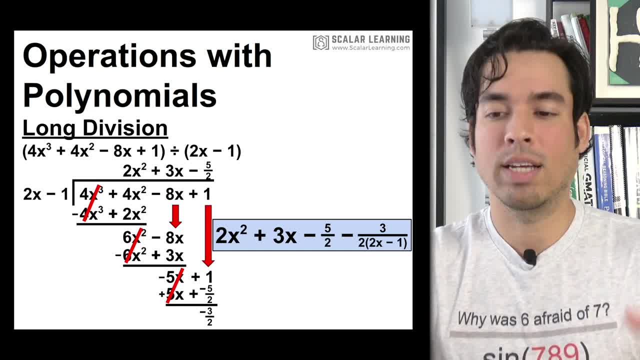 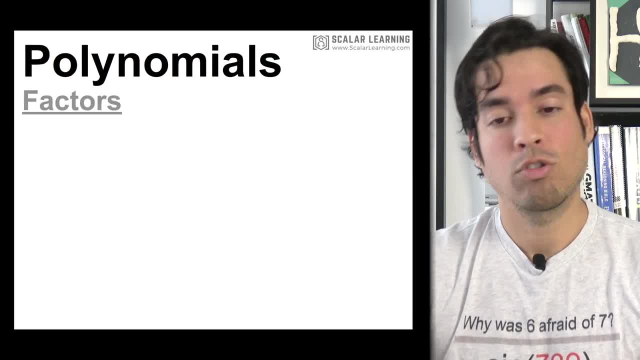 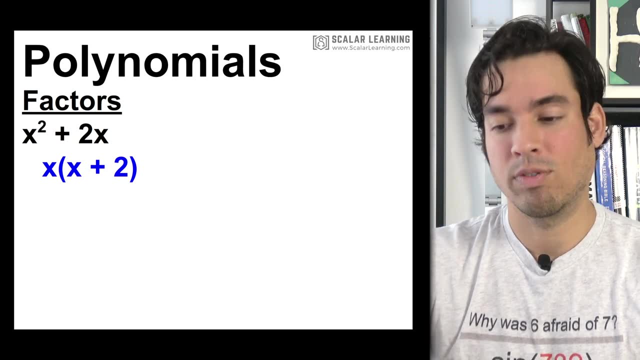 divisor, but again it's a fraction. you're dividing so that it becomes 3 over 2 times 2 x minus 1. now we're going to talk about factors of polynomials. so just some simple examples. we got x squared plus 2 x. here we can factor out in x and we've got two factors. we've got x and we've 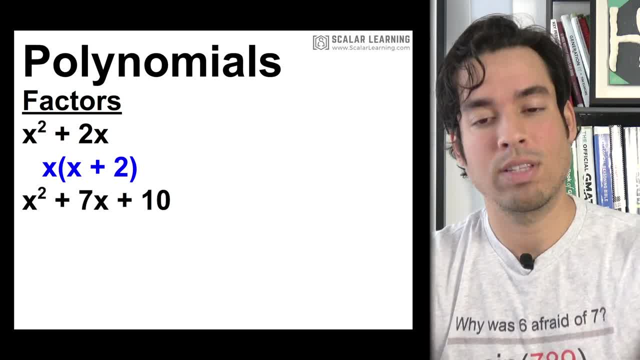 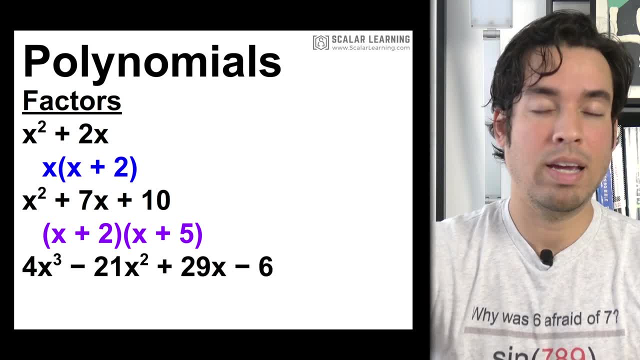 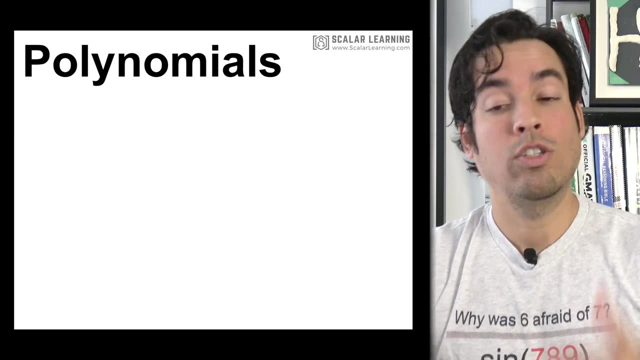 got x plus 2, then in this one we notice we again follow that same protocol. what multiplies to 10 and adds to 7, that's positive 2 and positive 5, and with a more complicated one, this one factors out to 4 x minus 1 times x minus 2, times x minus 3. so what do these factors mean? 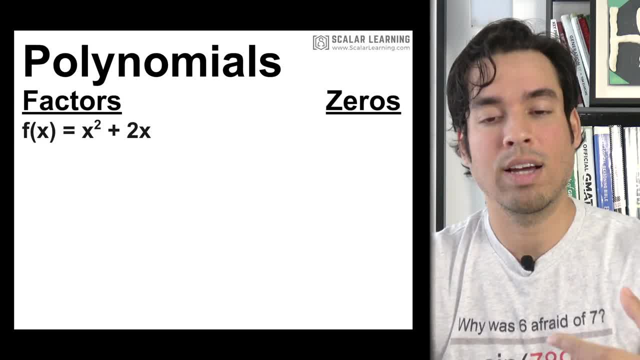 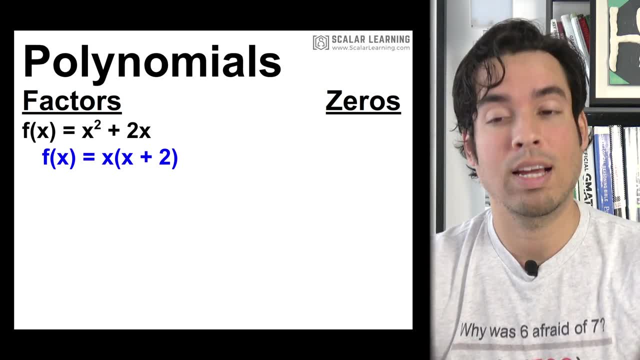 in terms of zeros. so let's go through the list again. so we've got this one that factors to, and now look, i'm expressing it as a function. i've got a function of x times x plus 2. it means that i have two zeros at zero, because when i plug zero in for x on the left, 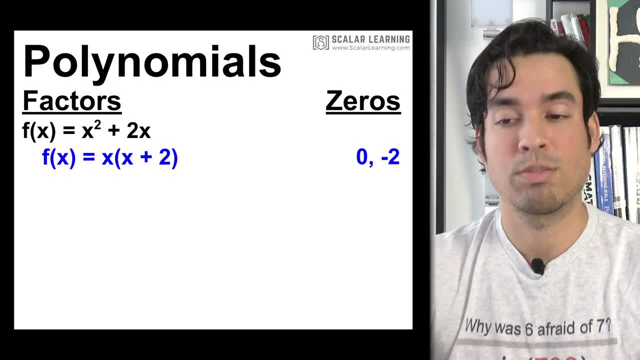 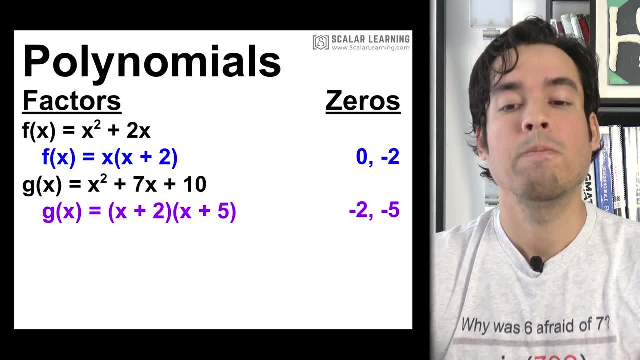 zeros everything out. by plugging negative 2 into that binomial x plus 2, i get a zero. when this guy is factored again, i have zeros at negative 2 and negative 5 and last but not least, with the big dog, if i factor that one i've got three zeros right, because the fact goes into: 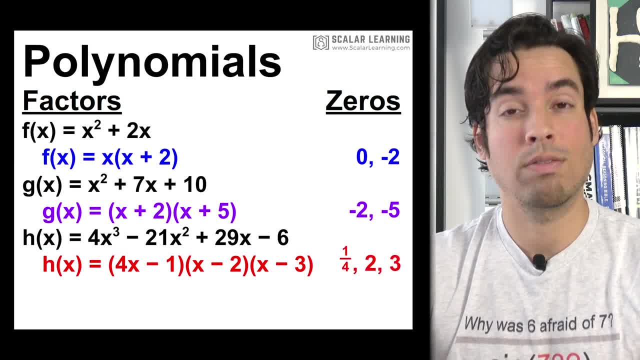 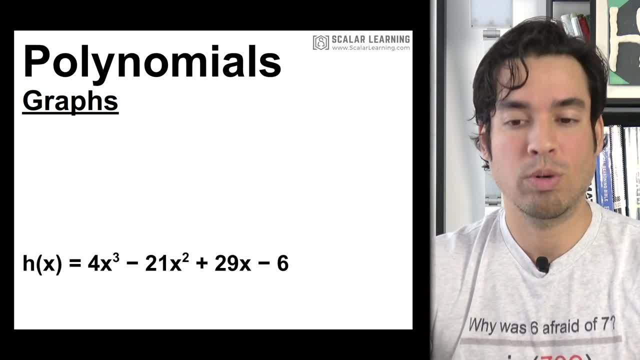 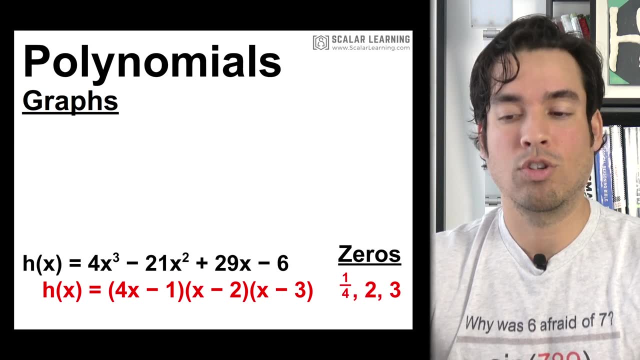 three factors: positive 1, fourth, positive 2 and positive 3. now let's talk about the graphs of these polynomials, especially that more complex one that we saw at the end: 4 x cubed minus 21 x. so when we factor it and we know that the zeros occur at one, fourth, two and three, what does that? 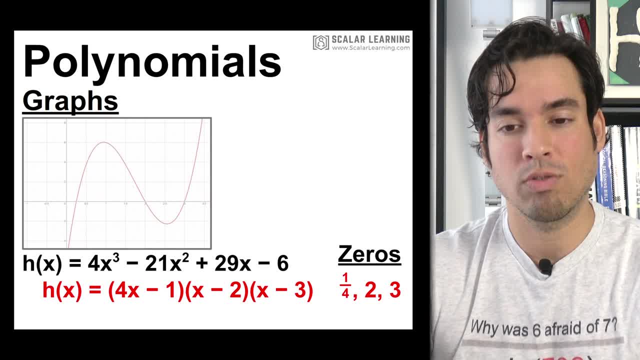 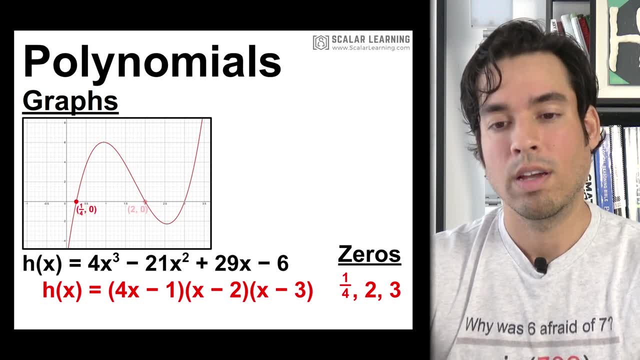 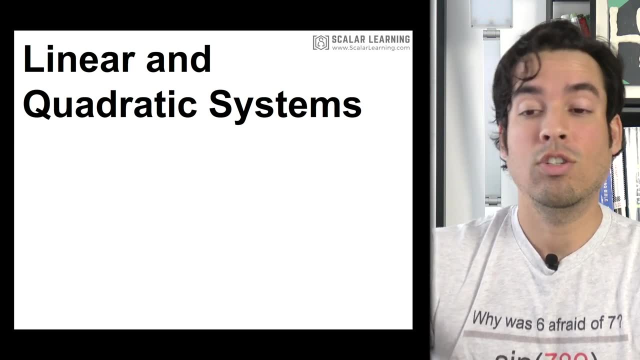 look like on the graph. again, the zeros are the x intercept. so if i look at this function, you notice that i've got a zero, aka an x intercept, at one fourth zero, at two zero and at three zero. next let's talk about linear and quadratic systems. okay, these are systems of 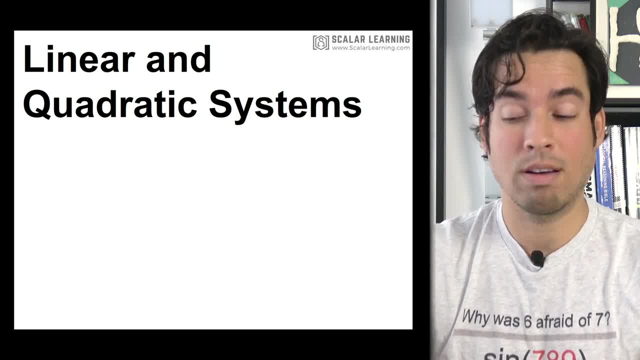 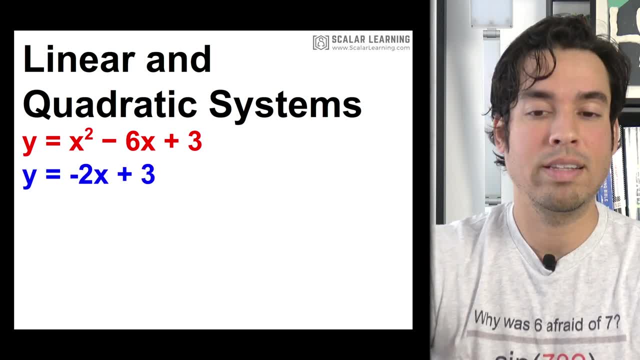 equations. anytime you're thinking about systems, you're thinking about points of intersection. so y equals x squared minus 6x plus 3, and then which is the quadratic? and then we got a linear of negative 2x plus 3. if we look at those two on a graph, one's a line, one's a parabola, and we're 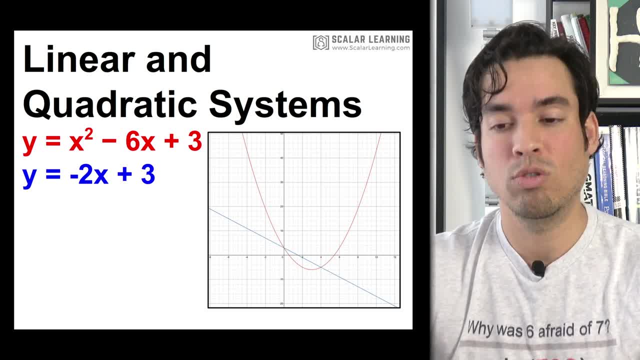 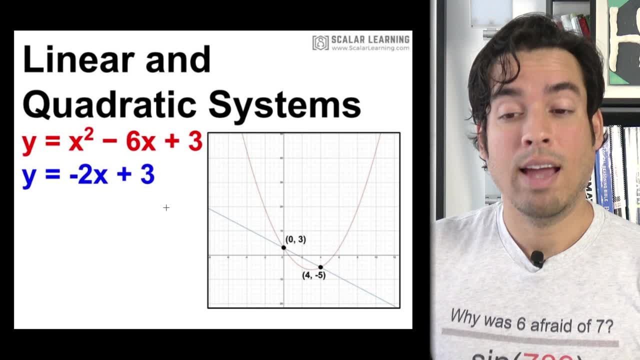 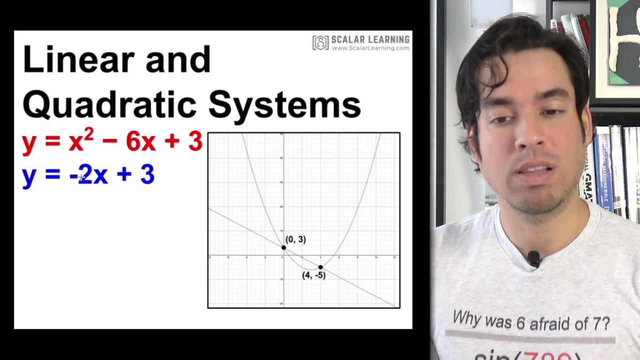 looking for the intersection points. those are the solutions. so the two solutions are 0, 3 and 4, negative 5. now, if i didn't have a graph like this to show me the intersection points, there's another way that i can solve this: just by simple substitution and isolation, so i can plug in. 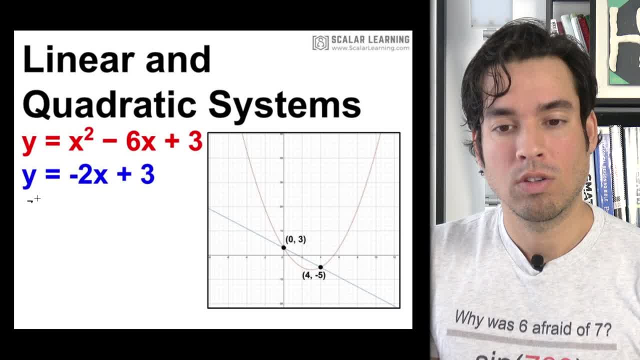 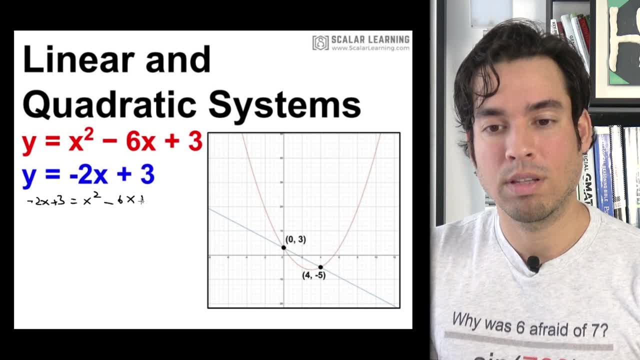 negative 2x plus 3 for the y up top. so let me show you how that looks. so i have negative 2x plus 3 equals x squared minus 6x plus 3.. now i want to isolate, so i'm going to add 2x to both sides because, again, we always want to. 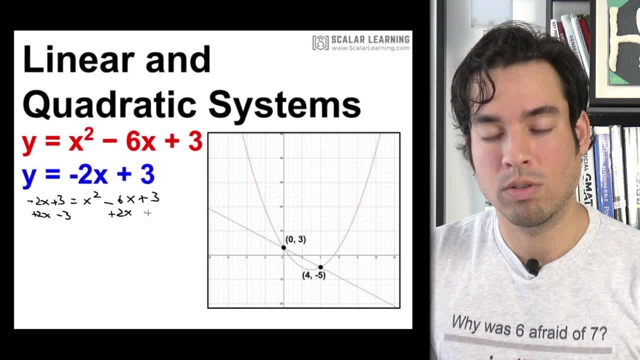 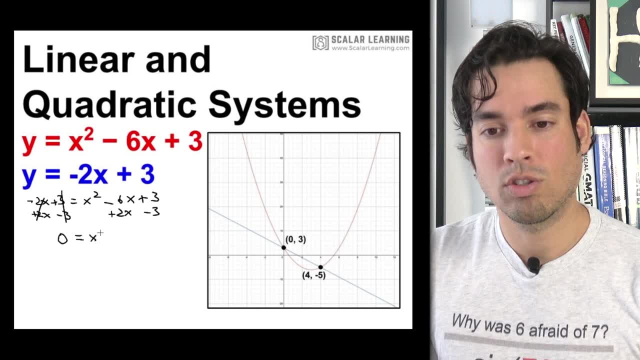 set everything equal to 0 and i want to subtract 3 from both sides. okay, that cancels, that cancels. now i have 0, which is exactly what i want. equals x squared minus 6x negative. 6x plus 2x is negative. 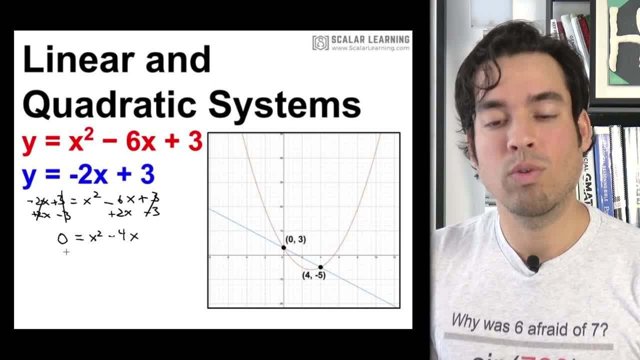 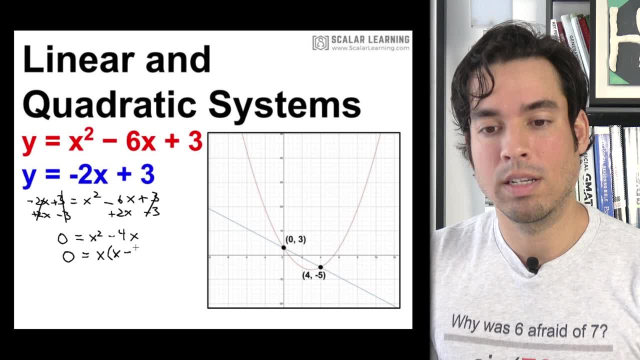 4x. these guys cancel out again. now we're going to factor. so again, here's just a simple factoring. i can factor out an x, i get x minus 4. so again, if i distributed that, i get x squared minus 4x, which is what we. 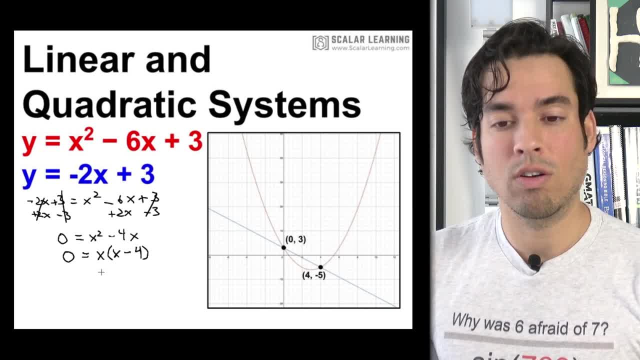 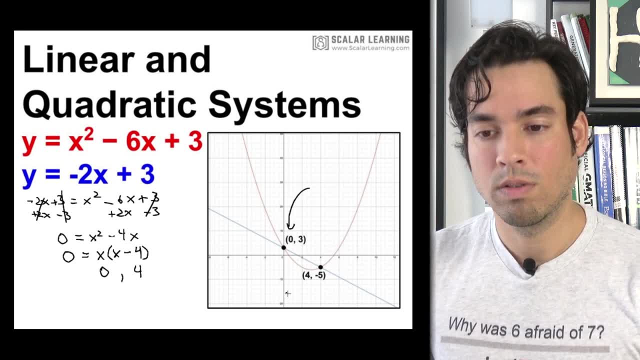 want? and what are my two zero values? what zeroes this out? it would be 0 and 4, and if you notice on the graph, there's the 0 and there's the 4. now if i, if i wanted to get the corresponding y values, i 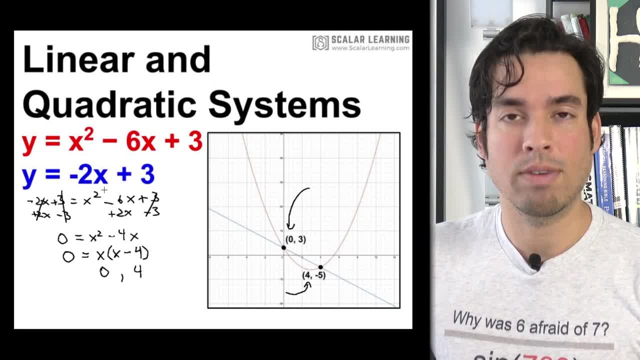 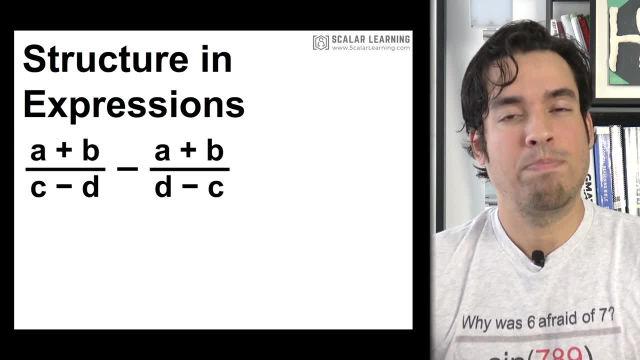 would get the corresponding y values into either of these equations and i'll get the right, the right y value. next we have structure and expressions, another subcategory. what we're doing here is we're basically just combining these two rational expressions and the way we want to think about it. 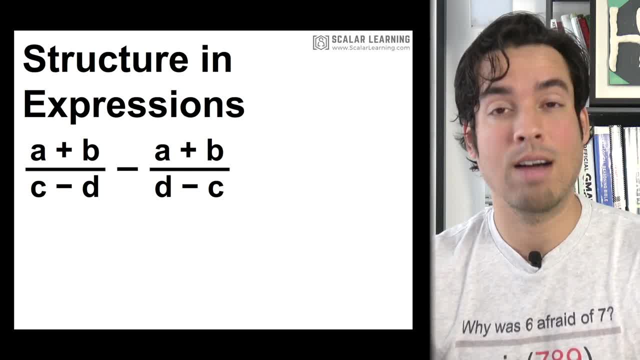 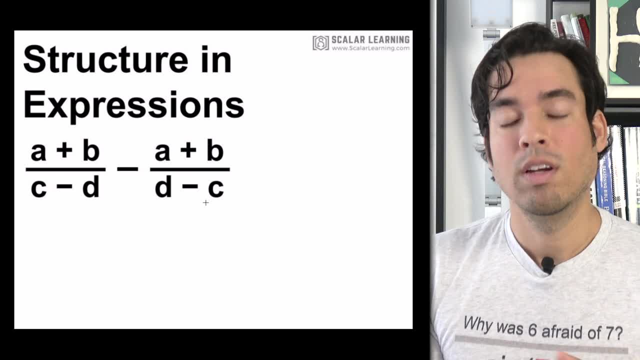 is the same sense that we think about combining fractions, getting common denominators. so let me show you how this works. so the thing is, i look at this and it almost looks like they have the same denominator, except for this is flipped. so i, i can, i can, real easily. 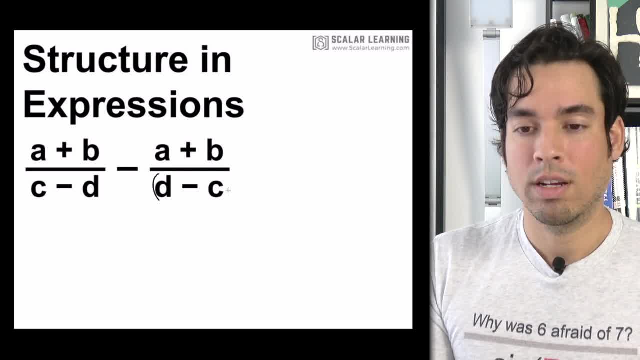 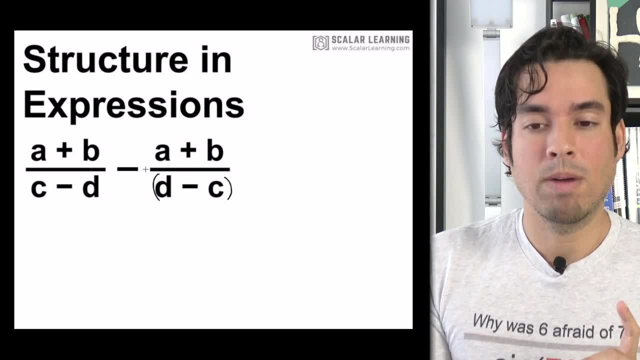 factor out a negative one out of this expression and flip it to c minus d. okay, by the way, if i factor out a negative one, it's going to come up top and make this whole expression negative, but it's going to nicely cancel out with that negative in here, that minus in here. so watch what's going. 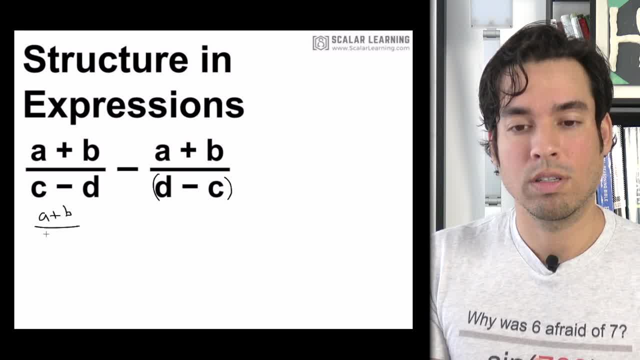 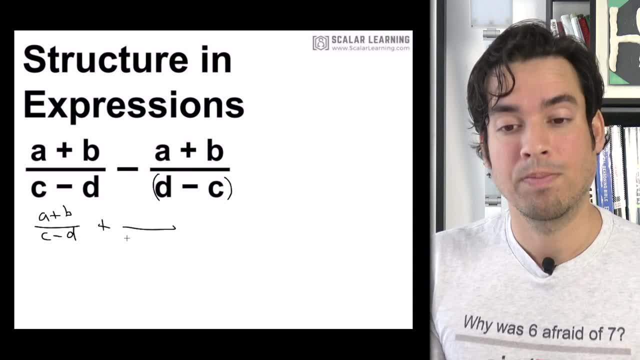 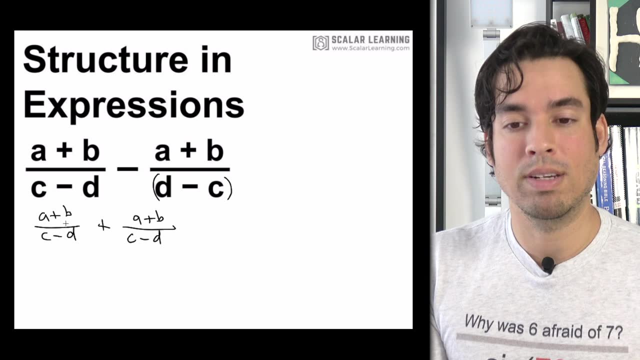 to happen. it's going to be a plus b over c minus d. that's fine plus, because again i factored out negative, which flips this into c minus d, and then it cancels out with that minus and then i got a plus b on top. now what's going to happen now? 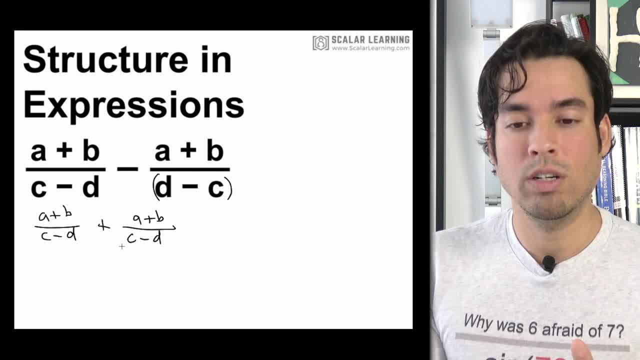 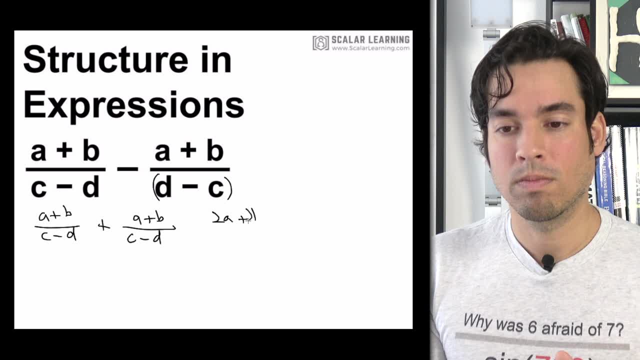 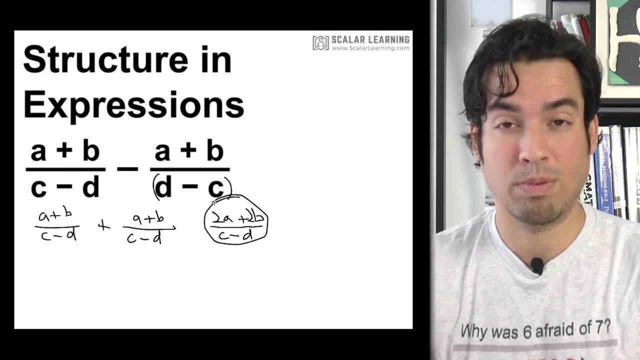 i've got common denominators. very straightforward, just add the numerators. so if i add a and a, i get 2a. add b and b, i get 2b over c minus d. and that's it. that's our fully simplified expression. and next here's another. 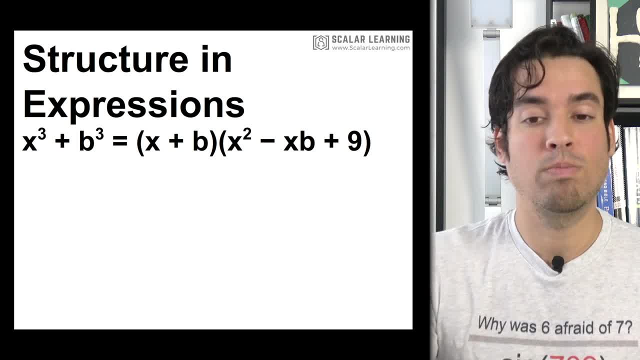 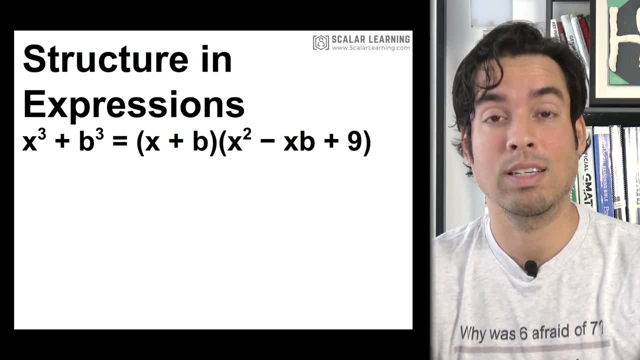 example of a problem where we see on the left it's x cubed plus b cubed equals this whole craziness right a binomial times a trinomial. so how do you approach something like this? well, you start by recognizing that the two sides are equivalent. and again, my advice is always: if you see something, 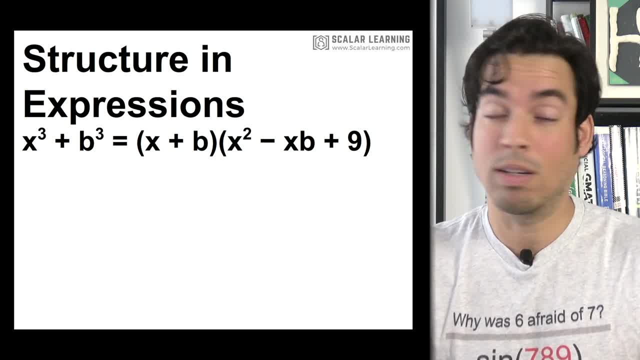 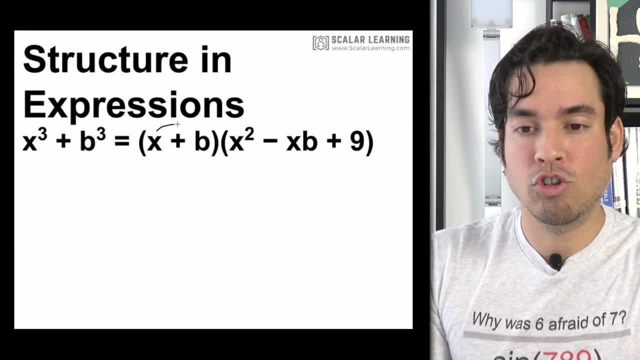 in its normal form and it's a quadratic or higher factor, it. if you don't know what to do here, it's already factored. well, what should you do? the opposite of that, which is foiling. so let me show you. so first, i'm going to start by distributing boom, boom and boom. so i got x cubed minus. 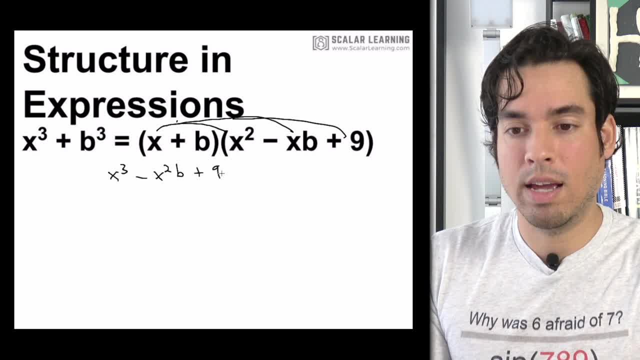 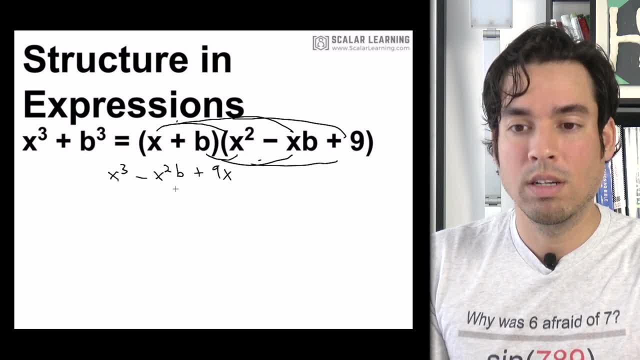 x squared b plus nine x. now i'm going to start with this guy. now notice how i'm going to just kind of lay it out a little bit differently, and you'll see why in a second. so i'm gonna do b times x squared, or let's call it x squared b, and then i got negative b squared x and 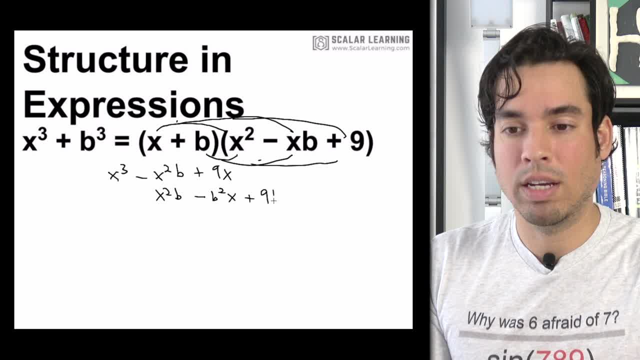 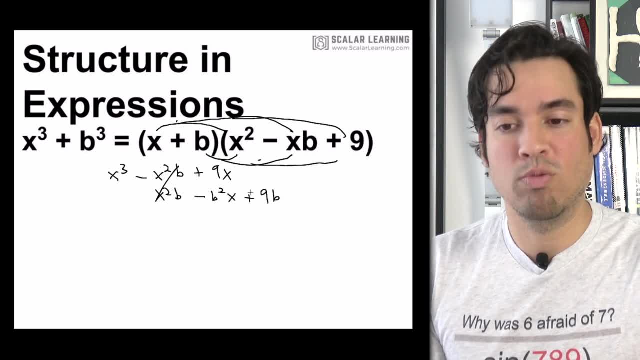 then, last but not least, i got 9 times b. okay, the reason why i did it like this: first of all, these cancel out, which is great, these kind of combine, because they're both x terms or they they can be grouped together. and then i got 9b at the end. so i've got now on the 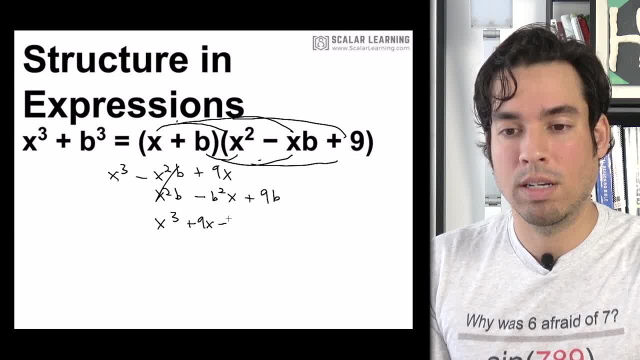 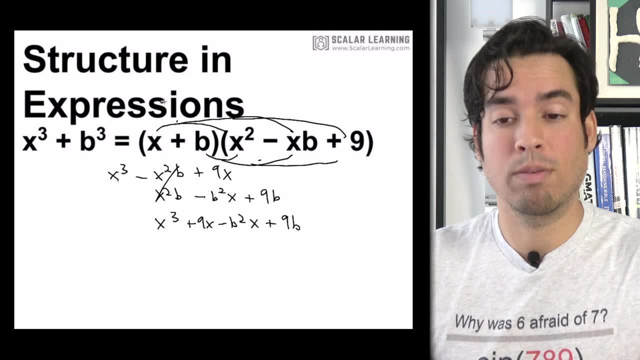 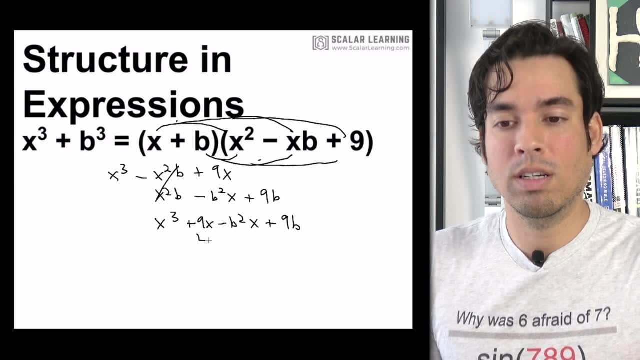 x cubed plus 9x minus b. squared x plus 9b. So there's two things that are important to note if I'm trying to figure out what the value of b is. Number one: there's no x term on this side, which means that these guys are probably going to zero out. The second thing is that 9b equals b. 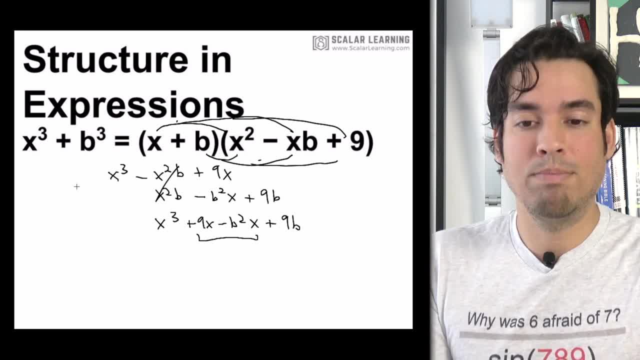 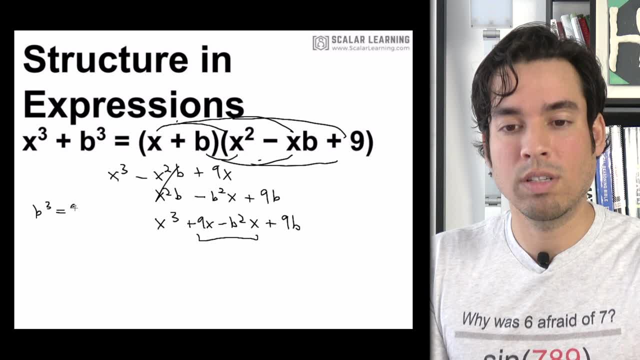 cubed. I can use either of these to solve for b. Let's use the 9b equals b cubed. so because 9b is the constant here and b cubed there, So if b cubed equals 9b, I can divide both sides by b. 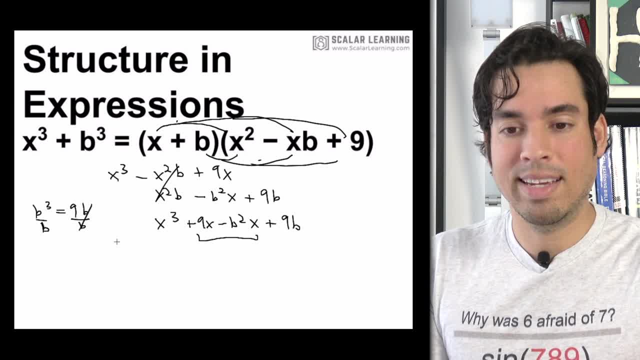 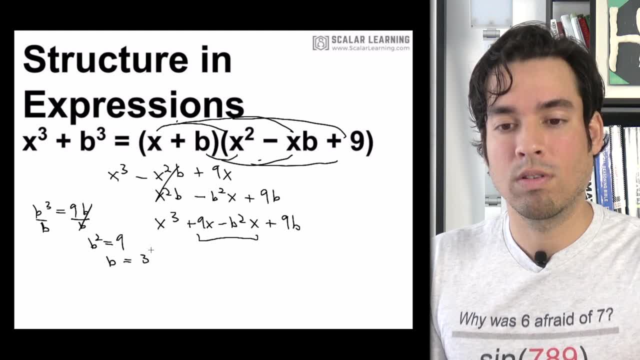 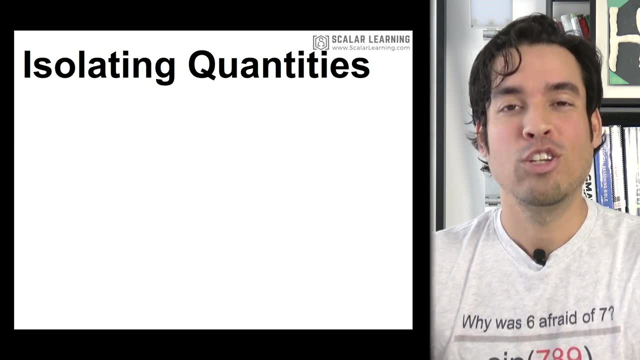 and I get 9 equals b squared, which means that b is going to give me a value of 3.. Next we come to one of my favorite categories, which is isolating quantities. and why do I love this so much is because usually isolating quantities questions have all this dense. 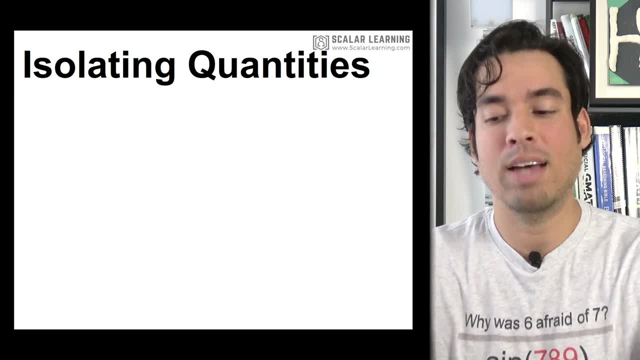 verbiage and they go through this in these complex ways. So I'm going to show you how to do that. So I'm going to show you how to do that. They're really meaningless because you look at the answer choices and you're like: oh they're. 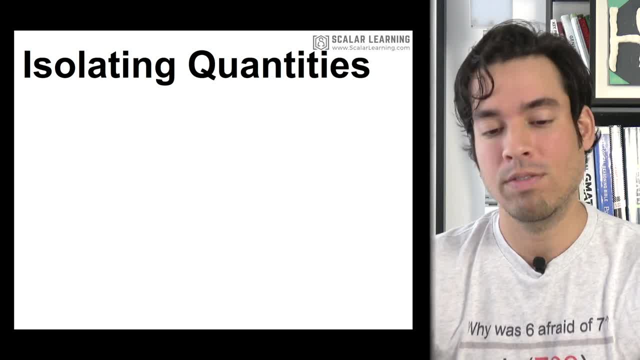 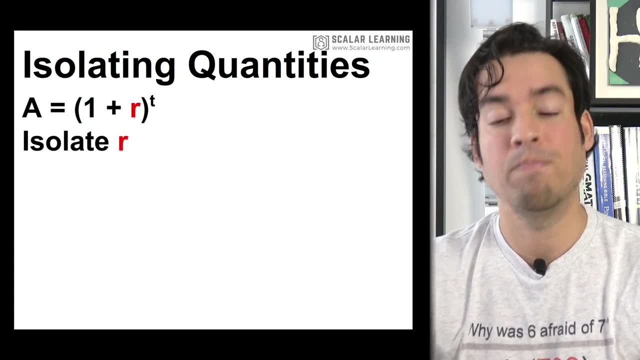 just isolating one variable in this equation. So I'm going to give you this example of a equals 1 plus r to the t power, and we are trying to isolate r. that's why I put it in red. So let's go through the process. So all we're going to do is we're going to first get rid of this t. Well, 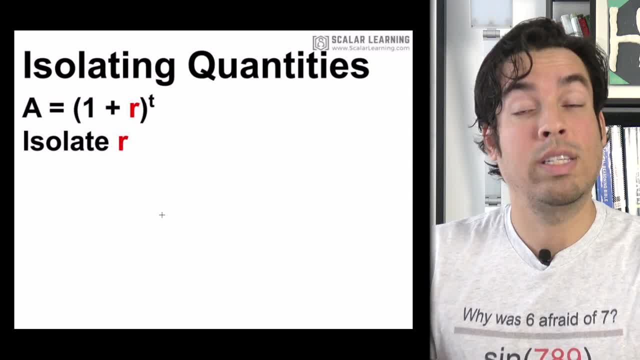 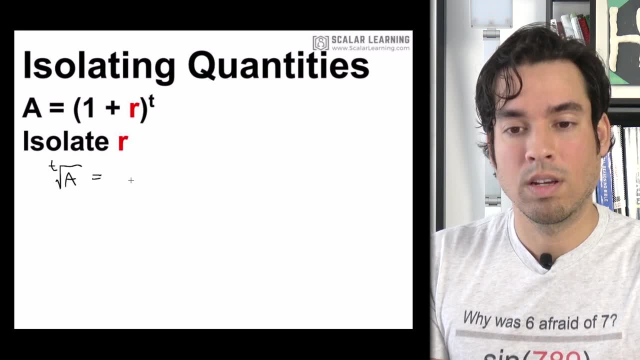 first of all, how do I do that? It's to the t power. So what's the opposite of taking something to the t power, Taking the t root? So, for example, I'm going to take the t root of a and the t root of 1 plus r to the t power. These cancel out. Now I have the t root of a. 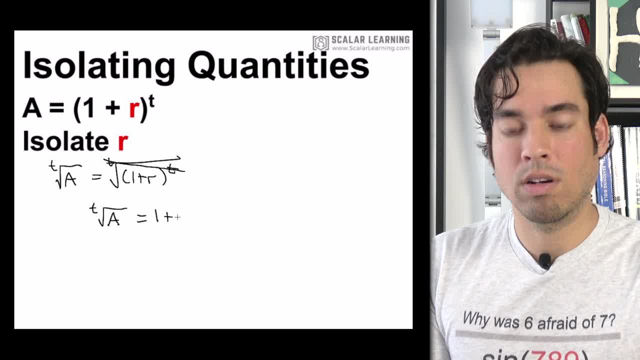 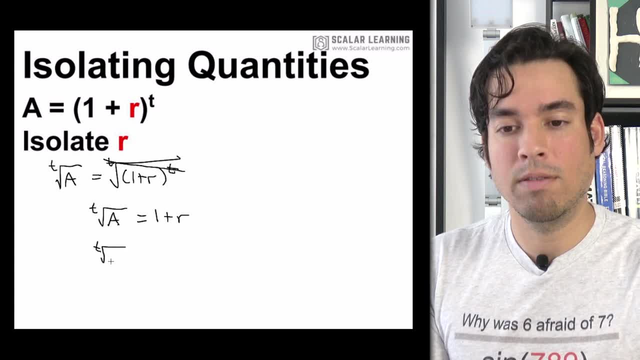 equals 1 plus r. Last but not least, I need to get rid of that 1.. So I'm going to subtract 1 from both sides. We could say the t root of a minus 1 equals r and we have successfully isolated r. 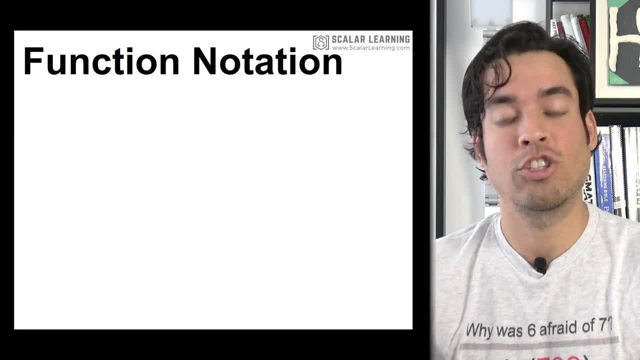 Finally, we come to the t root of a. So I'm going to take the t root of a and the t root of a equals 1 plus r. Next we need to do the function notation. So function notation is just simply knowing function notation, understanding how to apply it. So I'm going to give you a couple examples of a function. 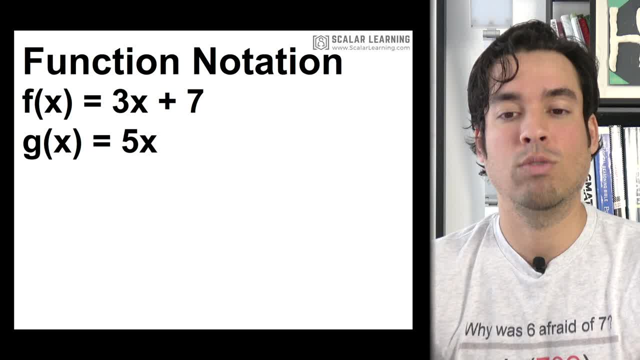 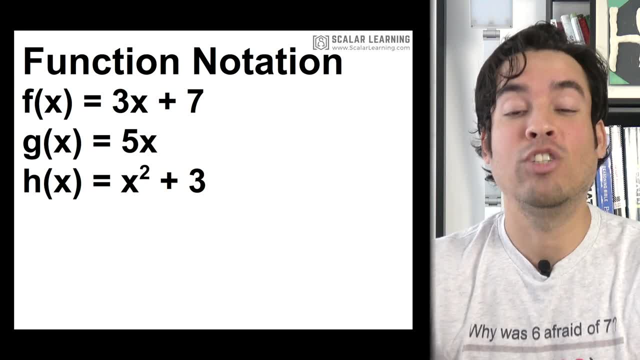 So, for example, we have f of x equals 3x plus 7, g of x equals 5x and h of x equals x squared plus 3.. What the heck are these f of x, g of x and h of x things? It just means function f, function g and 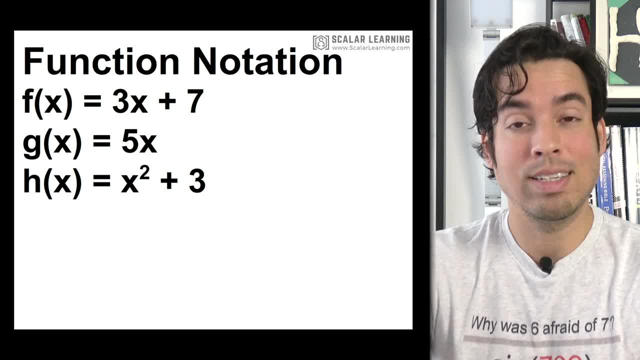 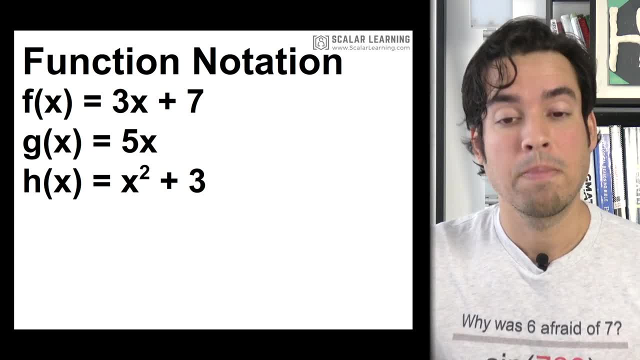 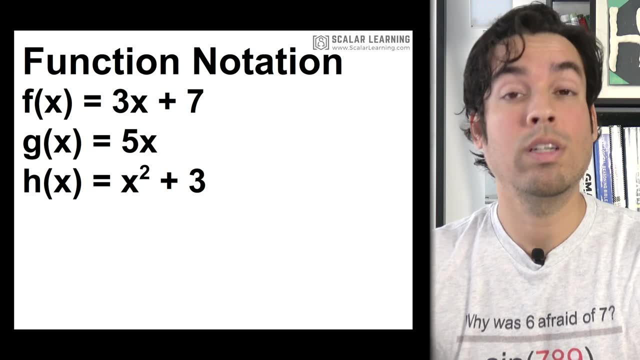 function h and the reason why the parentheses and the x. it doesn't mean it's f times x, It means variable of x. You can literally substitute y in The function value is the same as the y value. That's it. Now we're going to go through some other examples where what if they ask: hey? 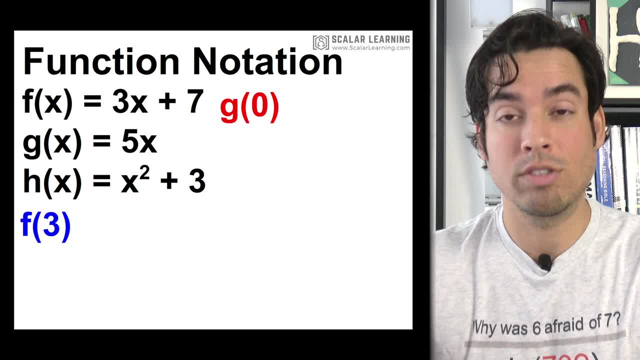 there's f of x. We want to know what's f of 3.. We want to know what's g of 0, and we want to know what's h of negative 2.. This is where understanding the notation comes into play. So if I want f of 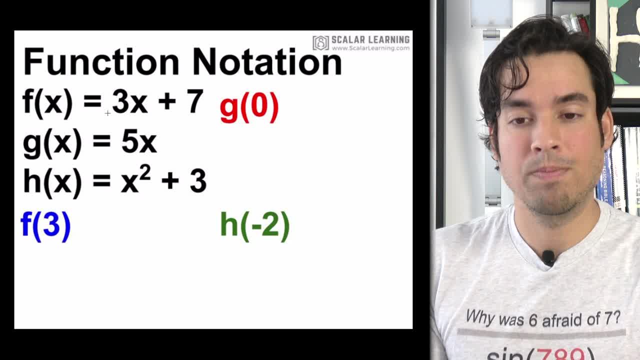 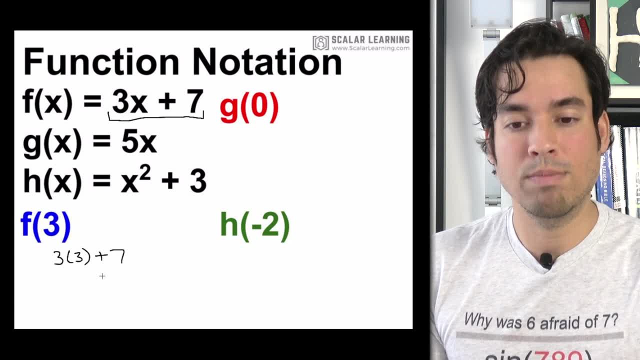 3,. they literally mean to replace the x with 3 in this function. So it becomes 3 times 3 plus 7, which is simply 9 plus 7, or 16.. Same with this one. I want to plug 0 in for x here. 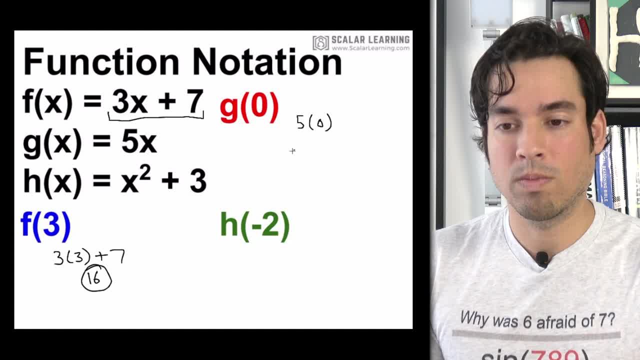 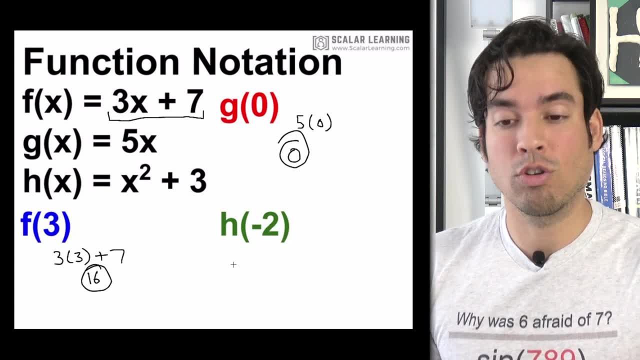 So it's simply 5 times 0, which is 0.. Last but not least, I want to plug in negative 2 into my x for h, So it becomes negative 2 squared. Don't forget, the whole thing is squared plus 3.. 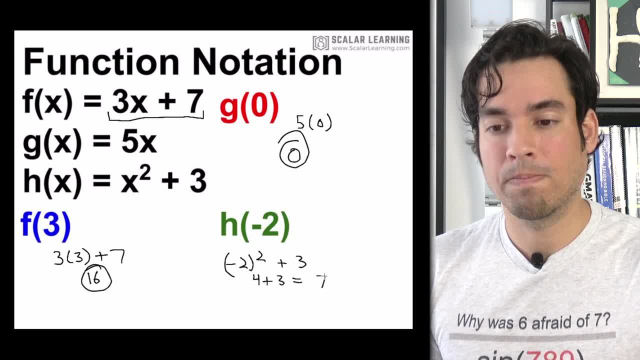 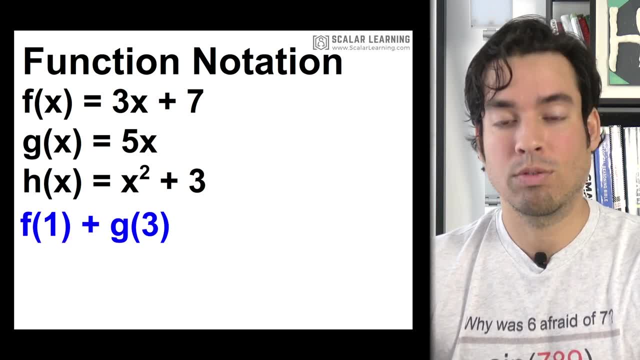 That's 4 plus 3, which equals 7.. Another example involving all three of these original functions: it would be f of 1 plus g of 3, addition g times h of negative 1.. What the heck is that We're going to talk about that in? 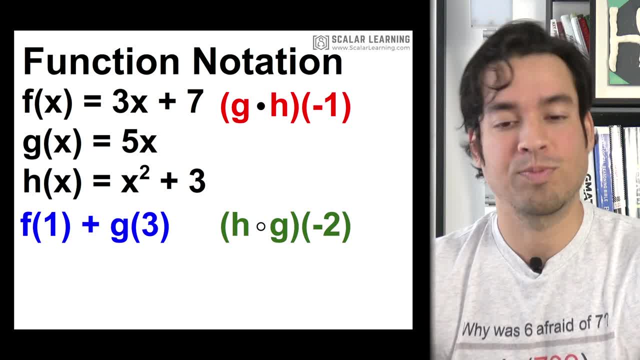 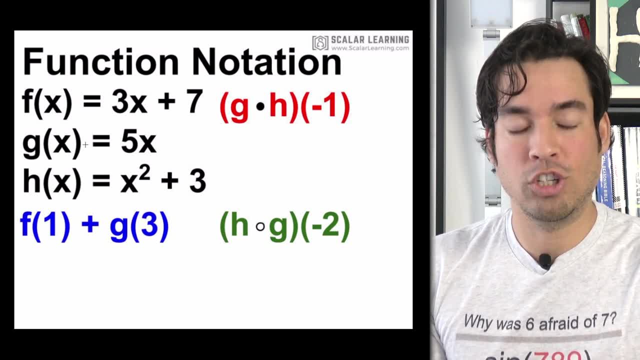 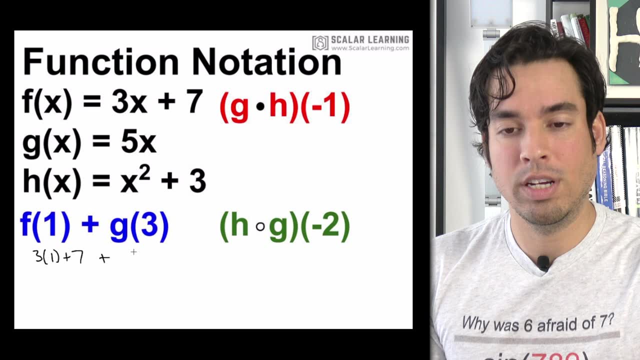 a second And then this interesting open circle. So let's go through all these examples. The first one is pretty straightforward: We're simply plugging in 1 for f of x and 3 for g and adding them together, So it'd be 3 times 1 plus 7, that's my f of x plus g of 3.. 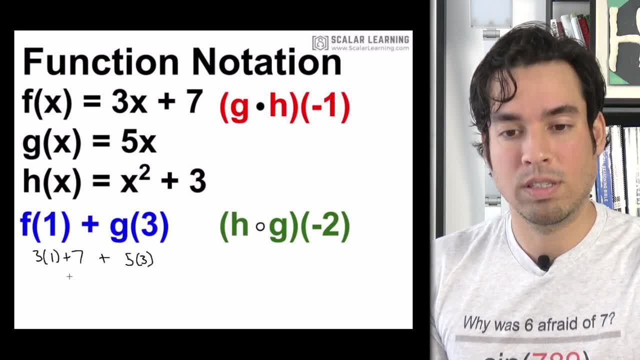 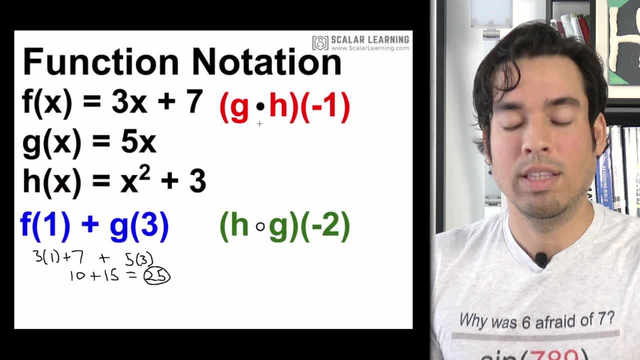 Which is 5 times 3. This becomes 3 plus 7, is 10.. Plus 15 gives me a nice 25.. In this example they're saying g times h of negative 1. So there's two ways we can think about.